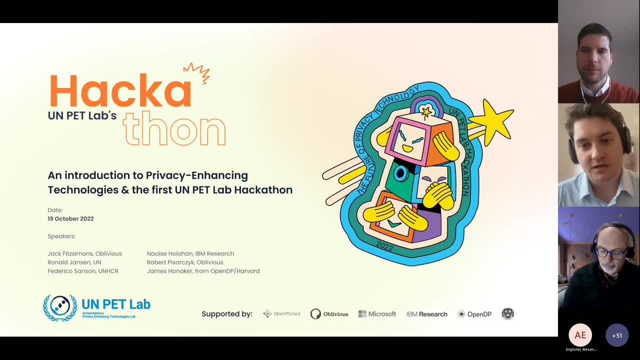 of the pets landscape And finally, one of the important topics- that's a major topic that we're going to be talking about- is the future of the competition and is also around differential privacy, and we want to have a bit of an understanding from that And fortunately we have James Honaker, who's the Chief Privacy Officer. 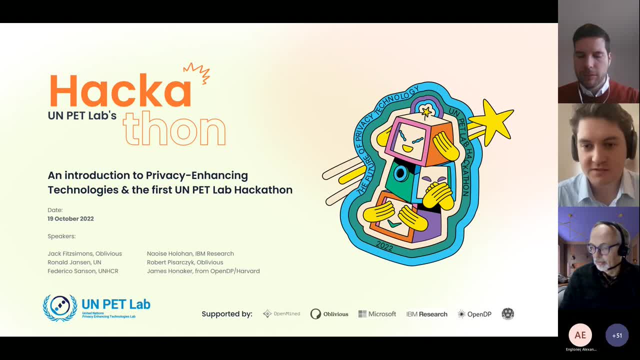 of OpenDP and has worked in the space of privacy, really been a pioneer of that over the last decades. So it should be a good lineup and at the end of it all, hopefully the competition itself will seem to make a bit more sense. and then the webinar. 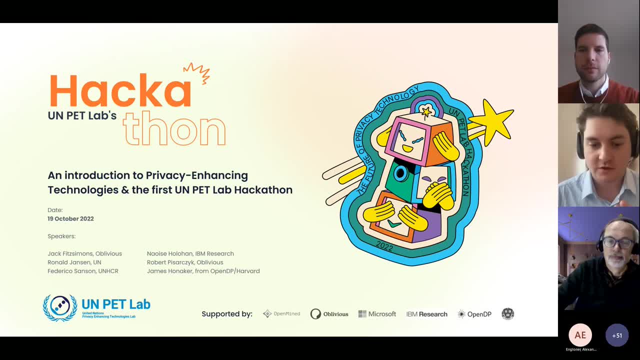 this day, same time next week will actually go over the libraries, the scoring, the mechanics of the competition itself. so you know how to be engaged throughout the competition that's running, once again, from the 8th to the 11th of November. So from there I'll leave it to you, Ronald, to take over. 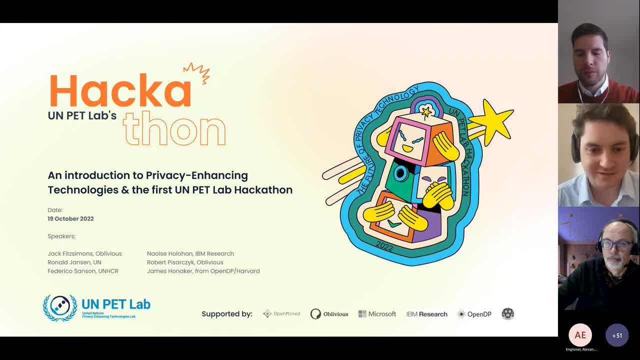 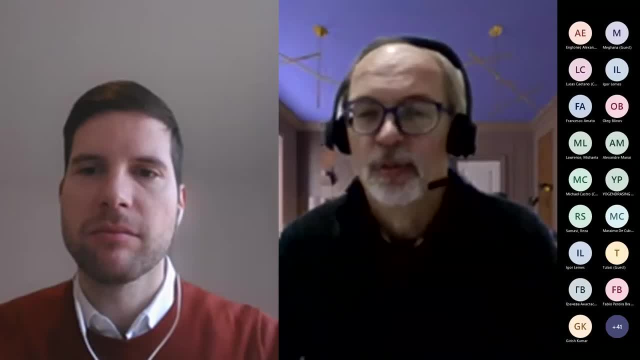 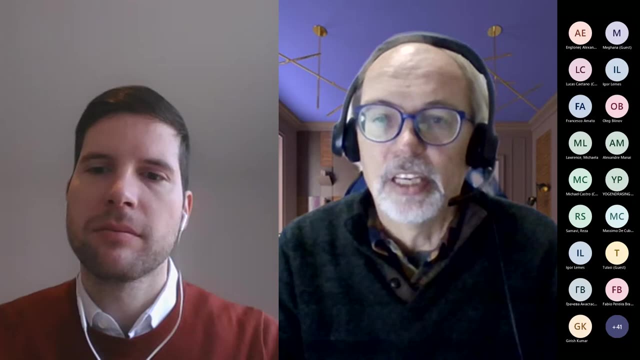 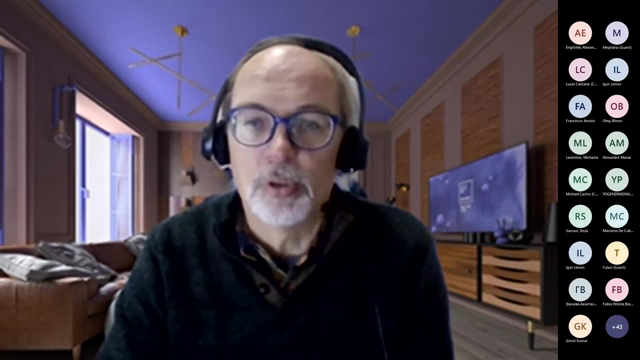 and, yeah, welcome to everyone in participating in- hopefully, this exciting new competition. Thank you, Jack, and yes, good day to everyone. I'm Ronald Jansen. I'm with the United Nations statistics division in New York, so it's still morning here, but I'm sure we have people from all around the world. 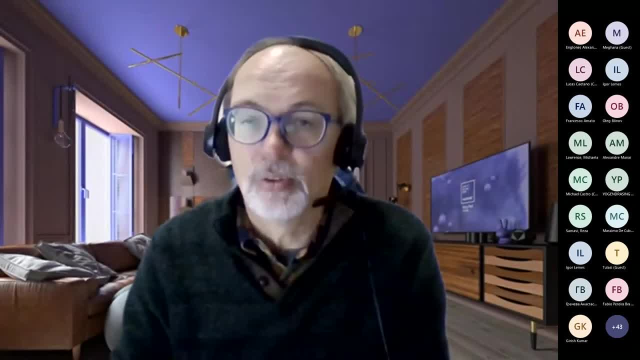 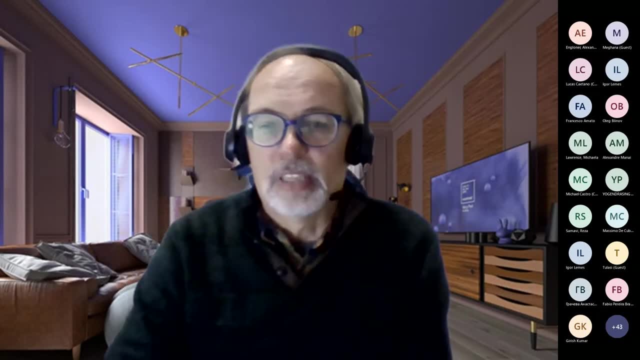 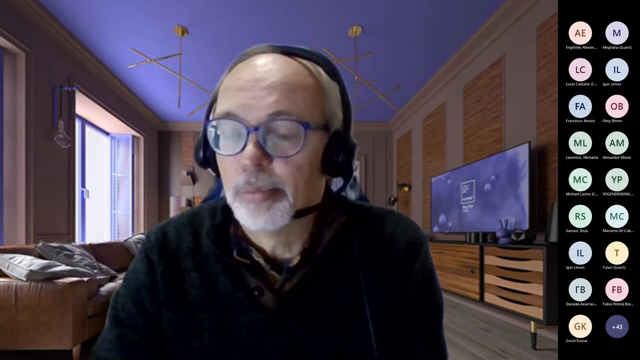 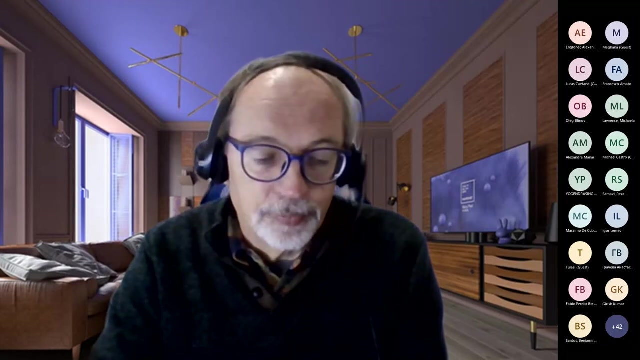 so thank you for connecting. I would like to spend a few minutes to give a little bit of context to where this hackathon fits in the overall picture. So the UN PATH lab, so the privacy enhancing technologies lab, is part of the United Nations committee of experts on big data and data science. for official 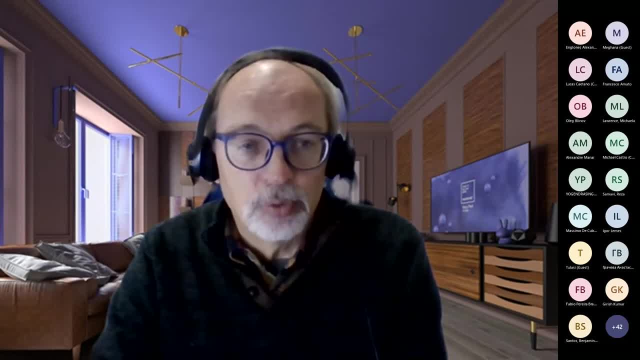 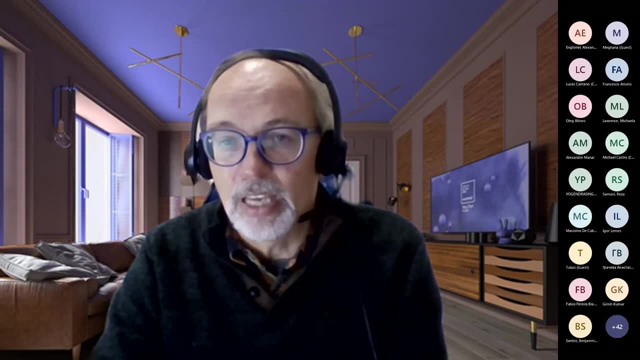 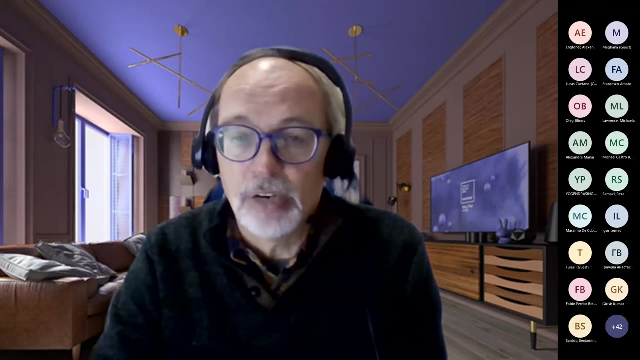 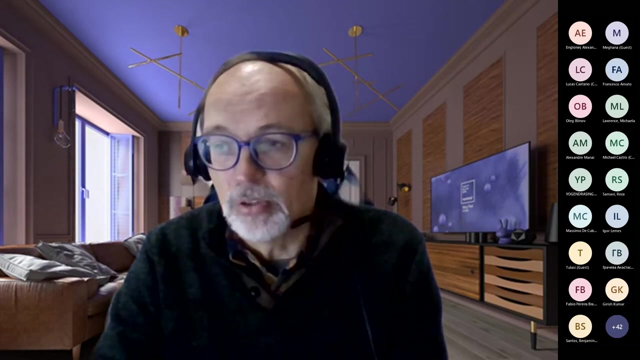 statistics. The community my office works for is the community of national statistical offices. so you have census bureau in the US, that's Canada- you have statistics in the Netherlands, but also the broader picture, we have statistical offices in Latin America and Africa and Asia. all part of the of this family of statistical institutes working for, for official statistics. 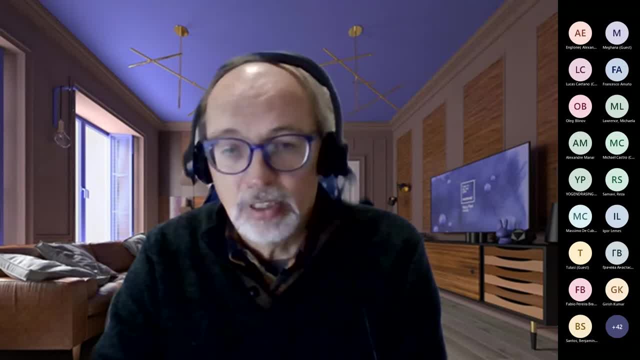 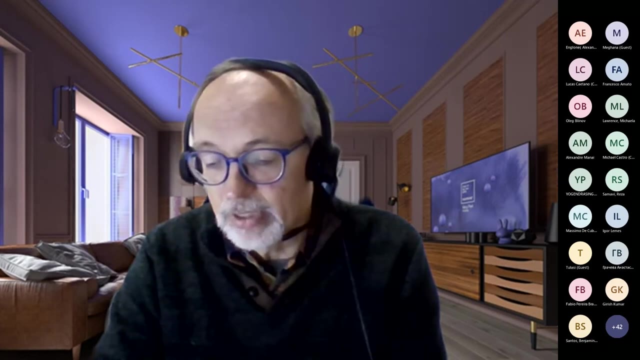 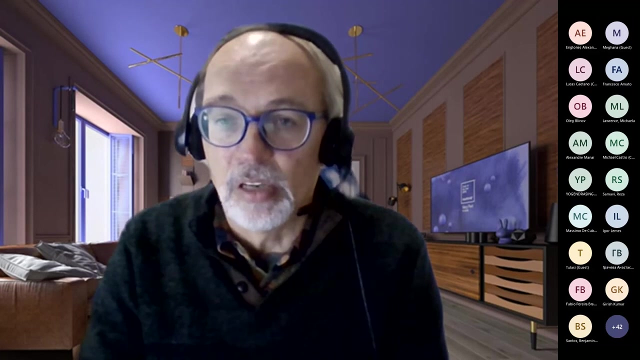 They come together every year in the statistical commission- that's usually around March at the United Nations, to discuss all topics on official statistics, so basically deciding, agreeing together what um our methods, recommendations, international recommendations are on on many topics over this population or or economics or environmental that be discussed, but also then in the area of 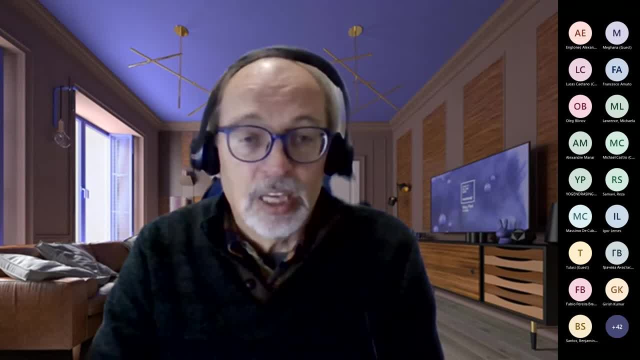 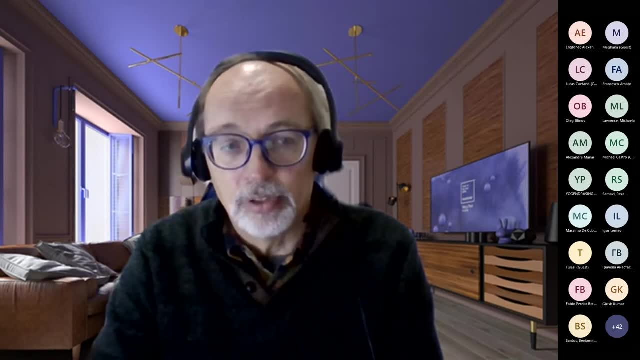 innovation. Innovation can be use of big data. A lot of it is also getting access to new data sources, getting access like to, to the use of logistics, totally just to touch on the practice of the data. so the use ofester traces and all of those sections start and then things change all the time. 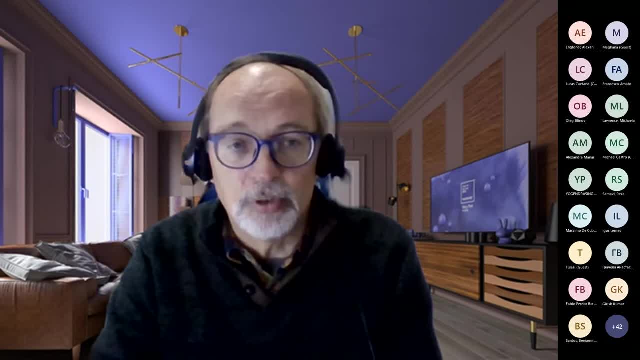 Now somebody needs to get a real sheet on two axes, which is very interesting this part. many scientists have tried to prevent many data sources from becoming explicit, but that's also not possible under ground, and these start and move rapidly: access like to, to the use of mobile phone data, to the use of other data that are that are sensitive. 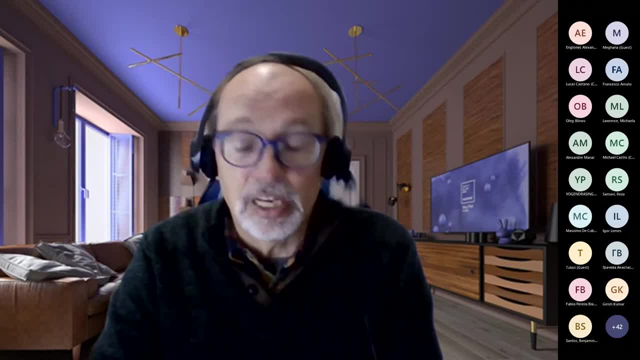 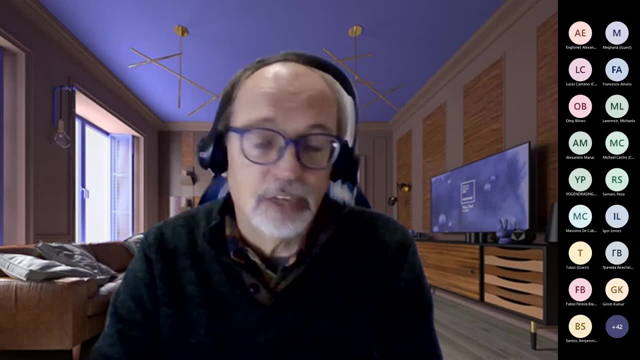 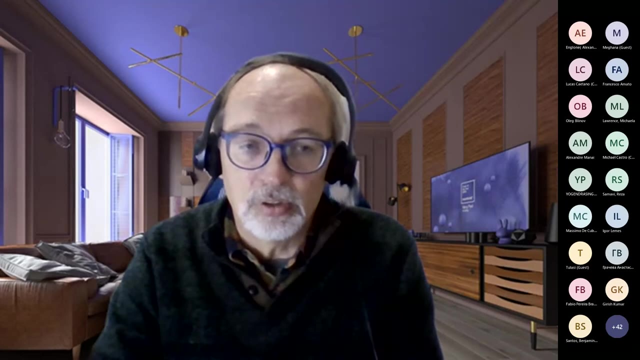 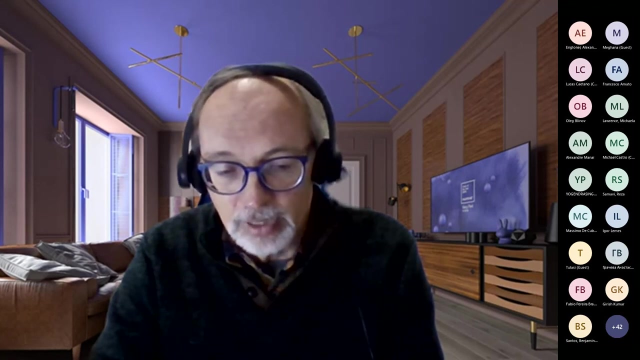 and that's where privacy enhancing technologies can help us a lot. also, statistical institutes do collect micro data, or they compile micro data and want to make it available to the research institutes or to research community or to other communities, and also at that end we we need to make sure that we have a privacy enhancing technologies. 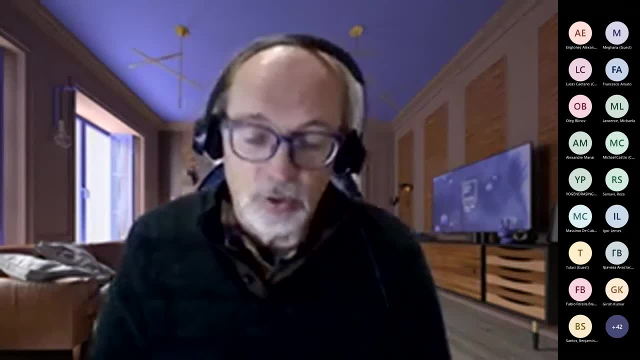 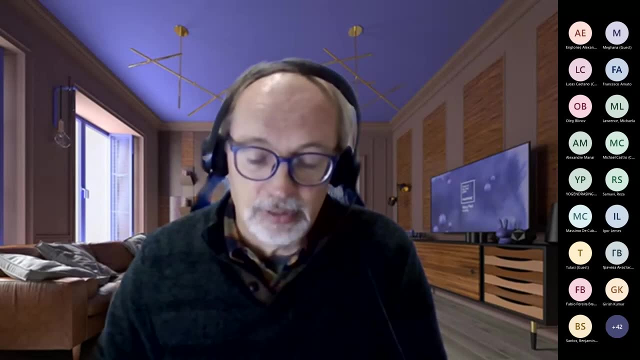 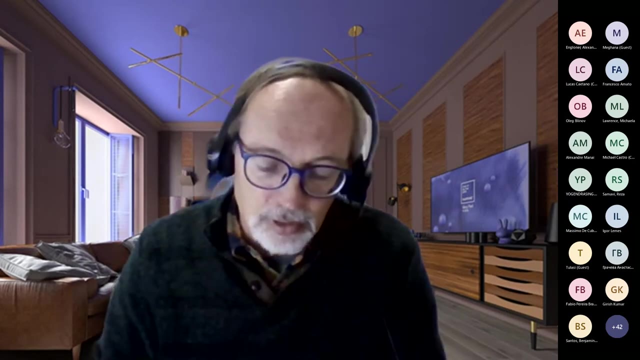 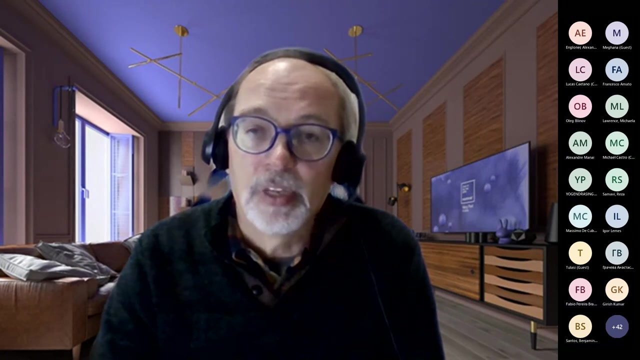 which which can make it can, can make it so that those data can be used by others without while protecting privacy, without violating any, any privacy of the sensitive data that that we have. so that is the context of of of the hackathon. a specific context is also the the conference that we are having in in indonesia. the conference 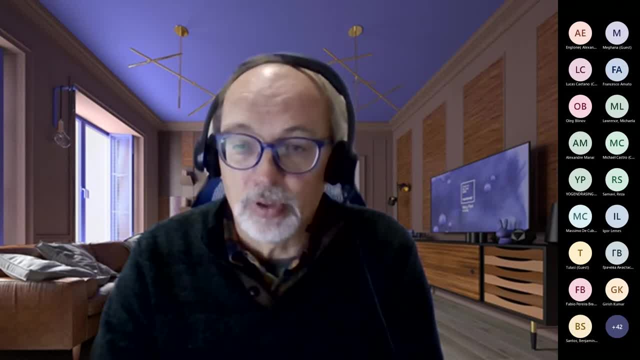 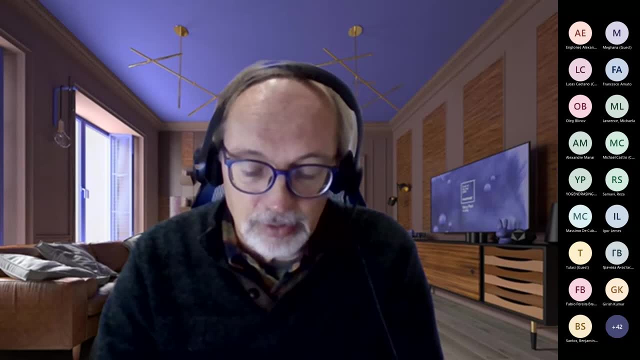 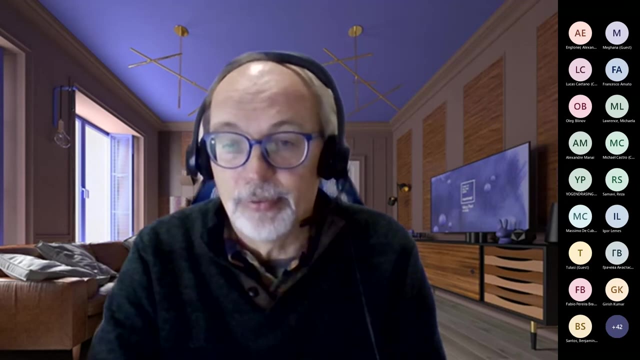 of this committee of experts on big data and data science for official statistics. the conference will take place in person from 7 to 11 november in yogyakarta, indonesia. on the opening day we will have there some high level officials from indonesia and from the un. the first day will really be a connection to 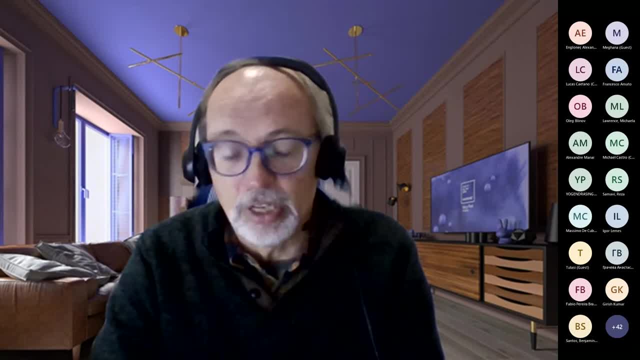 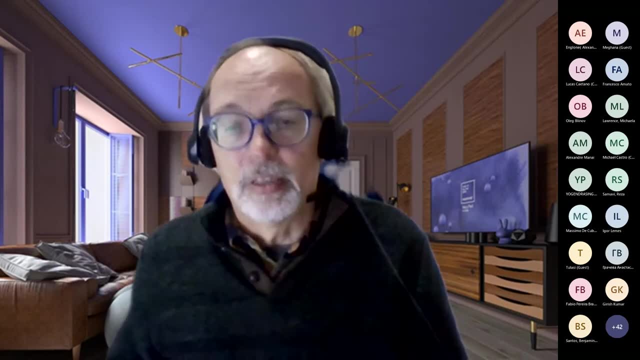 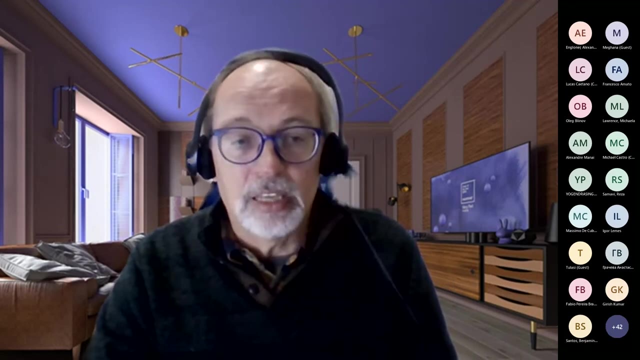 to those who are using sense, i mean who are using data for policy making. we will try to connect with the political agendas regarding global challenges like food security, like economic recovery, and we want to stress the point that, from our community's perspective, so access to relevant data is really important. 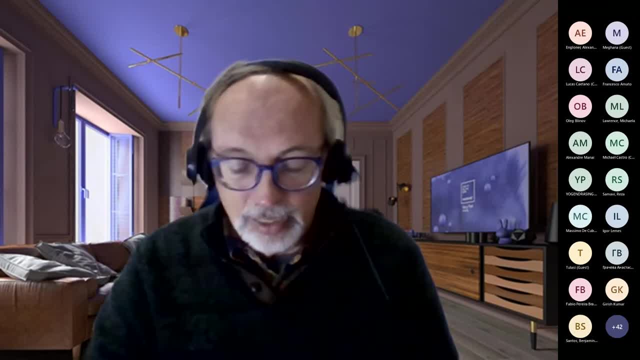 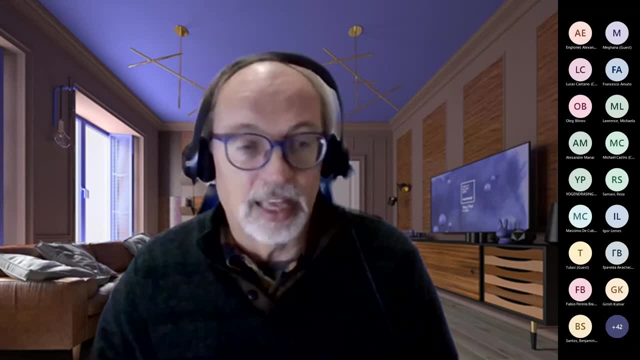 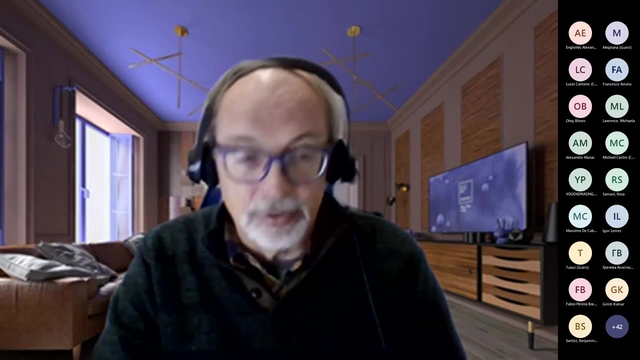 i hope you have seen the the website. so within that conference we have a few hackathons and in one of the hackathons is this hackathon on the use of of pets as an example of access to relevant data. we will have the access. we will discuss the. 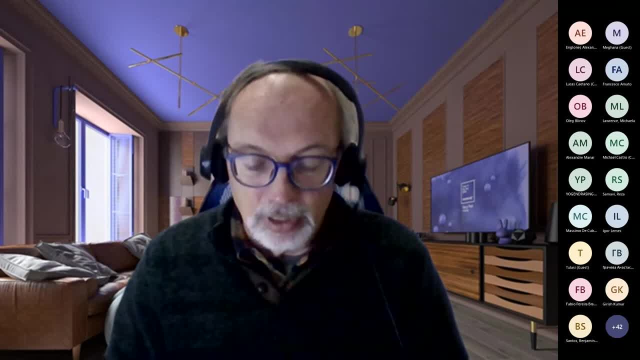 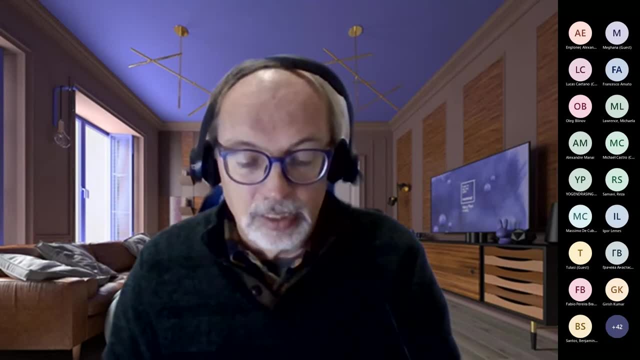 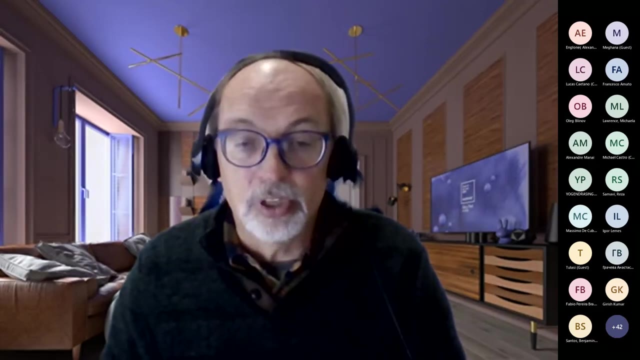 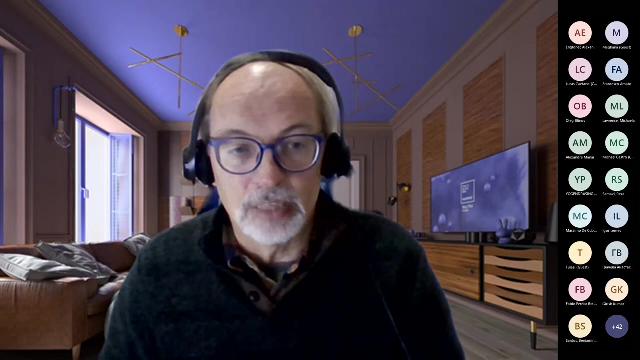 data from the uh on refugees from the uh, unhr and frederico will. we'll talk about that in a little bit, but i i think what the importance is also for us on this competition is to show that, um, that privacy enhancing technologies work, uh, that they can be used and that for the future of of our community, uh, it will be very important that we have. 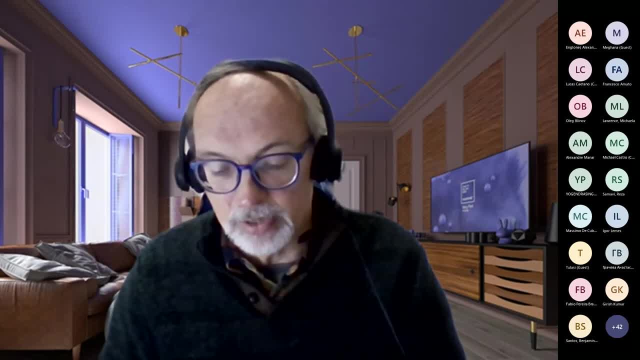 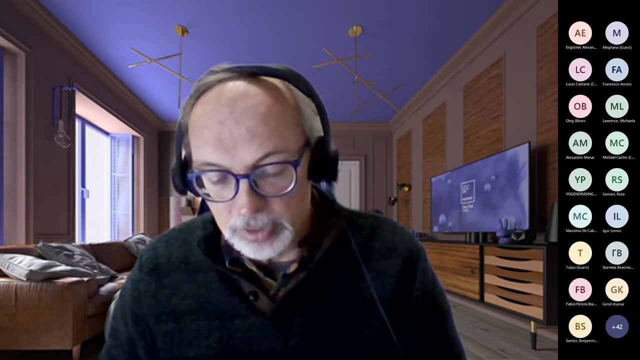 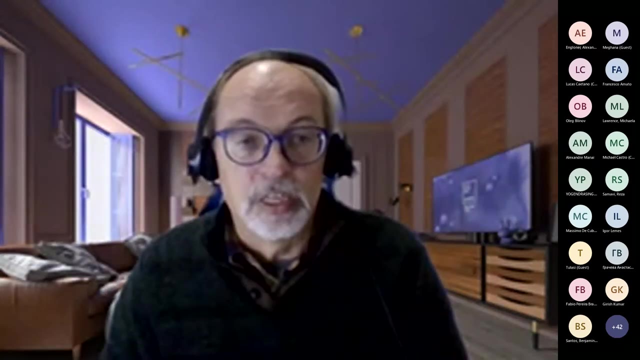 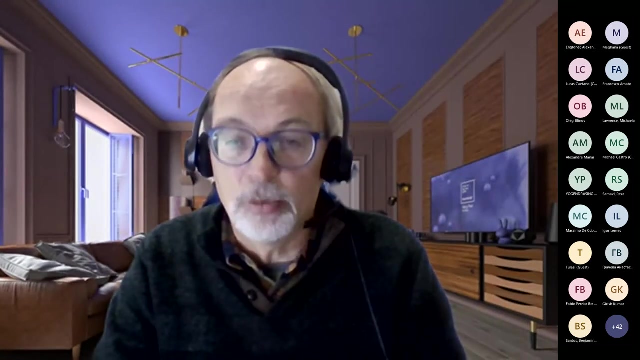 trustworthy pets that can be used by statistical officers to get access for the statistical offices to sensitive data and also for the statistical officers to be able to disseminate data to the society and researchers in a safe way. so with that i'll, i'll give back jack to you and i really wish everyone a great competition. 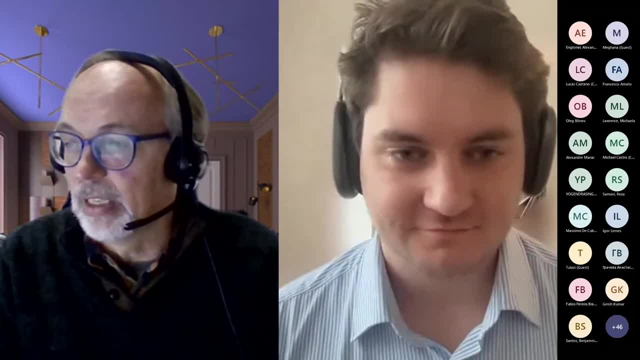 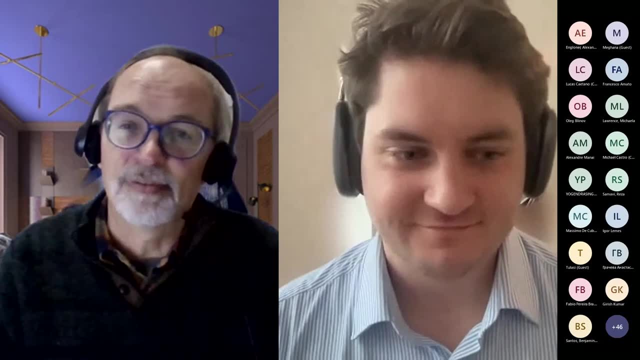 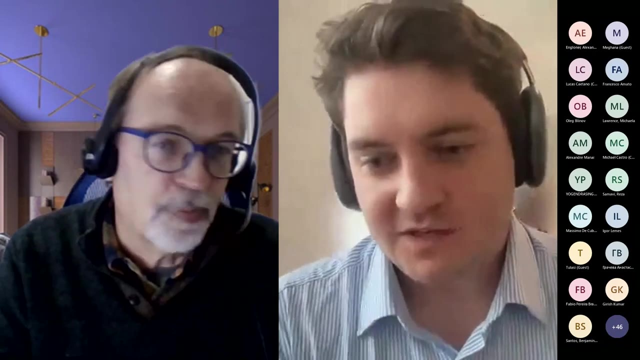 i hope you can see the broader picture. this is something that that is relevant and- and i hope that you really contribute and compete here- jack back to you. thanks so much, ronald. so you know, i think i think we hopefully have set some of the stage for why you know, privacy as a topic is is important and relevant, obviously within the 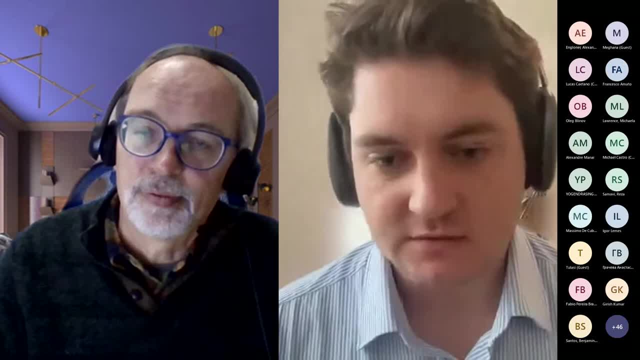 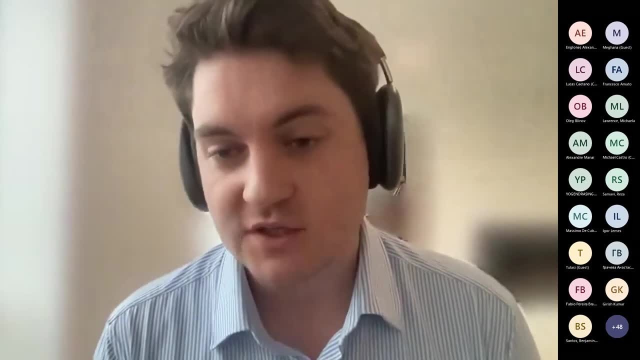 context of um of you know, nations and all of the national statistics communities around the world. but i always found that the real value is when you talk to someone who's actually worked on these challenges themselves and you kind of hear from their perspective the challenges that they have. and 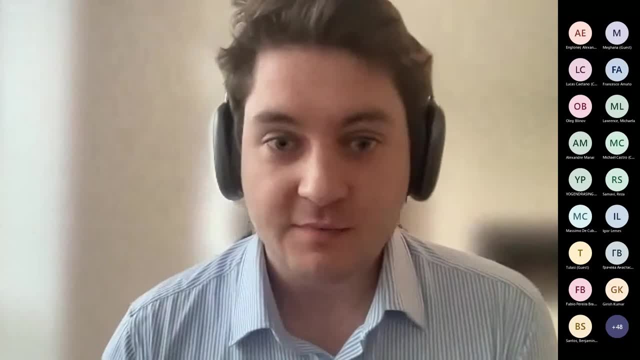 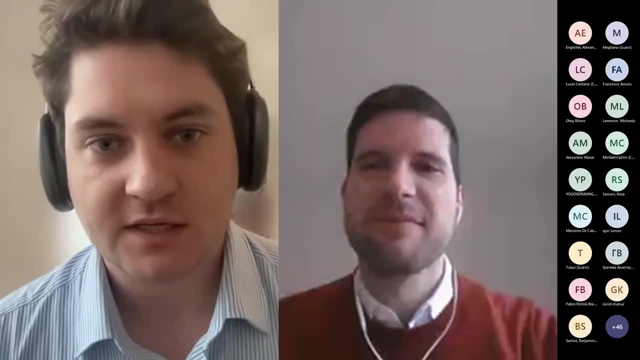 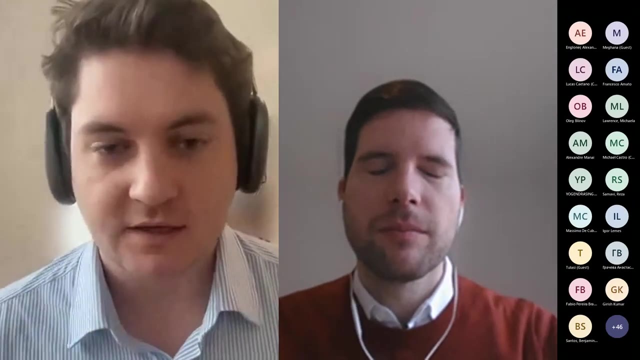 and and why it's important to their role. so we're very happy to have federico sanson, who's a regional data curator with the global data services team as part of unhcr, to speak to us now and tell us a little bit about, you know, their work and their challenges, and. 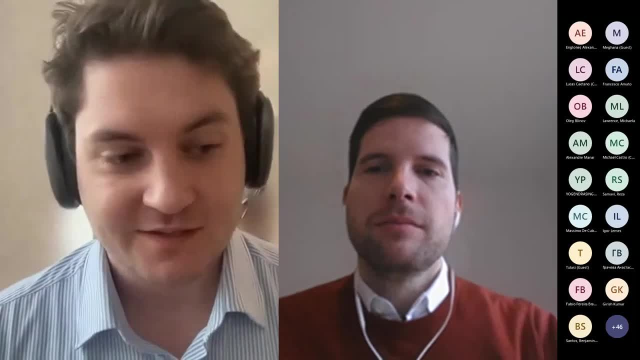 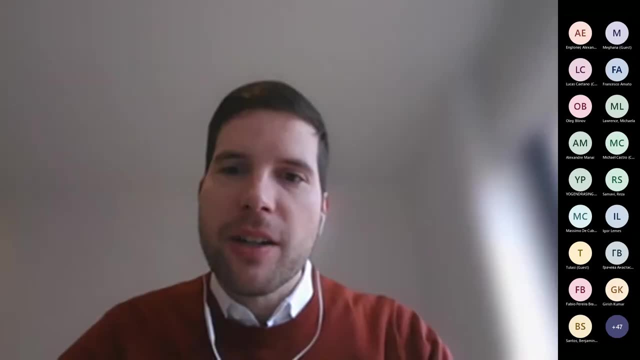 and how and why they exist, even as a team, in the first place. so i'll pass it over to federico and thank you very much for joining us. thank you, jack. good morning everyone. i'm federico sanson and i'm part of the data curation team, which, basically, we are the un refugee agency. 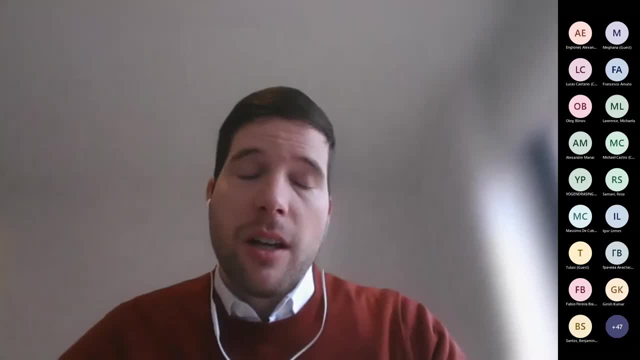 and part of the data curation team, which, basically, we are in charge of managing the data sets worldwide and making them available both internally and externally, with all the challenges that this brings. um. we are arguably the leader of refugee data. we make many data collections, many services every year- hundreds of them. so the challenge is to find. 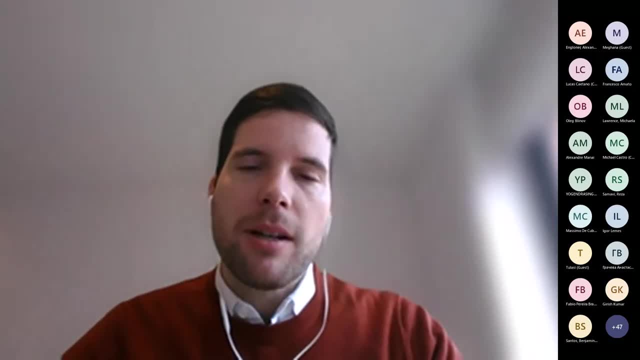 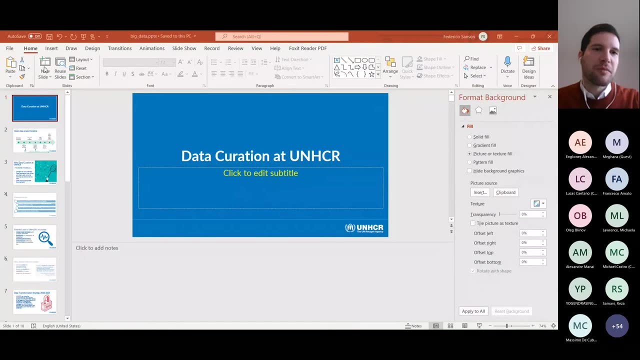 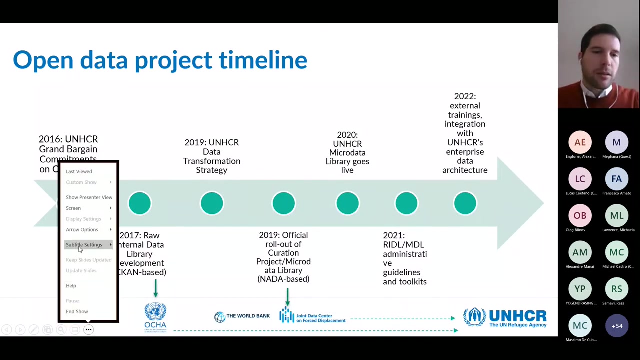 manage all these data sets and make them available, so i will share a short presentation. they probably will help to understand the better what we do. okay, so this is a process. um, our team is not that old, so we started doing the actual creation since 2019. 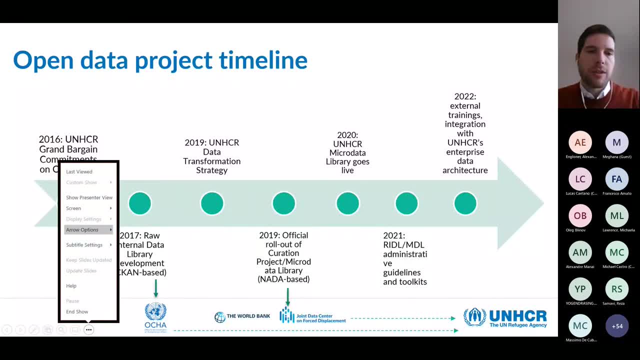 of course, there was already some data curation, but was not that standardized okay? so we improved these aspects and the whole idea is to make sure that all the data sets are available and that we are able to use them in the right way. so we are also in collaboration with other organizations to work on managing the data. 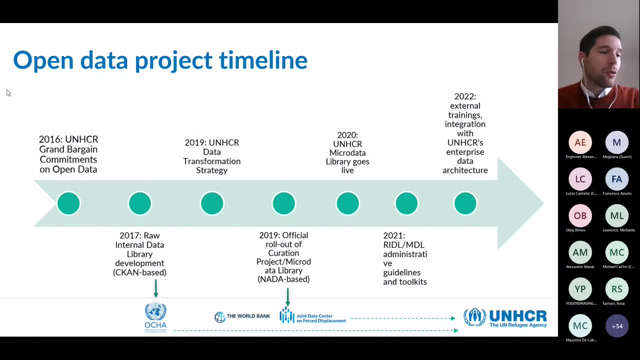 make it available, make it safe, and we are working towards open data and we are working on technologies to make these available for the reason pets are very, very interesting to us. we are working down, we are exploring these technologies and we keep studying them. so this is competition, is a big opportunity for us to test these technologies and to show that they are very useful for the purpose of open data. 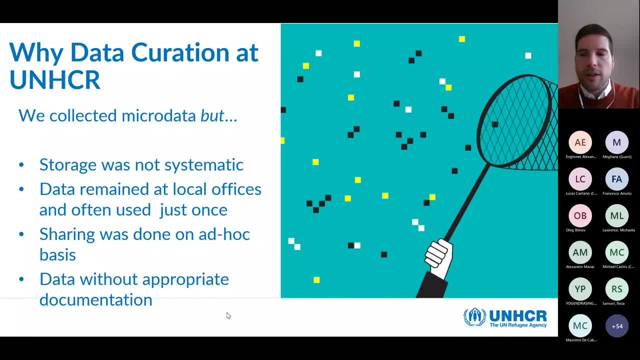 so before we did this data curation a very standardized way, we had many data collections, but there were few challenges, a few problems. first of all, the storage was not a systematization, So we have some tools for the data collection, in particular COBOL, if you're aware of it. 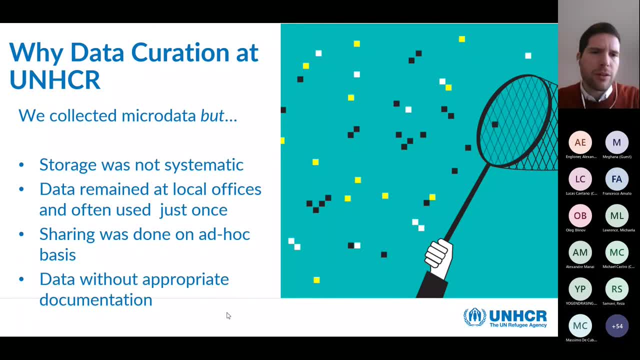 But what happened is that we had many data collections. These data collections were managed at local levels, So each operation, each country did their own data collection. They used the data collection for the purpose of the data collection, So they did one analysis. 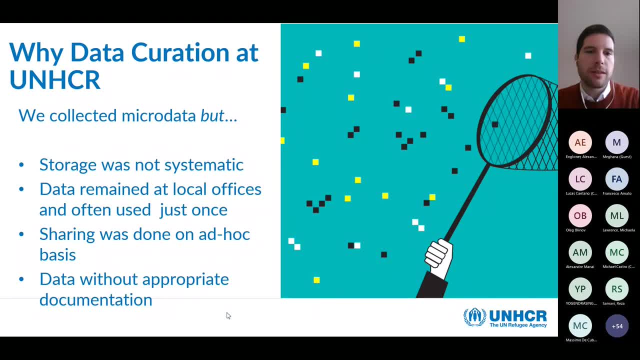 So most of the time they used just once the data and then the data was not used anymore, And so there was some issues with both the visibility of what data was available internally, So it was not so evident what data was available around the world. 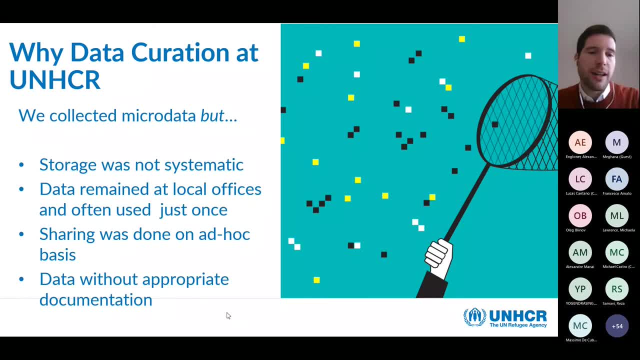 And also it was not easy to share the data, Because Before we had to share the data and create each time a custom HADOC agreement, Which took a lot of time and created many issues, Also because this was managed at local level. 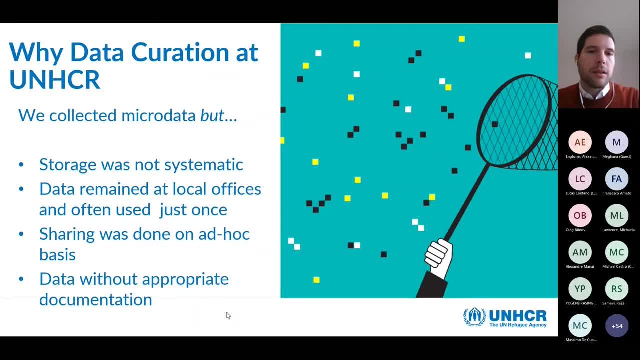 So there were many doubts And this was a big challenge to make it available both internally and externally. For this reason, we shared- We used to share the data externally, But Much less than now, And we did it only with the main organizations like the World Bank, all the UN agencies, few universities. 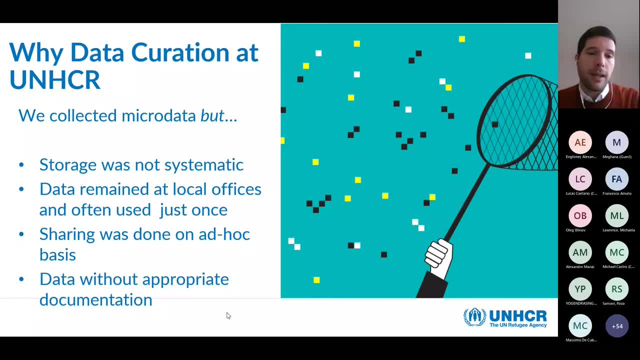 But it was very difficult to share it with many, many people, many researchers, many statistical offices, etc. The other issue was a lack of standardization in the documentation, So the lack of information metadata for each data set. Currently we use the DDI standard. 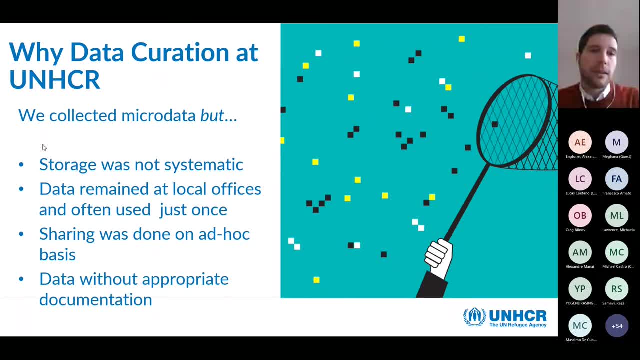 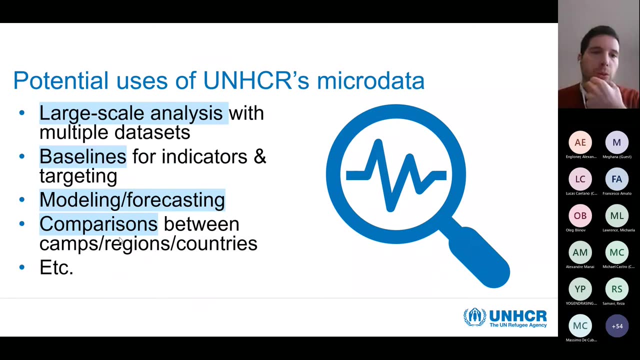 So it's also easier to understand the data set, the content of the data set, etc. Okay, So why we want to share this data? What's the potential? Is that large scale analysis will be possible. So we could combine. We could combine different data sets to make large analysis. 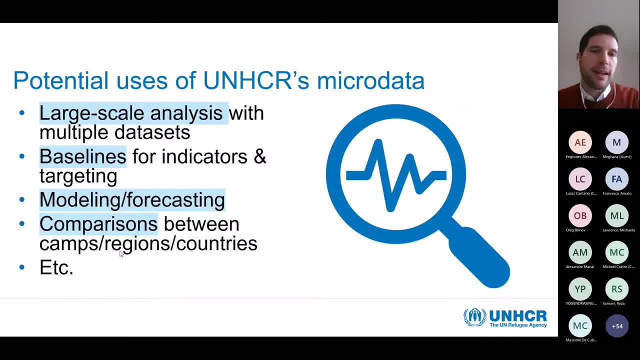 We can create indicators, baselines etc. Better models for forecasting. Also, we have the opportunity to compare between camps, regions, countries, different indicators Also to compare, to have year over year, to see the same kind of data collection So we can see the changes in data during the time, on how it evolves, etc. 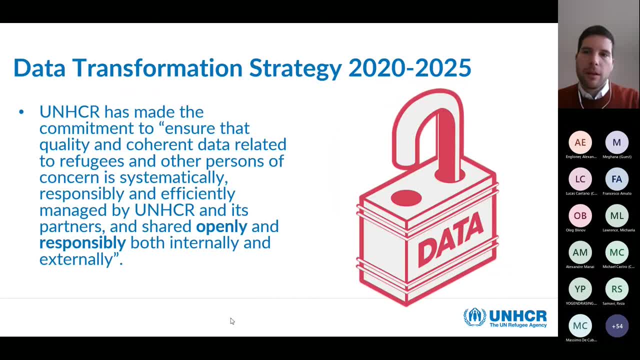 So we are working hard in this direction. We have data transformation strategy. Basically, the main reason we have it is to make it as much as possible available- open data. But these sharing data, both internal and external, of course brings many challenges. 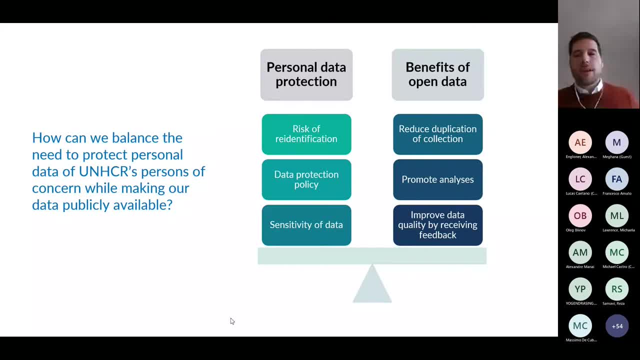 But these sharing data, both internal and external, of course, brings many challenges, and the main issue that we always take into account is to find the right balance between what we call privacy protection and the benefits, the utility of the data. so, of course, if you don't, 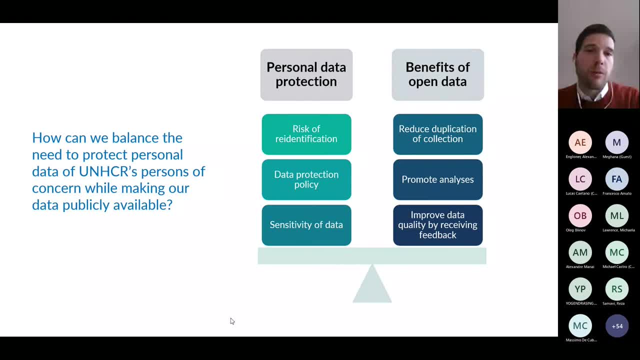 share anything. uh, you, that is going to be very protected, but the same time we lose a lot of utility or the opportunities that we are going to have, uh, or the data on the other side. we had to make sure the data is safe. that's why we are exploring new technology. the pets are very 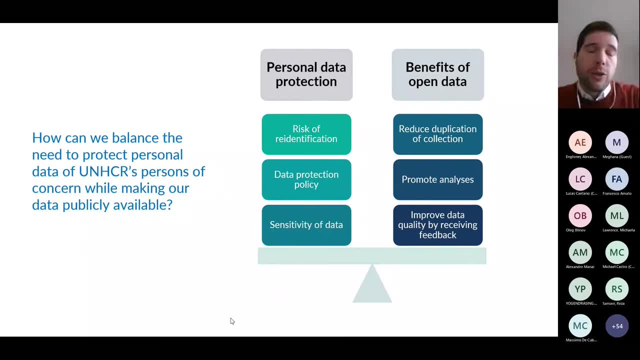 interesting and also take into account that unicr, the refugee data, is quite sensitive itself. first of all, well, there is the privacy in general, which refugee- but also the refugees is more vulnerable people. so we have to pay very strict attention to these aspects also, because there are 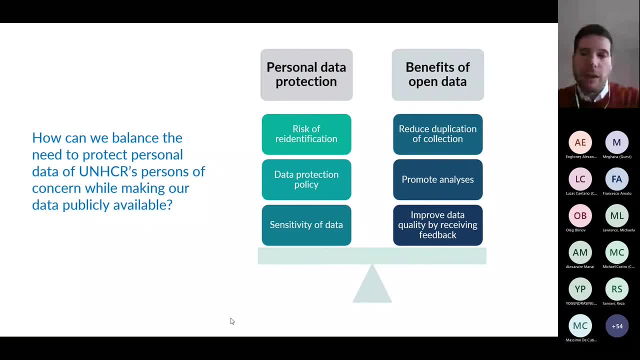 the refugee may be in danger for some particular reasons in particular particular reasons, or maybe because they belong to a minority and this may be the reason they prove for which they had to fled their country. so we had to be very careful to take into account also the sensitivity that could be specific of a certain community or certain country only. 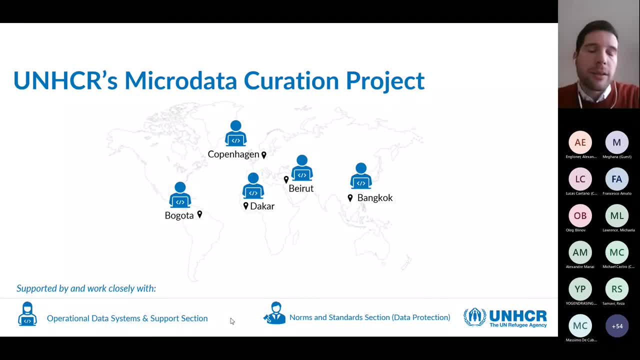 regarding our team, we have, i would say we have hq in denmark, in copenhagen, where we provide support worldwide, and then we have data creators around the world with idea to provide support to each region. personally, i am bogota, currently in colombia, just to give you an idea of the challenges that we have, as well as an organization we have. 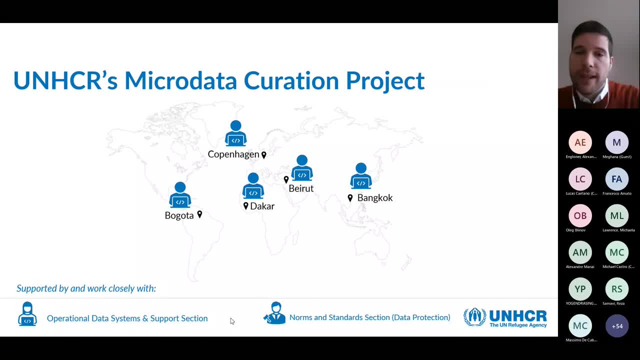 we are a very complex organization, very big but also very decentralized organization, where most of the work happens in the field. so the data collection happens in the field, is managed directly by each operation, by each country, and also what's interesting is that the ownership of the data belongs to the operation, so one when we want to share the data. 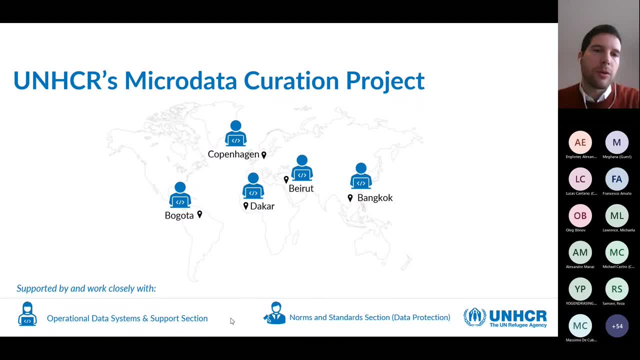 we want to work on the data, create the data, we need always the green light, approval or the operation of each country. so this brings many challenges because when we prepare the data, we need to discuss with each operation. and this is also where the pets technology are interesting, because the more we streamline the process of sharing data, 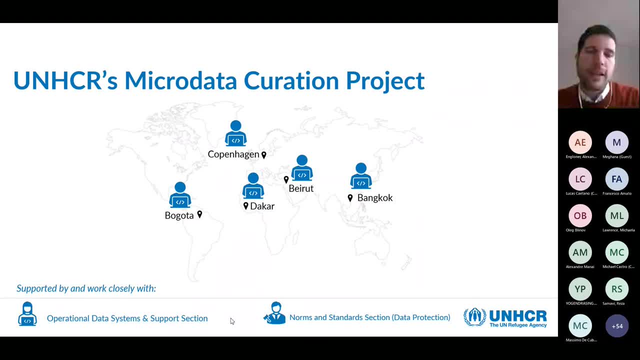 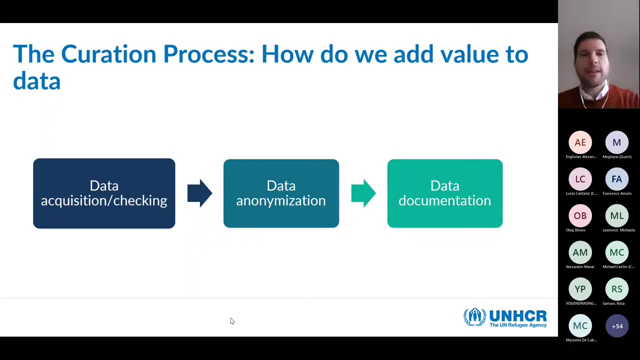 the more standardized, the easier and faster it gets to get the data outside and share this kind information. currently the curation process works like this: we work with operations to get the data, so it's the acquisition, we do some checks on the quality and eventually some cleaning. 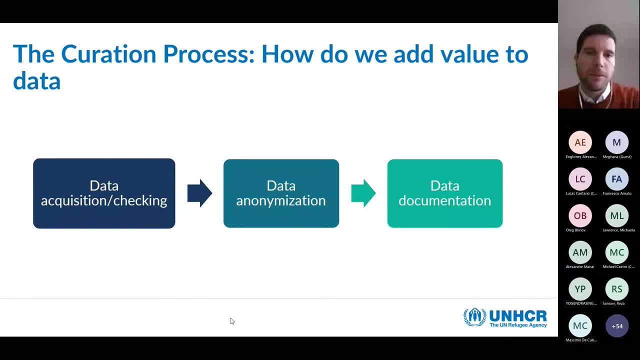 then there is the part of the minimization that we'll discuss soon. so we prepare the data for sharing and then we have the documentation, the data. currently, as i say, we follow that documentation initiative, ddi, so to make sure that data can be understand in this easier to work with. 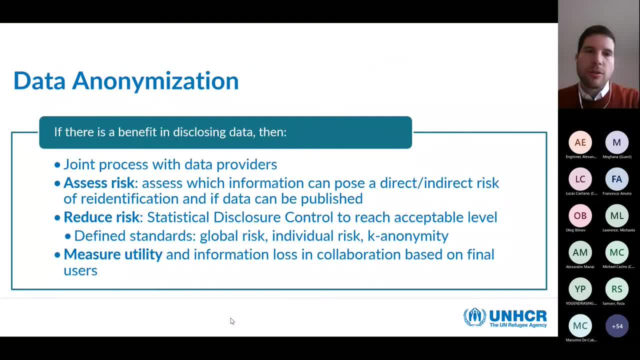 it. so now let's talk about the minimization. this is the current process that we have, which is slightly different. he has quite a bit difference with the kind of data sharing we are going to work in the hackathon, because the hackathon we're going to use mostly the 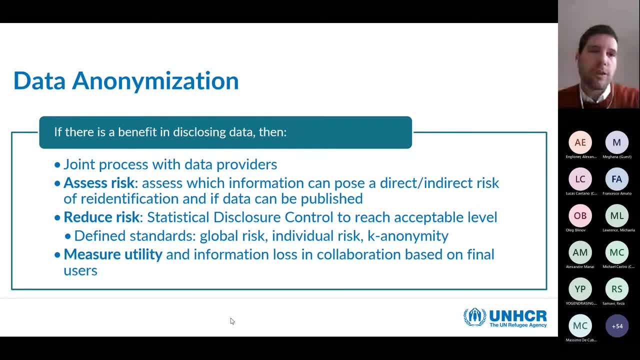 differential privacy, while currently in cr we are using that minimization uses, statistical disclosure, control the methods. they are different technologies- i would say Aristotle and Cons Huhu Brookes- but we also explain why differential privacy can be very, very interesting, very useful and provide solution to the limitation of the sdc methods. 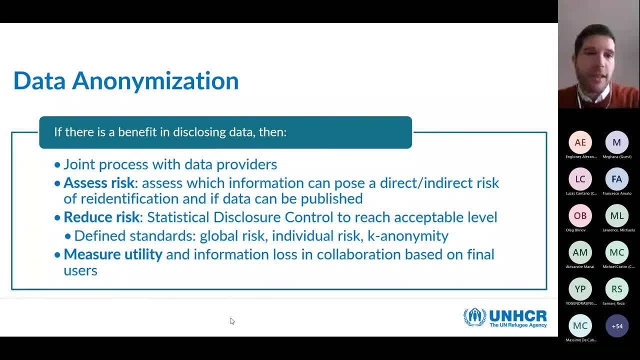 for the Shirin genomization. the process works like this: first of all, we have a process with data convergence provider. we have a process with the data provider. we have like majority square body of our common physics Performance Notice are at settings say, private resources be driven as a way to the solution. they can be deployed through different levels there. 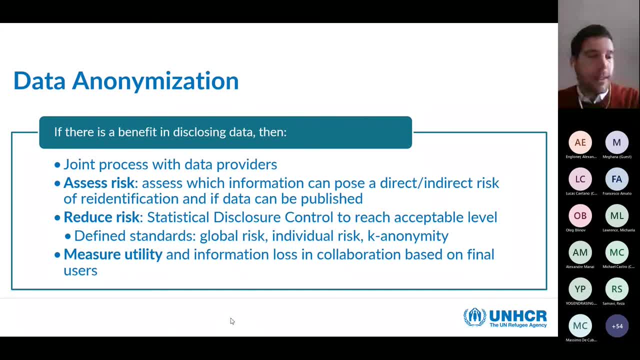 oure will explain some more processes for audible with" each country to discuss the particular characteristic of the data set. so the process standardized but still requires quite a bit of discussion with the operation because each data set has its own characteristics. we have to take into account also the characteristics of the 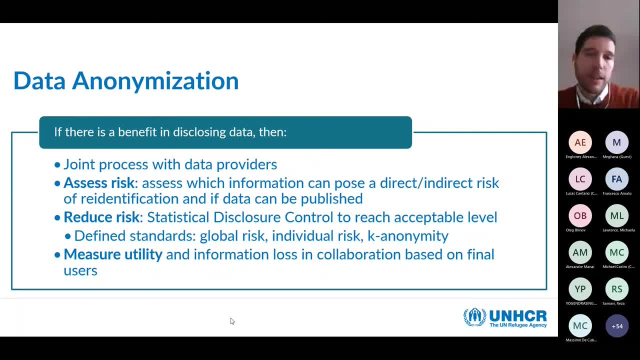 country. so we assess the risk and we have to notify the variables that could be used to re-identify somebody in the data set. then we work to reduce the the risk. that includes many different methods and these methods modify the data set. okay, so we modify the data set and we 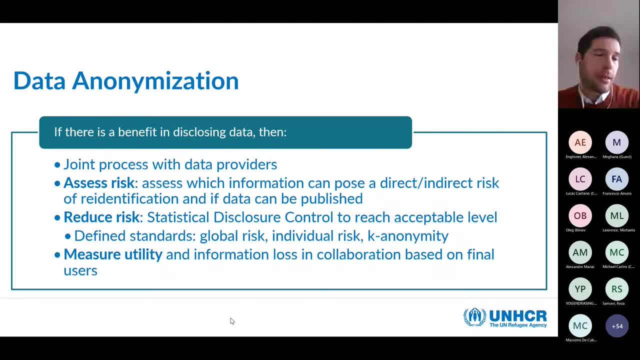 will share the macro data data set. this modify in respect of the original one, and that's why differential privacy is quite interesting, because differential privacy works on the original data set mostly. it gives you the opportunity to work on the original data set. it adds noise afterwards so it can provide better results and also, in some, for some data. 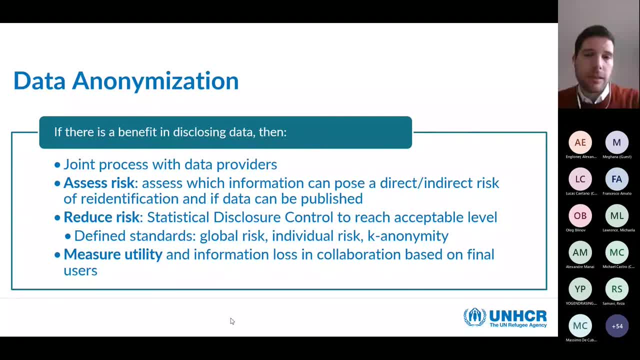 that i will explain later can be a game changer and that's why we are exploring these technologies. and finally, we measure utility, just to make sure that the modify data set will provide a similar results when they come in to the data set. and we use this to allow us to, as we see on the data set. 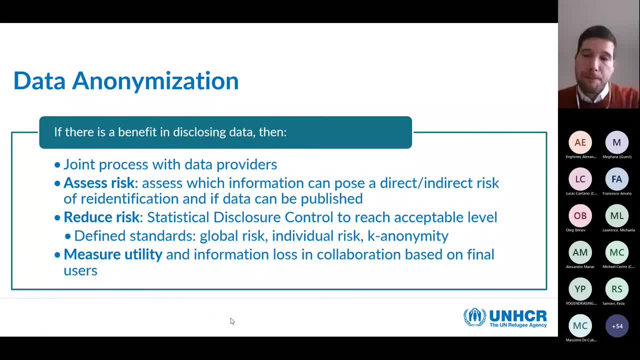 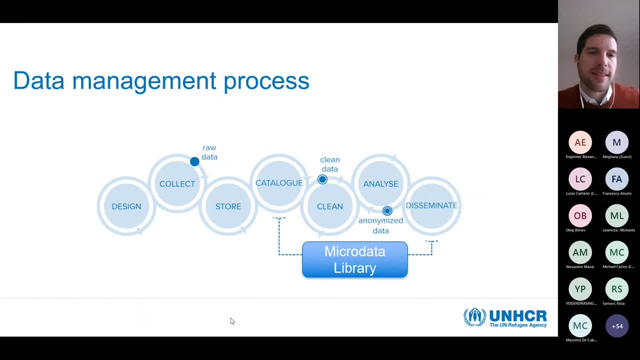 we are exploring these technologies and finally, we measure utility, just to make sure that the once you do an analysis and that's it. So just to give you the whole data management process as it is. now we start with the design, the survey. 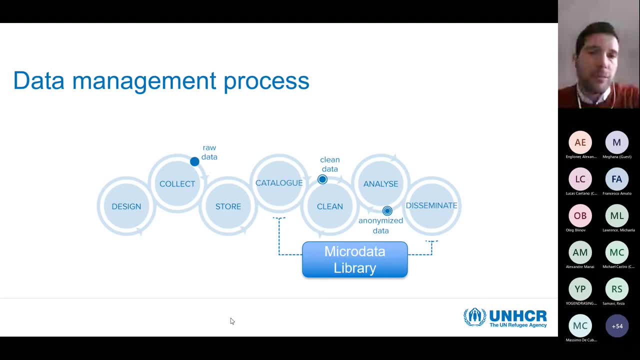 we do the collection of the data at the local level. we store the data and then there is the part operation. So we do the categorization, we do some cleaning, we analyze that eventually, and we do the anonymization and then we disseminate. 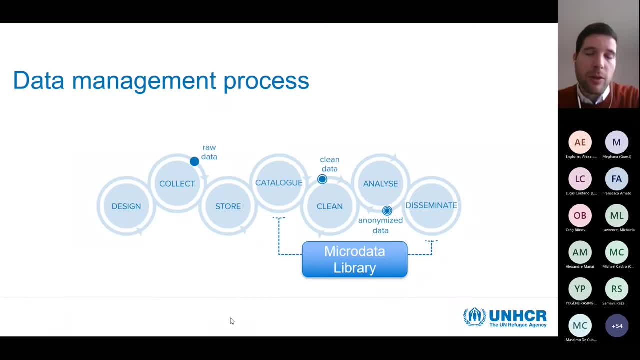 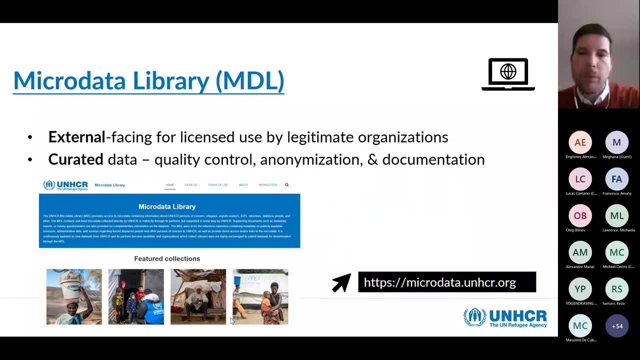 This dataset they get anonymized. Currently we have a macrodata library that we launched a few years ago and I'm going to show you. So it is available at macrodataunjcrorg, so I invite you to go and give a look. 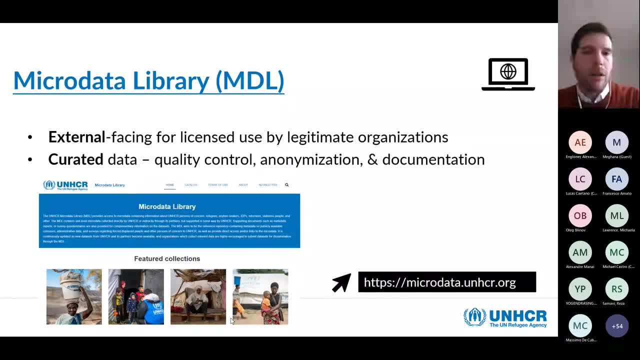 We have already many datasets available of refugee, internally displaced people, other people concerned. It is an external facing library with macrodata that's being anonymized. Most datasets are available under license, so you have to request the data and agree on not using the data. 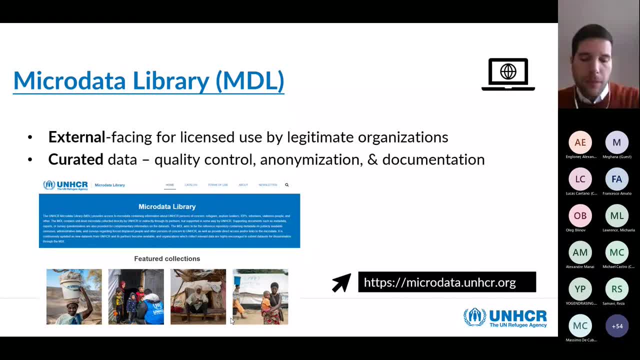 for other purposes, the analysis, So the data is given. the actual dataset has been modified under license. We like the idea of pets and if you have pets you can give them a認真, you can give them a real, real, real, real, real, real level of privacy. 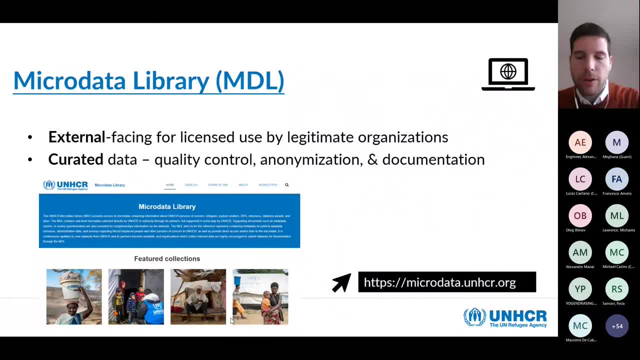 because they could give a higher level of protection, because we provide the data as the synthetic data or through differential privacy, not directly the dataset, While currently we provide an anonymized dataset. So we provide an actual dataset that can be downloaded and analyzed. 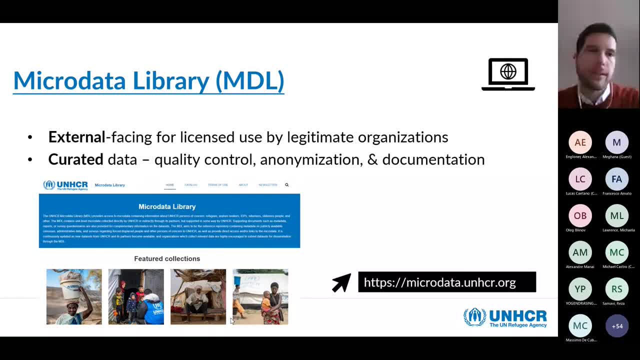 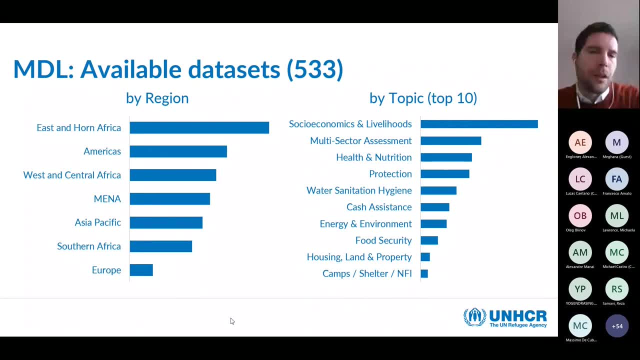 thing that can be interesting and if we can collaborate- currently we are- we have more than 500 data sets available, even if we started just a few years ago. you can see by region how many data we have. here is interesting to note: europe: we used to have around zero data sets for europe, but now, unfortunately, we say: 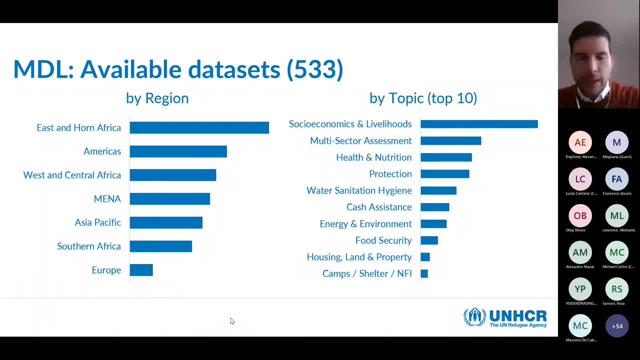 it's growing, as you know, for the situation in ukraine. so this is just to give you an idea that we work hard to make available data set as soon as possible, even if it's not always that easy, because the process currently takes some time and there's also white paths can be interesting. 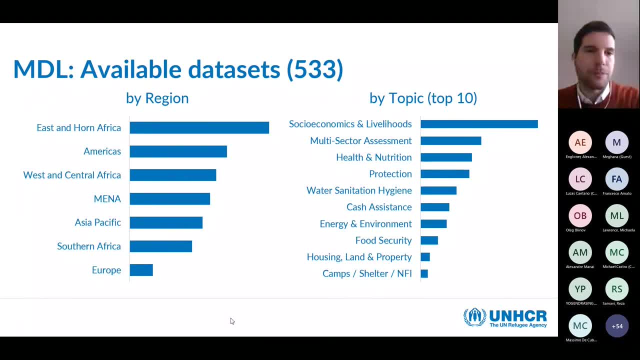 because it could streamline the process, and it's not always that easy because the process currently takes some time and there's also white paths can be interesting because it could streamline the process even more and, for example, we have many data set up in covid. that was the main topic for the past two years. 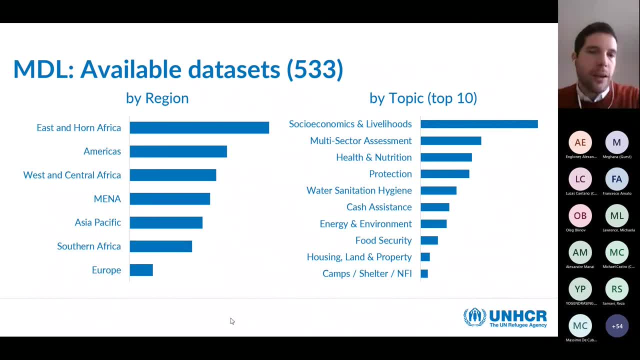 so we we always try to make available data sets that are interesting. currently they are the main topics. we work hard in this sense and that you can see also the main topics that we have so to give you an idea of the data we work on on umcr, so more the main category is socio-economic level looks. 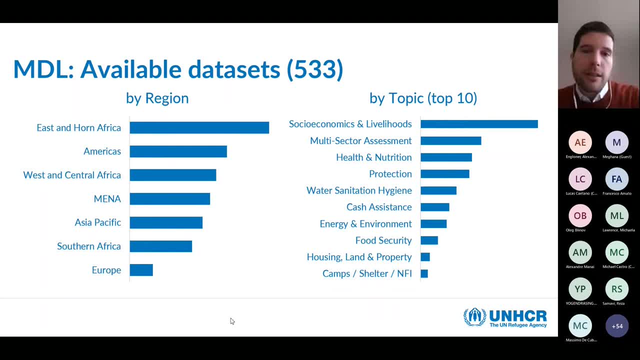 then we have generic multi-sectoral assessments: health and nutrition, particularly interesting for africa, where also we check, particularly important for children to see if their growing food nutrition is enough, etc. then we have protection uh data sets to see if there there are production needs, how we can address them. 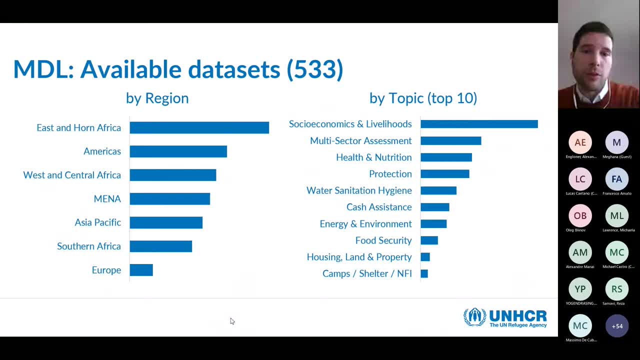 Another big category is the water sanitation. the water is water sanitation, hygiene. So if they have access to water facilities, if they have knowledge about hygiene, et cetera, et cetera, then we do a lot of cash assistance and we have after each cash assistance. 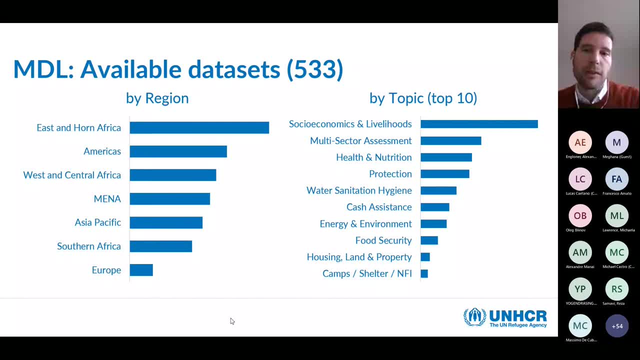 a post-distribution monitoring to see the effects of this assistance, And then we have other data sets. But anyway, since each operation work in its own, they do have their own. they're free. some freedom about the kind of survey. We have many ad hoc surveys for specific topics. 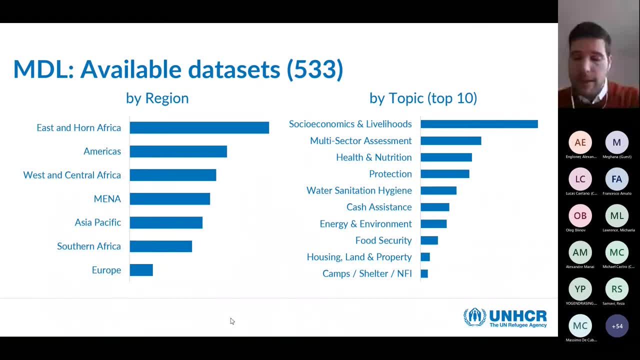 For example, since COVID was very important in the past two years, we have now many data sets about COVID, or in many data sets we included a section about COVID to have some information about the vaccinations, if they knew, if refugees have knowledge. 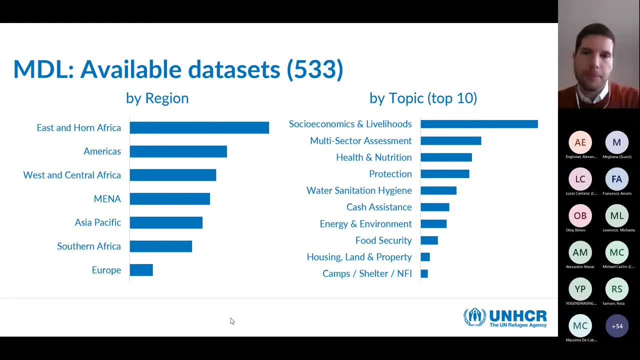 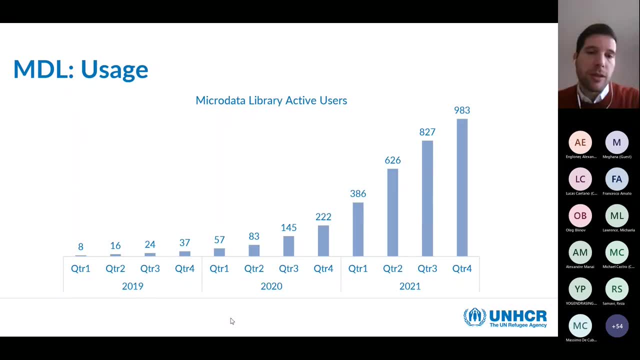 about the symptoms of COVID, et cetera, et cetera. Just to give you an idea about the usage. this is not really up to date, but it gives you an idea that we started in the last few years but the number of users they're using. 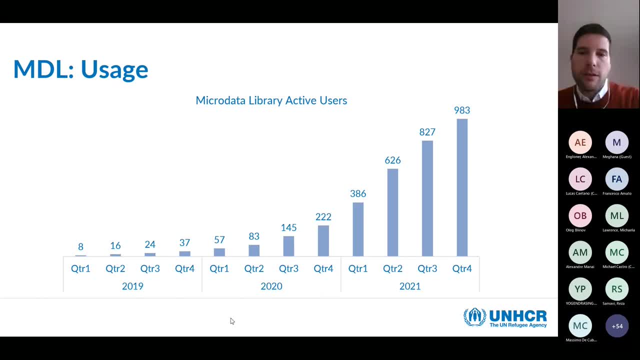 our library is growing exponentially. So this gives the idea of the great interest, the risk for this kind of information, this kind of data. So we really want to make this kind of data as much as possible available externally, because we can see big value in make this data available. 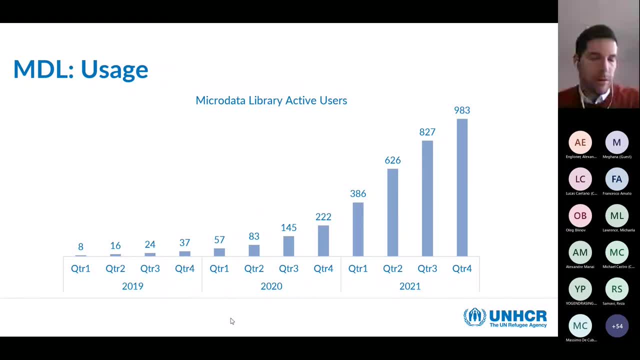 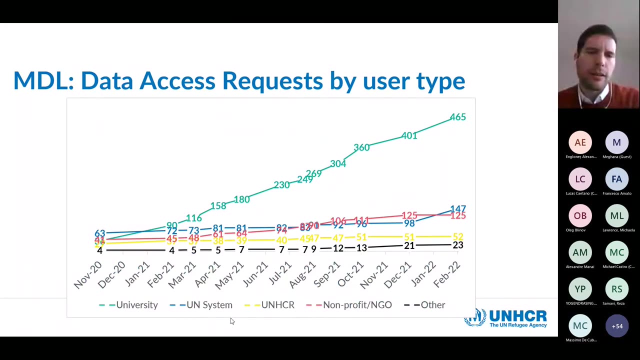 We already have many researchers that published some papers using our data, So we can see this very useful and we can collaborate together. And then, just to give you an idea on the kind of institution they are requesting the data, It's interesting that many comes from university. 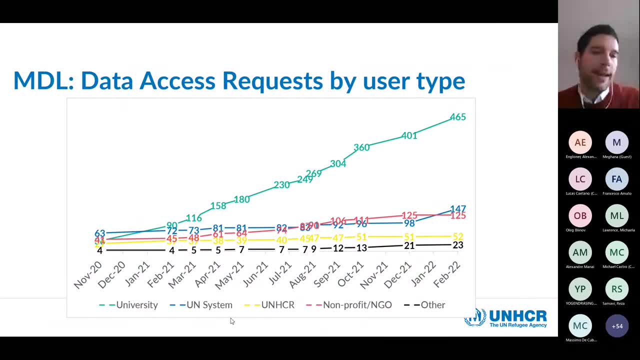 This is interesting because, as I explained before, we had to do some agreement- HADOC agreement- every time, So it was not really easy to share the data with every person, every researcher that wanted the data. So, using this kind of technology, 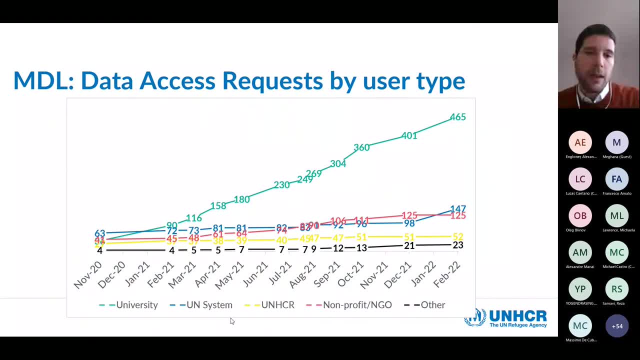 and we hope with PETS, to make it even more easy. it's easier to share the data with more people, with more institution- even the smaller one- with PhD candidates, with national statistic offices. So we see this number of data set that we share. 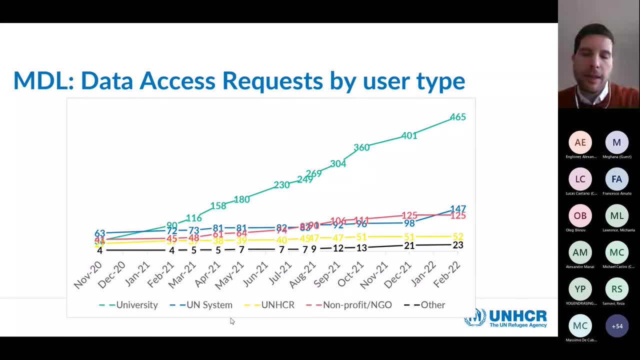 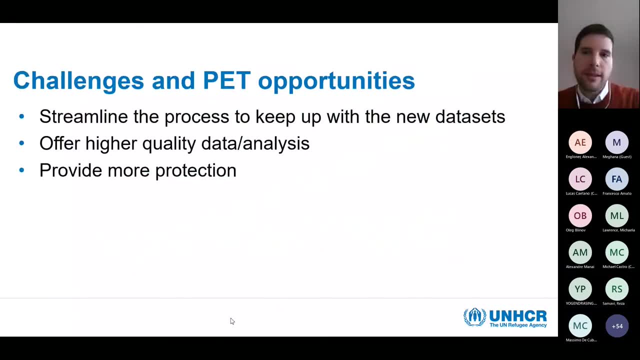 getting bigger and bigger and we can share also with smaller organizations and et cetera, et cetera. So to summarize everything, the challenges and the opportunities that PETS technology can give us is: first of all, we can see that PETS can give us. 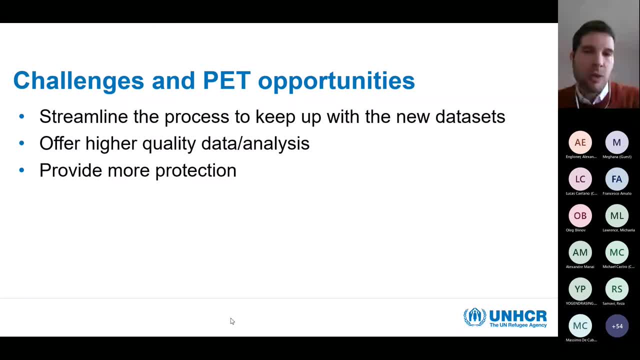 help us in streamlining the process. So we have hundreds of new data sets each year and we have to work on them, discuss which operation, which country, how to prepare them, et cetera, et cetera. So the more scalable is the process. 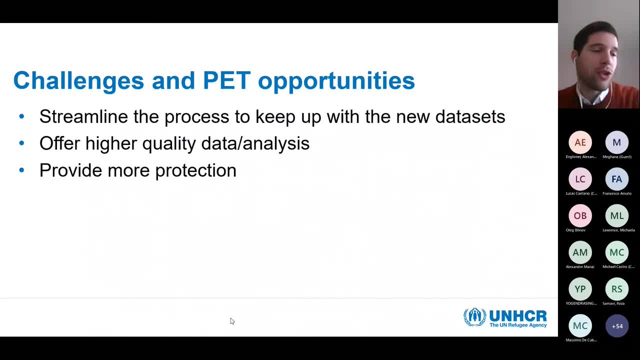 the more streamlined, the easier is to timely share the data set. So PETS can be very useful in this direction, especially differential privacy. we can see it as more scalable technology. Then we can offer higher quality of the data analysis because for some kind of data set, 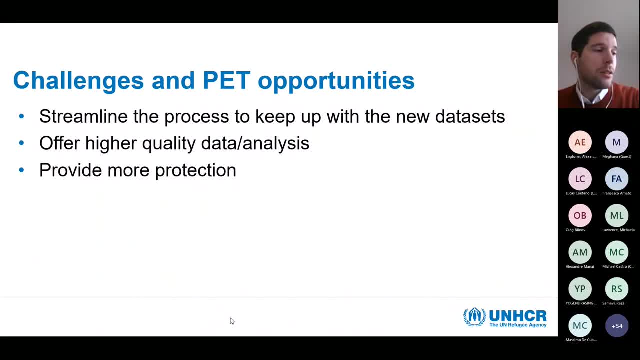 we can see as PETS, as a better opportunity. I showed before the kind of data set that we have. There is one important kind of data set. this is not yet available in the microdata library: this registration data. Registration data is basically a census. 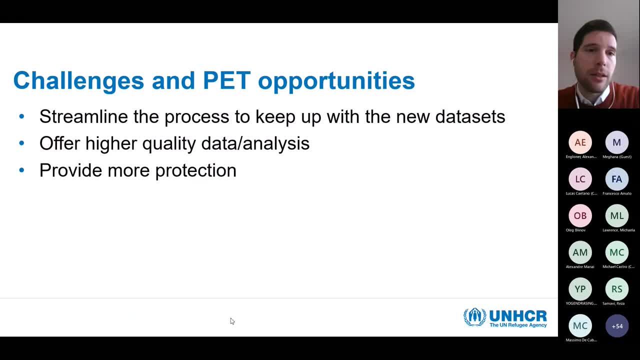 The idea is to have a census of all refugees in the world for each country. The data itself is mostly the demographics, but it is very important because it contains the data of each refugee, while all the data sets are mostly surveys done by sample. 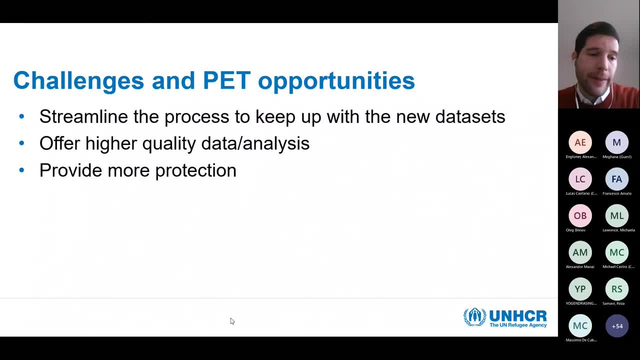 So this kind of data set is challenging to share it because it's a census, and in general it's challenges to share data set where the sample is big compared to the population and the event and if you want to share it using the current technology that we use, we will need 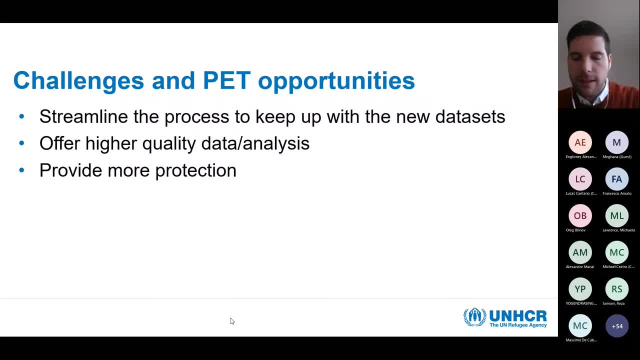 to do a sample of this data set or this census, so we will have to do, like a sample, five percent or less. with differential privacy or the pets, we can see the opportunity of providing a higher level precision of of the data because probably we will not need to modify the data, especially we 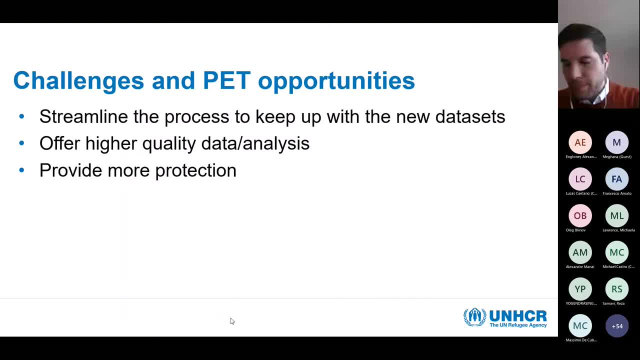 will not need to sample the data, but we could provide statistics based on the original data sets. and finally, we can see also the opportunity through pets to provide more protection because we will not need to share the actual data set. we could use differential privacy. we could provide a synthetic data data set. so, on my 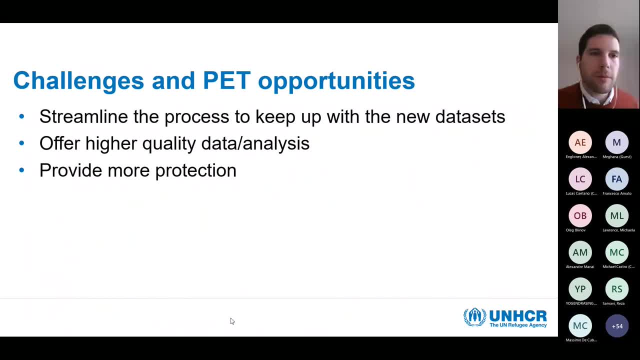 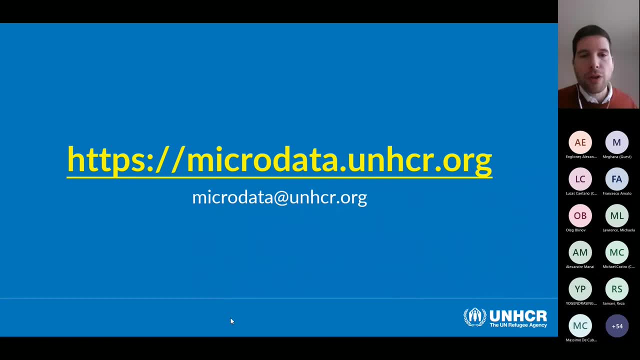 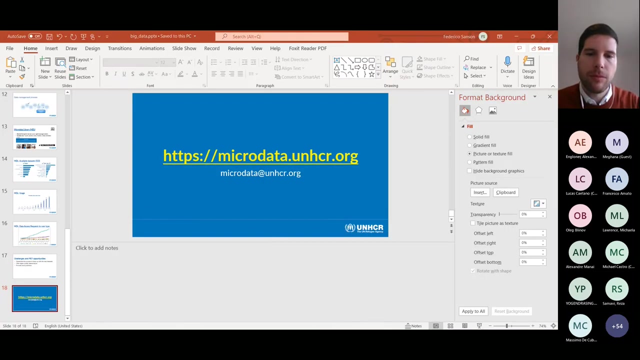 side. I think it's all. if there is any question, they're welcome. I just leave here the the link to the microdata library. again also our email, microdatacom. so don't hesitate to get in touch with us. thanks very much for Dr. I think one of the things that really stuck out for me when I first like. 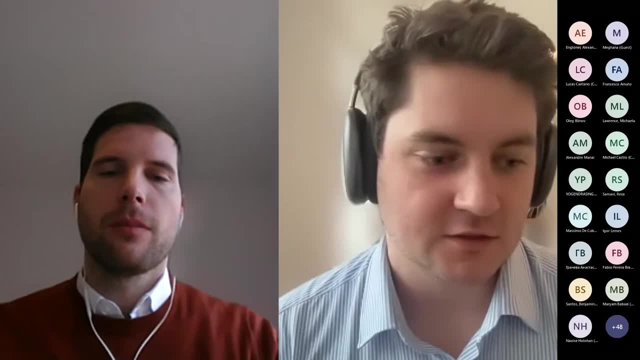 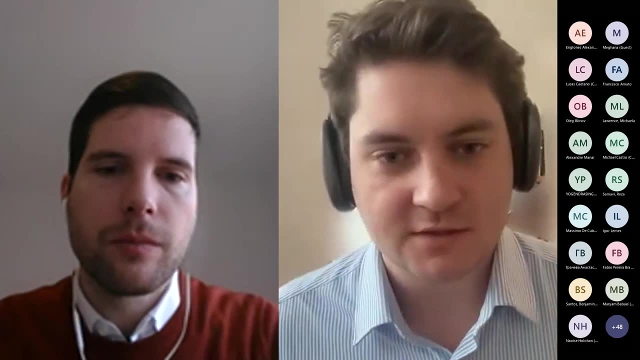 started to hear about the work that you guys do as well is kind of the sheer importance of it because you know, often you know people talk and hear about refugees all the time but there actually really are some of the most like vulnerable people in our broader society. usually they're leaving for. 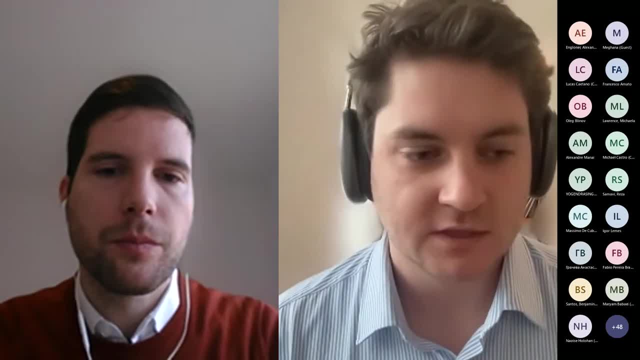 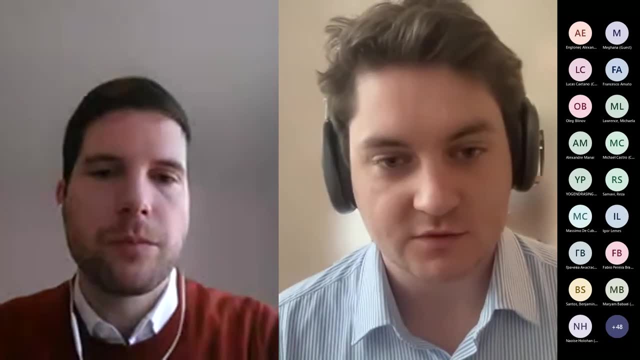 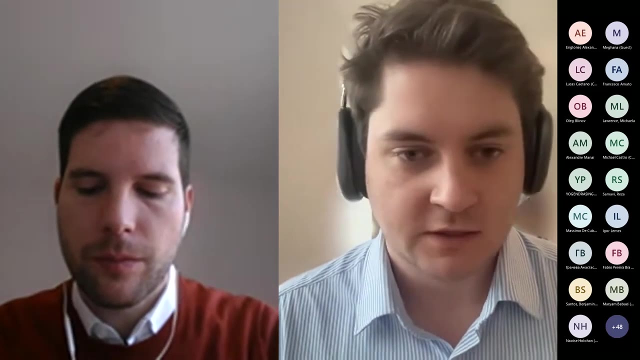 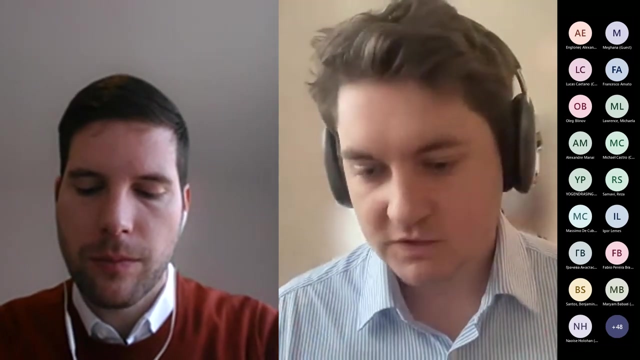 real and prominent reason. so i think the work that you guys do is incredibly important because it's fundamental to protecting so many people's identity and privacy, which is fundamentally important to them, while at the same time, as an organization, yeah, there's kind of a continued need to improve your ability to do data-driven insights and to share information with you know. 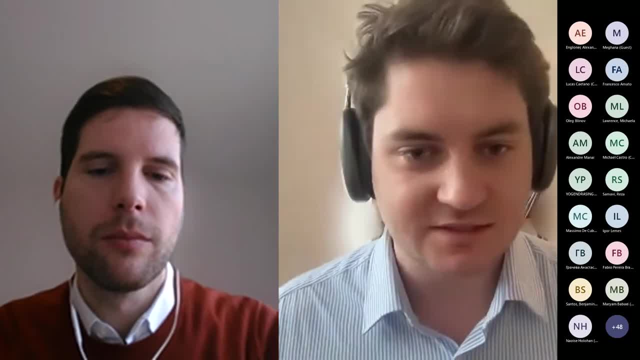 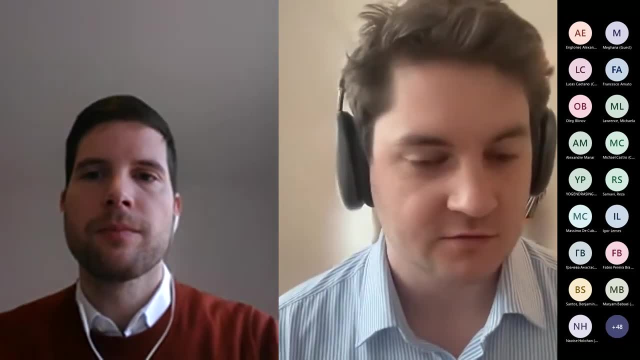 academia, governments, etc, etc. to be able to support uh- often in very short time periods, you know- uh developments in the area. so that's fantastic. i'm sure there will be a number. i can already see that there's some questions coming in, but it's okay, we'll pile them into the kind. 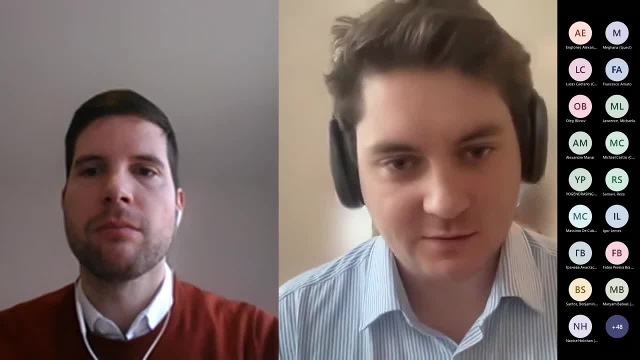 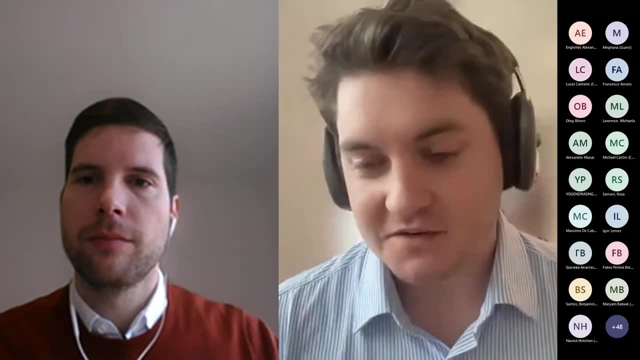 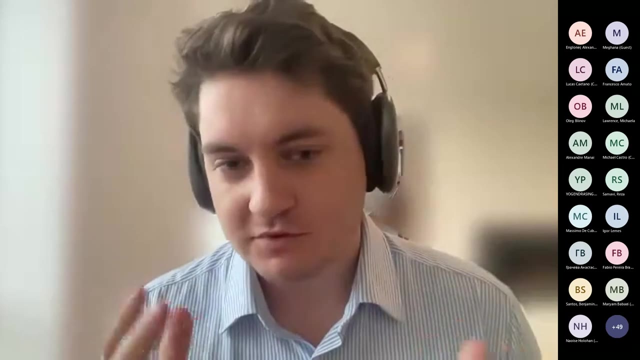 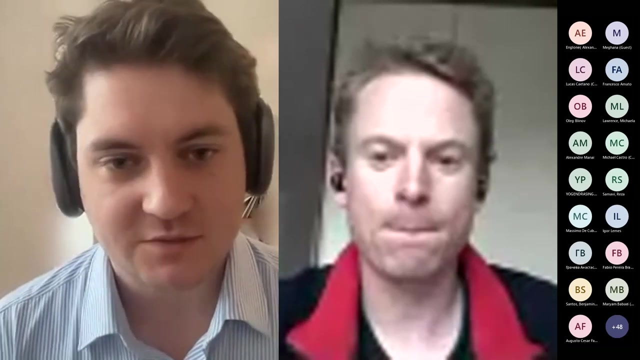 of q, a section at the end, and then we can discuss uh further. at that point, absolutely great. so the next speaker, and is a fellow irishman, nisha hallam, and he's the differential privacy kind of um lead researcher in ibm europe and his phd in differential privacy, um, and no better man to tell us what goes wrong. 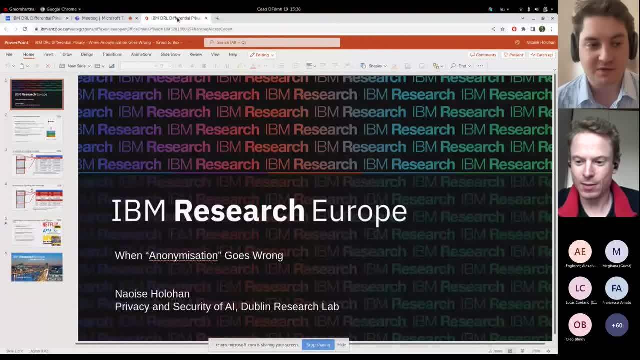 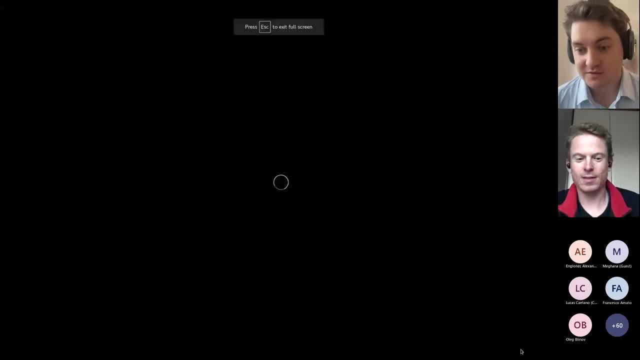 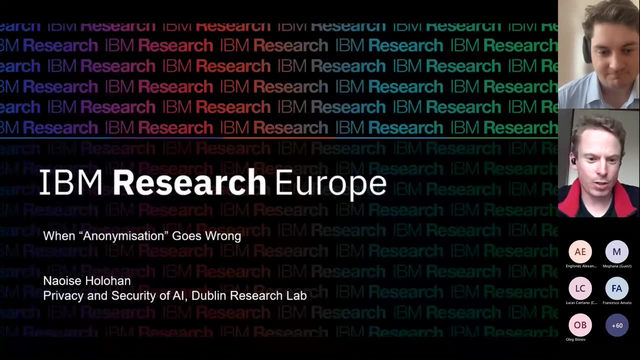 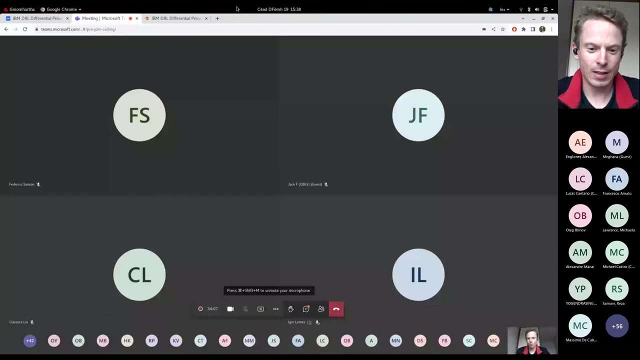 when we don't have structured controls in place um to to track and maintain what information we're actually releasing and disclosing when we share data sets, etc. so over to you, nisha, thanks very much. uh, hi jack, thank you very much. um just want to double check that you can see my screen before i. 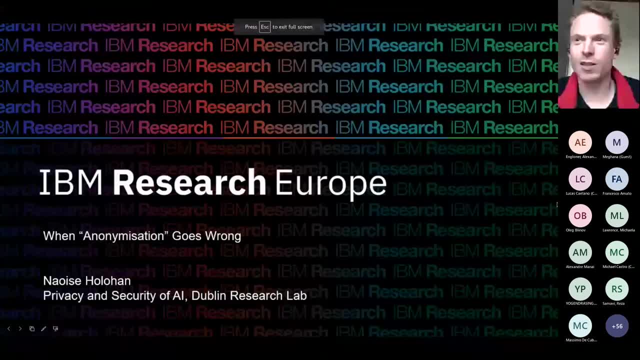 uh start speaking. um, it's a very wet and windy and stormy ireland at the moment. um, so, yeah, um, yeah, so, as jack was saying, uh, my name is nisha hooligan. i work in the privacy and security of ai team. uh, in ibm research in dublin here in ireland. 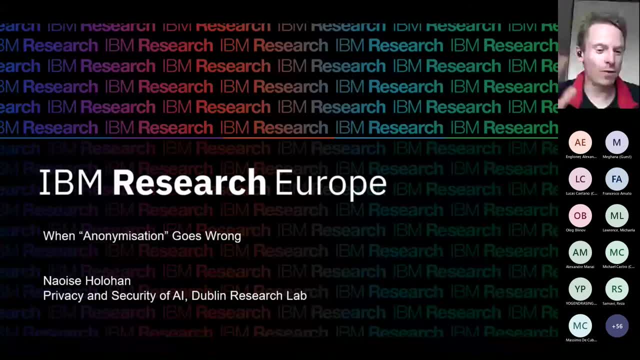 and i just want to give a quick kind of, i guess, a precursor to um, to robin james, speaking about differential privacy, which forms quite a, i guess, prominent role in this hackathon, and talking about the pitfalls of when anonymization and when data privacy goes wrong and i guess, in some respects, um, 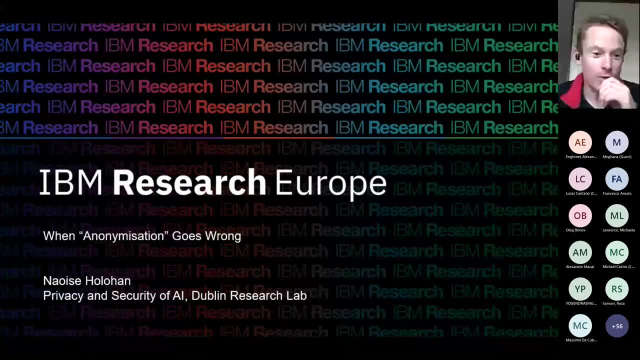 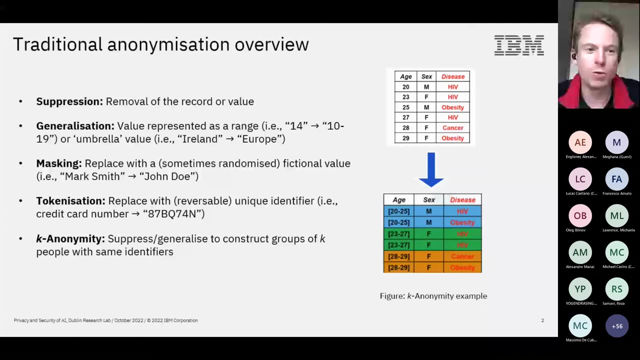 how is it that, early on in the thinking of these technologies, or older technologies, uh, give a false sense of security of the of their strength? um, so i'm going to start with a quick overview of what i term traditional anonymization, and these are typically deterministic tools that. 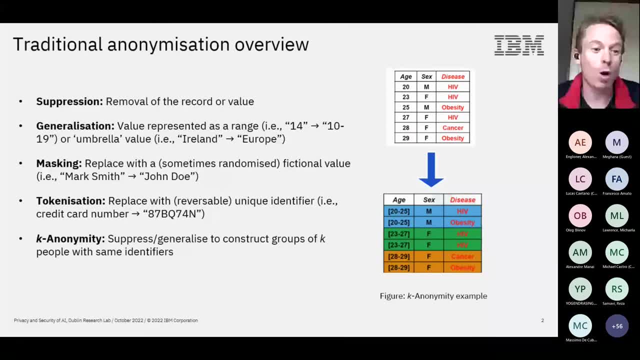 we use to remove sensitive or sensitivities in a data set that we want to publish or pass on to um external parties, for example, um. so suppression and generalization, where you, uh, remove entire rows or calls from a dataset, and rather, generalization when you, um, as it says, generalize this. so, for example, generalizing a. 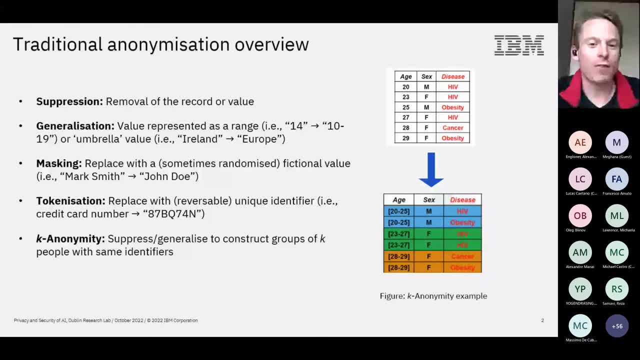 value to a range, or um if you have a hierarchy of values, for example, city to country to continent. um. masking and tokenization are also very important. masking is where you replace a value with a fictional or a randomized one, and tokenization when we um replace a sensitive. 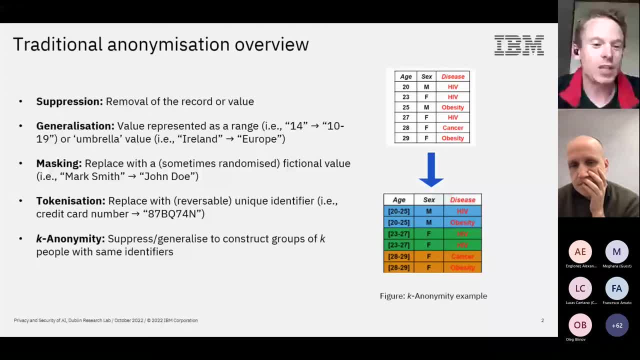 value with a, a unique identifier that we can still use to group transactions and things like that together. and then in the late 90s, the idea of k-anonymity was first conceived, where you use generalization and suppression of these kind of tools to preserve privacy, and there's an example: 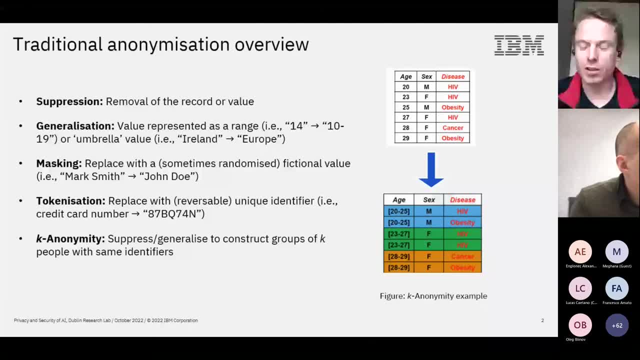 here. so i think it's always good to to work with an example. so in this example we've got two quasi identifiers, where a quasi identifier you can um link together to a unique identifier record, and then we've got a sensitive attribute, disease- that we're going to preserve, because that's kind 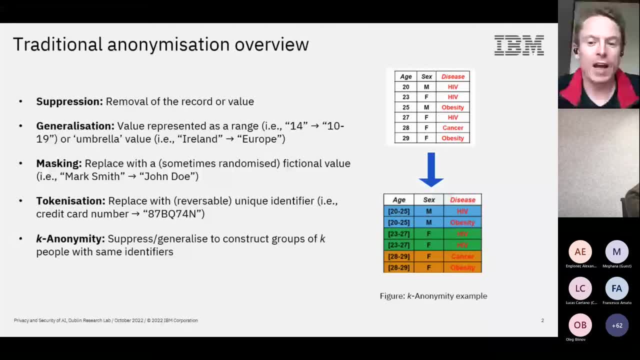 of the value that we have in this data set and we're going to generalize or suppress our age and sex to make sure that each combination of those in the anonymous data set appears at least k times, and for this k equals two. so you can see, in this colorful data set here we have, it's a two. 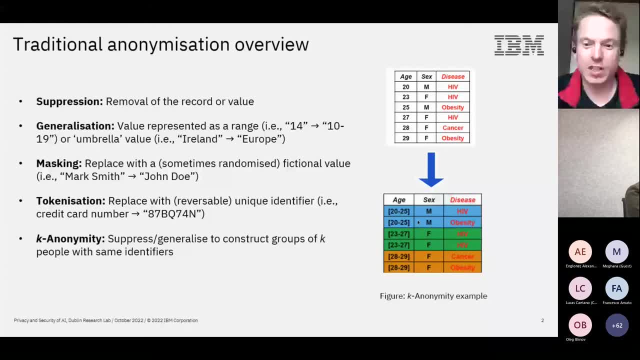 anonymous data set where each combination of age and sex appears at least twice. but the problem here is: if you know that we have a 23 year old female in the data set, then you automatically know that this person has hiv, and so in this instance, k anonymity hasn't really done a good. 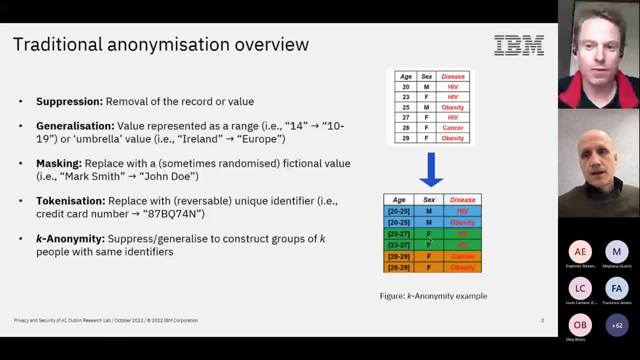 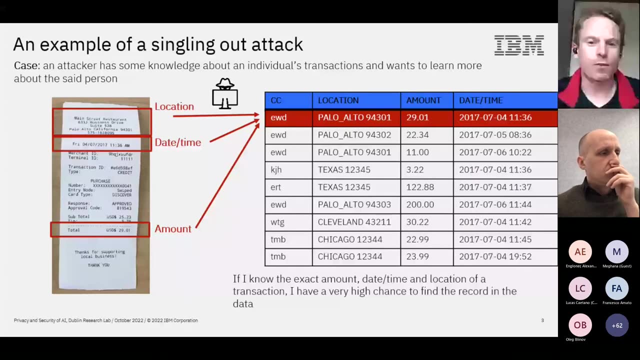 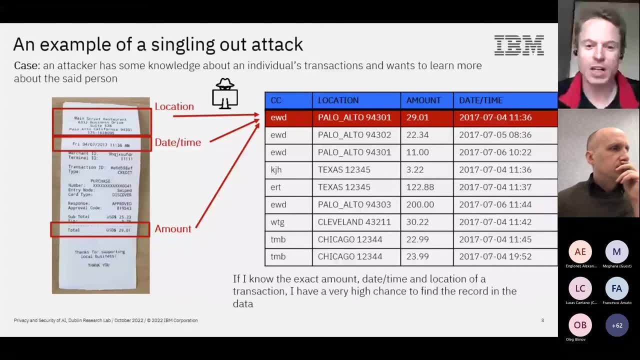 information about the location, the amount and the date and time, and we're going to anonymize in quotation marks by replacing the credit card number with a tokenization or tokenized value. now, this means if we had to have the credit card number or we know someone's credit card number. 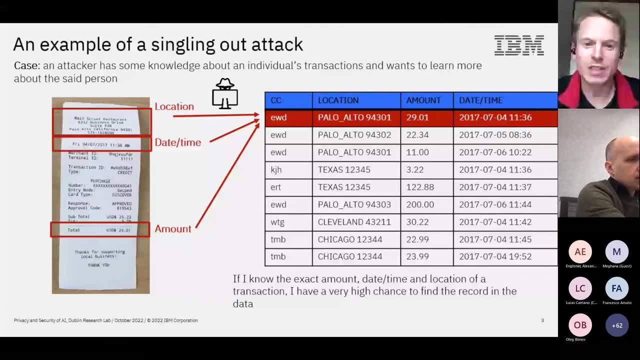 then we can't automatically go into the data set and find out what their transactions were over the last month. however, if we do have, if you manage to find a credit card receipt or something like that, then we can automatically go into the data set and find out what their transactions were over the 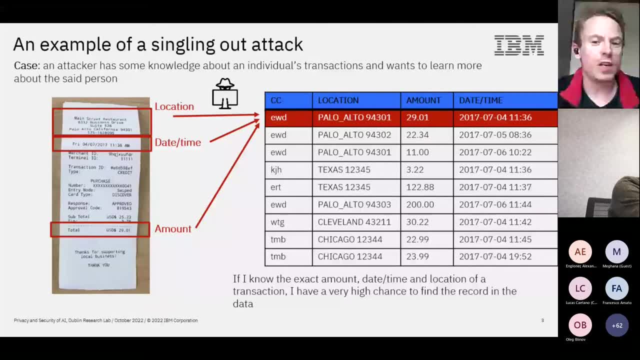 last month. however, if we do have, if you manage to find a credit card receipt or something like that, then we can use that to zone in on it, on that transaction in the data set. then we can uncover the tokenized credit card number and expose all of the transactions that have been um associated. 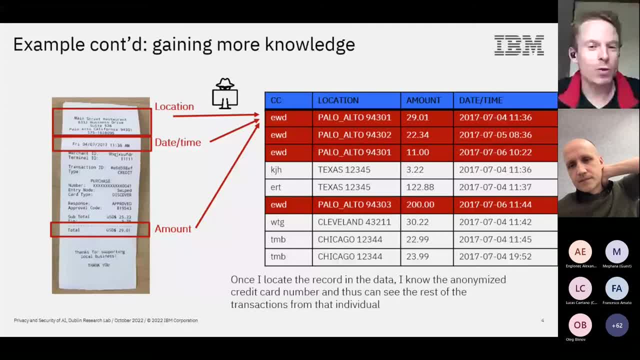 with that card. now you might say in this example: okay, what about if we, uh, change the amounts or, um, generalize them to the, the largest whole number, and do the same with the date and time, so remove the minutes or even the hours of the transaction? then you can say, okay, this attack wouldn't work. 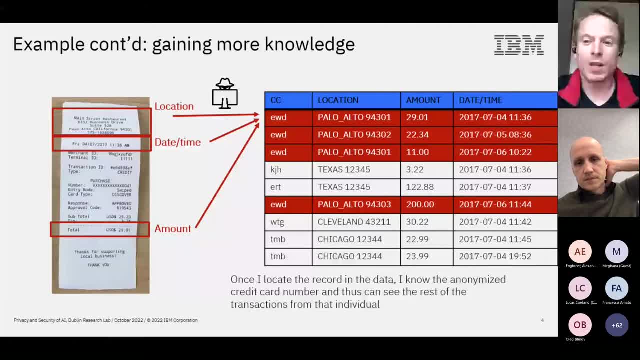 um, in that case you're correct, but um research has shown that doing those kind of generalizations, uh, limit the utility of the data but doesn't give you great protection, because if you have a second credit card receipt, for example, the uniqueness of those two uh transactions will. 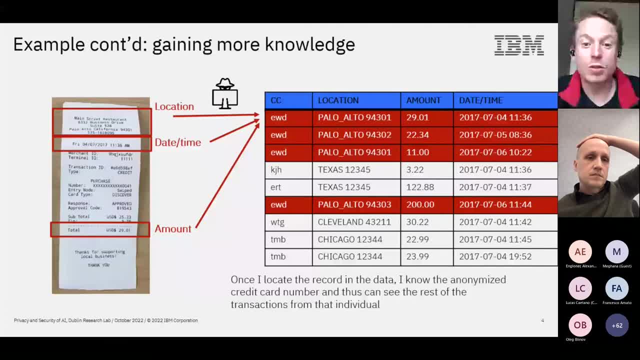 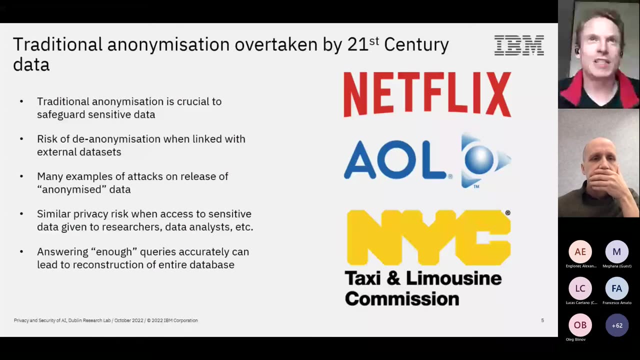 be enough to or could be enough to do to run this attack again. and i'm going to end then with, i guess, three more famous examples of um, of de-anonymization or anonymization gone wrong and attacked um in the wild and in in reality um. so the first of those examples is the netflix prize case, which 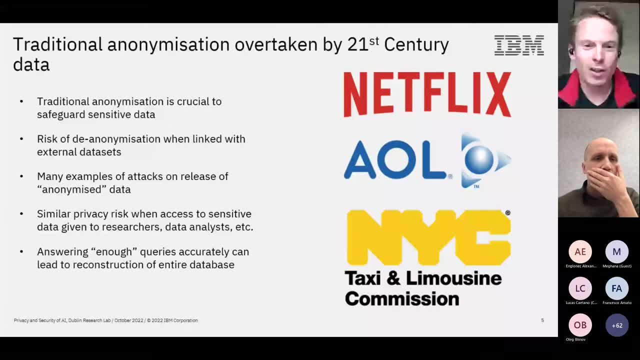 i'm sure the vast majority of people on this call will be familiar with, but i'll do a quick overview of it all the same. and so, back in 2006, netflix published a anonymized data set of um movie ratings in order to for researchers to improve their recommender. 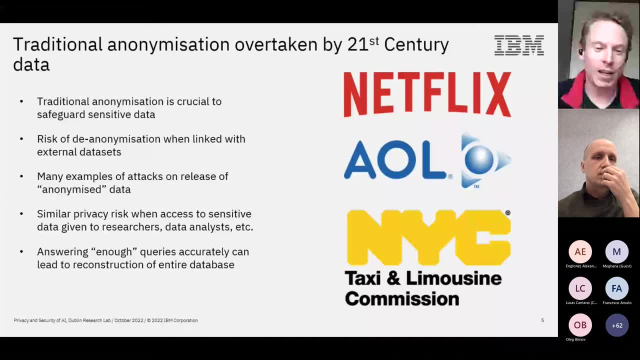 system and they had a cash prize for the for the best solution, and researchers were able to link it with the publicly available imdb and basically uncover individuals in the netflix data set. and you might think, okay, well what? what's the big uh deal with that? um, but if you could imagine that 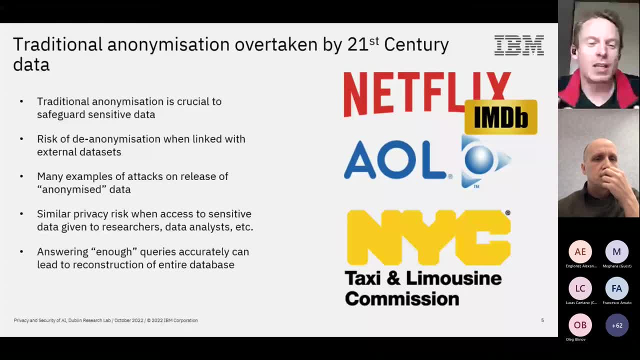 uh, you're probably giving a movie rate, movie ratings to netflix and you might think, okay, well, if you're going to give a movie rating to netflix in confidence, knowing that they're going to keep that data private, um, you might be a lot more willing to give uh ratings to sensitive movies. 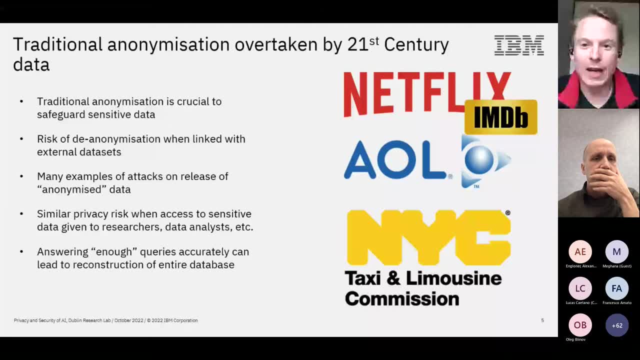 that you might be watching and it's this kind of an attack, then that linking you with a public data set out there in the wild and exposing the sensitive information that you've given in confidence to netflix, and this caused a lot of controversy within netflix um and culminated in 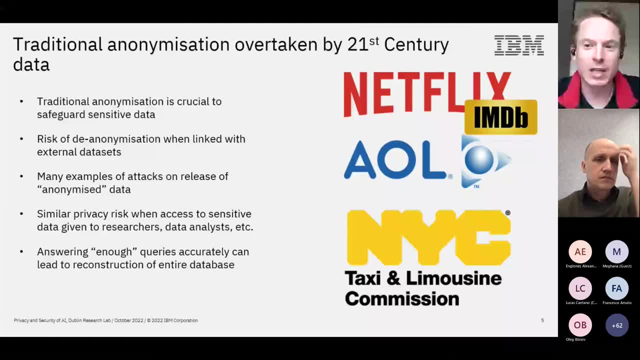 a second iteration of the of the competition of the netflix prize being cancelled. um aol uh put together a data set of an anonymous internet search logs and the real story is that uh netflix published a data set of anonymized internet search logs. and this is an interesting case because 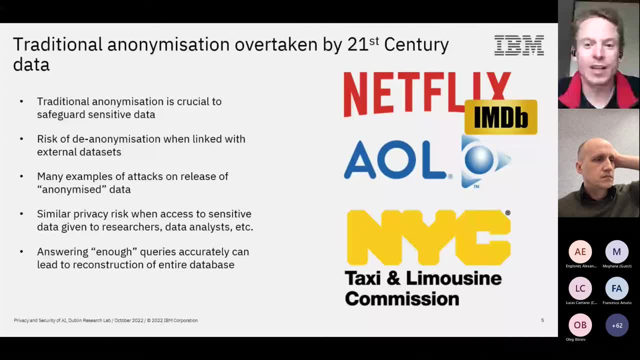 it's not actually an external data linkage attack that was conducted, but rather the data itself was rich enough and that the anonymization process itself wasn't sufficient to preserve privacy, and the new york times had journalists who dug into the data and were able to um expose an individual at. 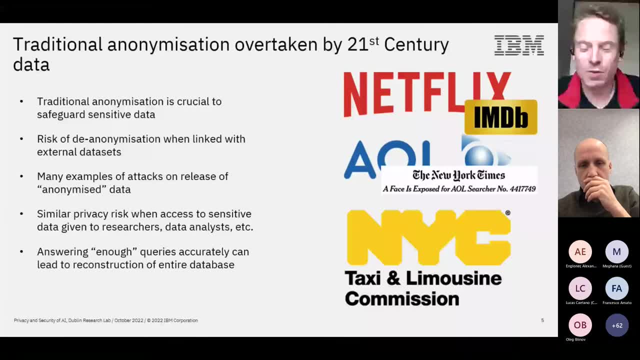 that data set and, i think, called to her home and gave her, gave her a printout of her um, her fucking over internet searches- which would be quite scary for most of us, I'd imagine- And to give you an idea of how you'd run an attack like that, 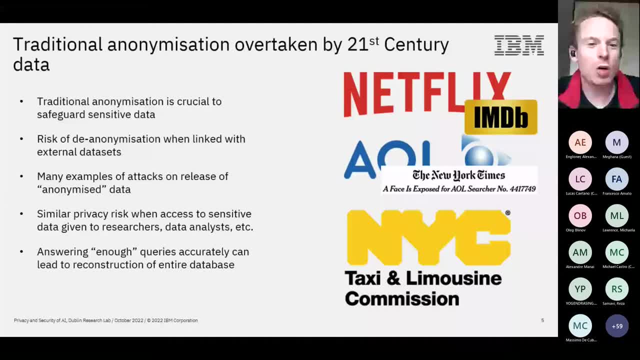 I'm sure everybody on this call has searched their own name in Google or your favorite search engine in the recent past, And I would suggest, I would wager, that you've searched your own name far more than anybody else on the planet, So it's these kinds of keys that you have. 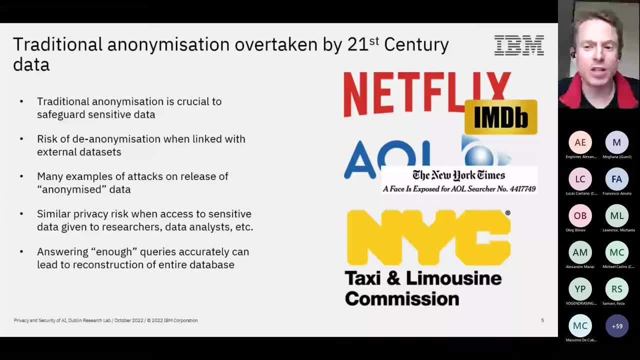 to very rich micro data that you can use to expose sensitivities when anonymization isn't done right. And the last example I have is more of a fun kind of example, I guess, involving the New York City Taxi and Limousine Commission. 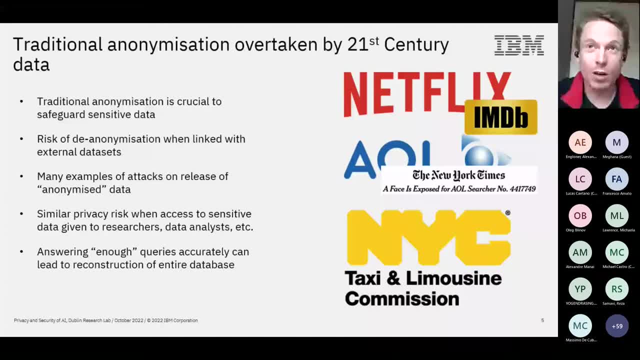 So they published a data set of anonymized taxi trip records in New York City and a blogger was able to de-anonymize it and, using photos on the internet, was actually able to single out taxi trip records in New York City and then use the trips that celebrities had taken. 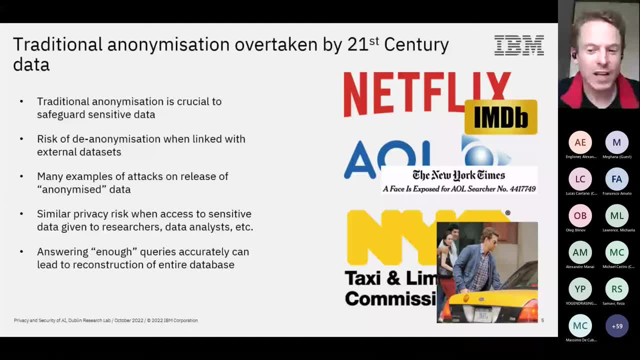 and find out the long laps of where they were traveling from and to and how much they were tipping the driver. So that's more of a, I guess, a more modern example of anonymization gone wrong, But in, I guess in a lot of these examples. 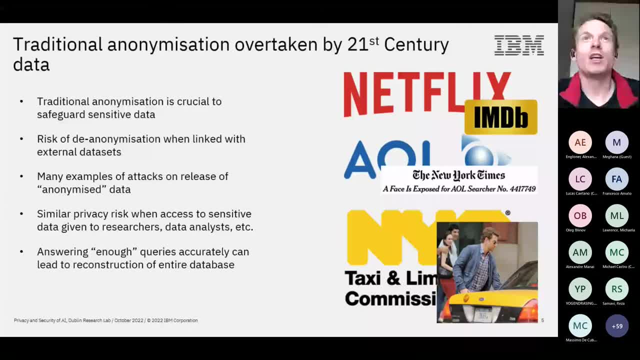 there were very small things that you could change to make the attacks that were implemented a lot more difficult, And I guess that sidestepping the point of privacy in general is actually quite difficult to achieve well, So these three examples were examples of data sets. 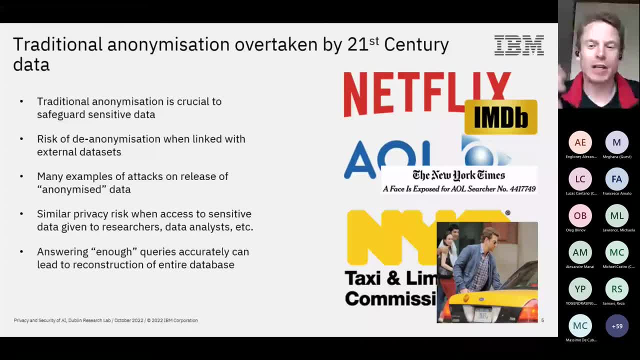 published in the wild and then subsequently attacked by some clever researchers or journalists. But we know that similar risks exist when you're giving access to data sets, for example for analysis, for� to just query. And there's this database reconstruction theorem that I'm going to paraphrase that says, if you allow enough: 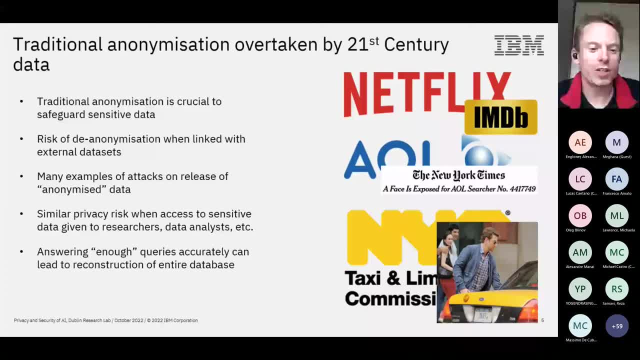 accurate queries to be executed on a data set, that then you can reconstruct that data set in its entirety. So it's very important that we think long and hard about the techniques we're going to use for privacy, as Frederico was talking about. He mentioned previously that we use all 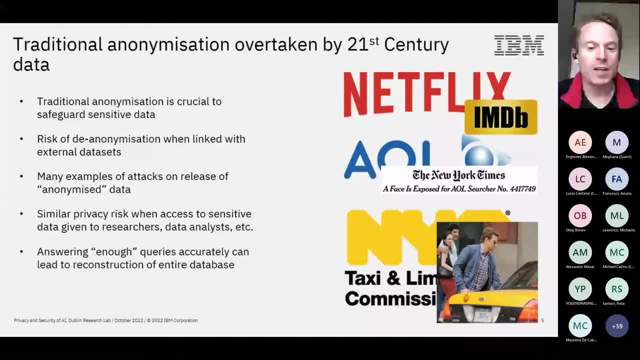 these techniques to manage risk and it's important to understand the limitations of the tools that we're using. So hopefully that will serve as a bit of a primer to, I guess, why differential privacy exists and why it was conceived as a result of all these failings of traditional. 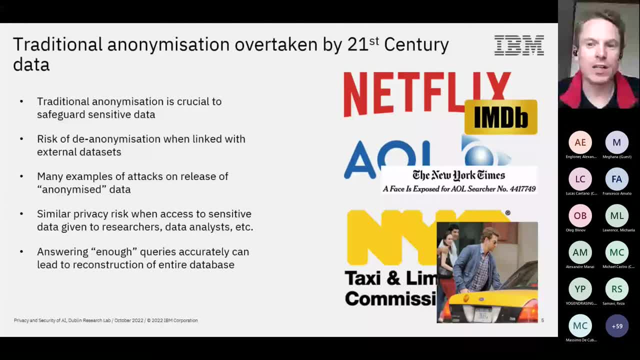 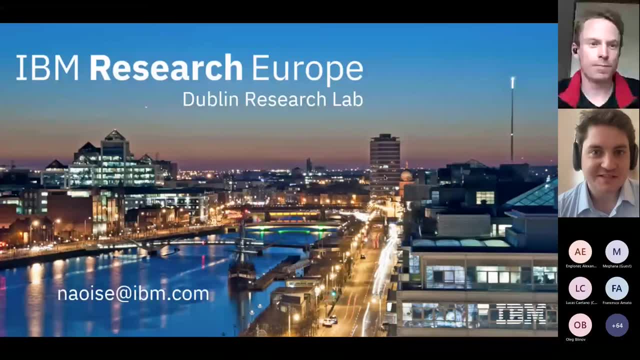 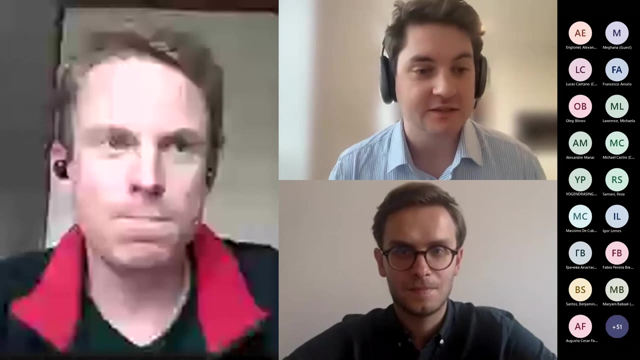 anonymization and I think I'll hand back to Jack now. Thanks very much. I think it really comes to light when you see the you know mess ups. I feel like none of these examples are people trying to maliciously share And expose sensitive data for some dubious gains. But even if they're you know, even if it's well, 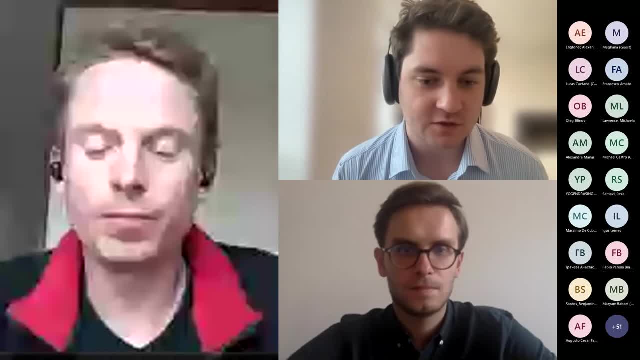 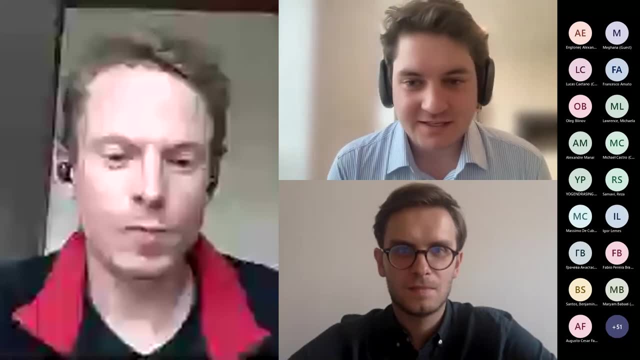 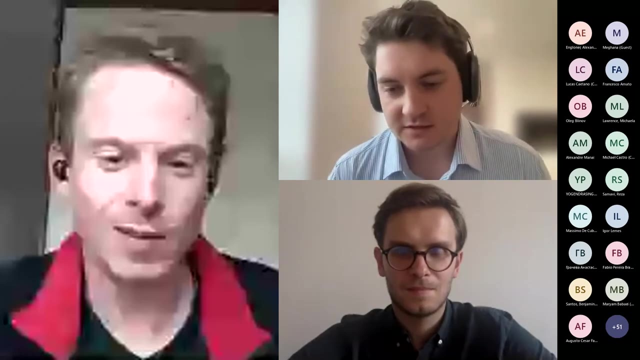 intended. often the information itself can actually cause more harm than good. So I see more questions coming in on this, so we're collecting them for the Q&A section, But we'll pass it over now to Robert Przarsic, who is the CEO of a company called Oblivious and that works on general input. 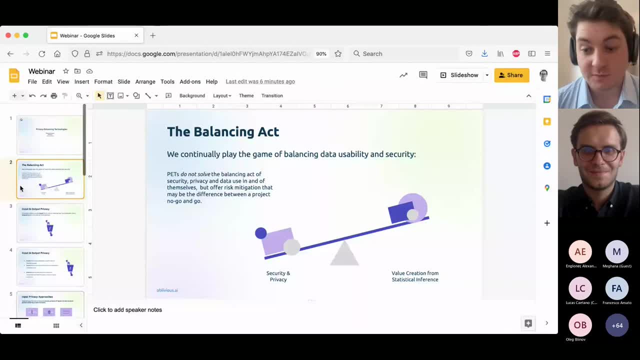 privacy, which I think he will explain very shortly, And he'll talk us through about the kind of landscape of privacy, enhancing technologies, not simply, you know, any of the kind of classical techniques or even just differential privacy, but actually giving a more holistic view of the landscape. So over to you, Rob. 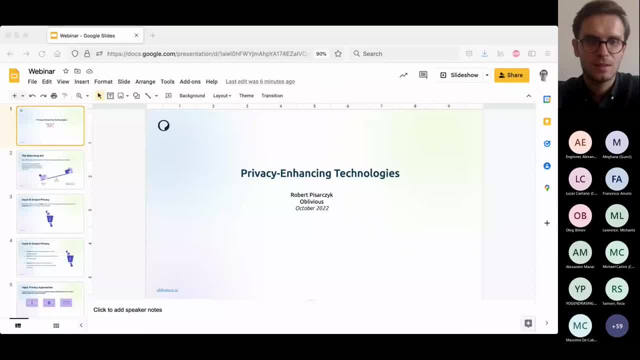 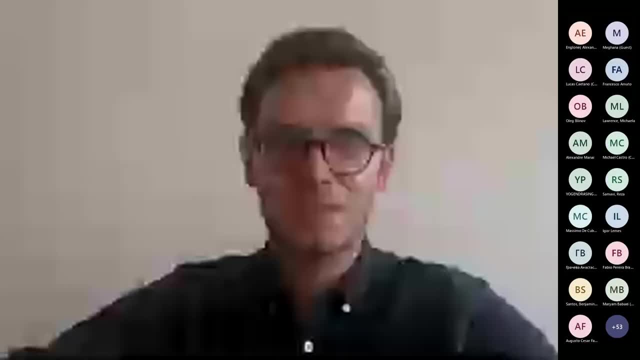 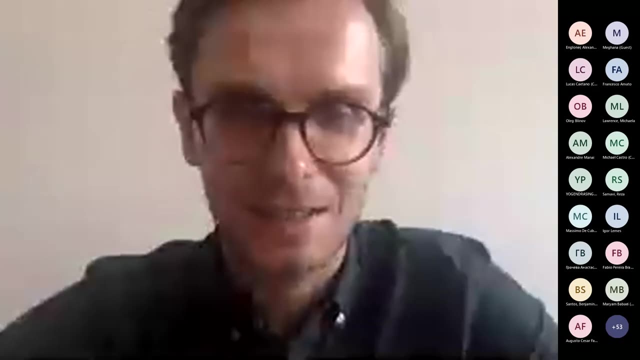 Thank you. Thank you, Jack, Can you see my screen? Just, We can, indeed. You're not in slideshow mode yet, though Is it now in slideshow mode? You are no longer sharing screen. Okay, Sorry, Maybe you can just share the whole screen, and that should work. 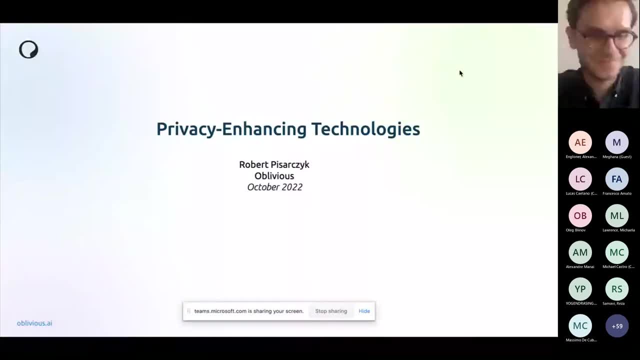 Is it working now? Perfect, You're in business now, Okay, Thank you. Thank you, Jack. Yeah, I think Nisha and Federica have done a fantastic job, really motivating why we need to care about privacy, especially when we're dealing with sensitive data, when anonymization can go wrong, that's one thing we have to do. And that's what we're doing now. Yeah, that's true. Yeah, it is. That's a great point. Yeah, I think some of the things that we're doing now, you know, we have to work with data and we have to work with privacy. 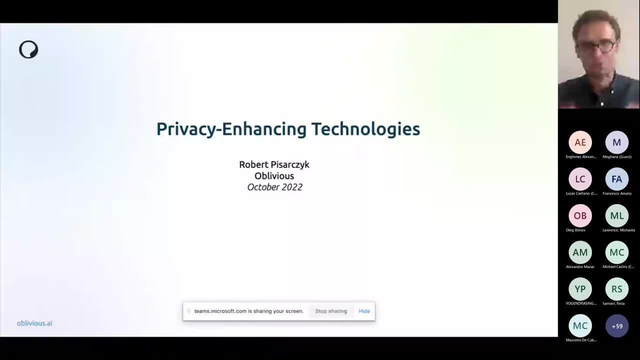 We have to work with privacy, We have to work with data and we have to work with privacy. We have to work with data and we have to work with privacy. anonymization can go wrong, So kind of, let's say some of the traditional techniques. 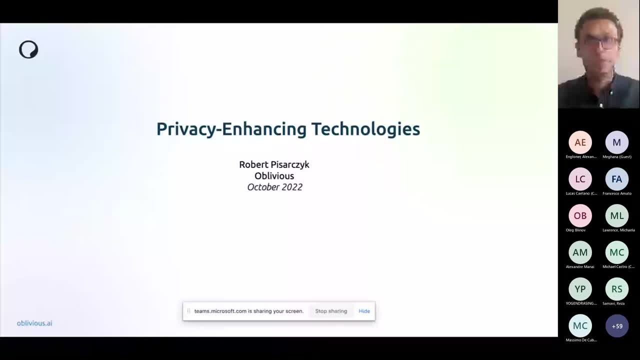 and therefore why we might need a new toolkit, and to think carefully about the toolkit that we're using when dealing with sensitive information. So, and that toolkit really really goes under- often goes under- the name of privacy and ASIC technologies. So the point of this kind of short presentation. 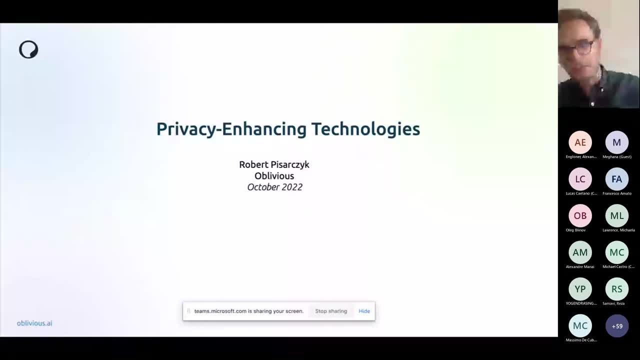 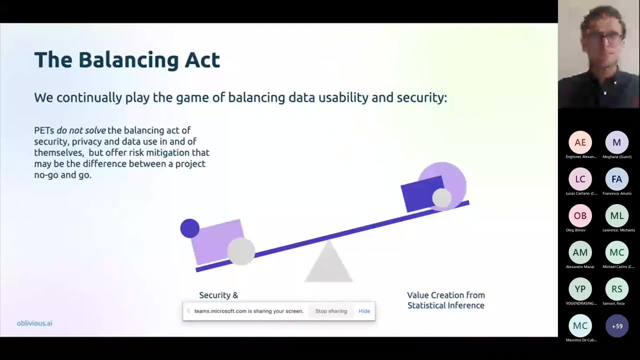 is to basically categorize those privacy and ASIC technologies and introduce some of them, especially the ones that will be part of the hackathon competition. So privacy and ASIC technologies are really about kind of this art and science of balancing data usability and privacy. And when you think about that, 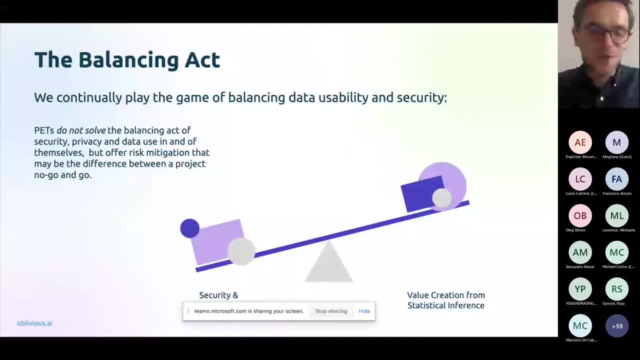 if you really want to make sure that your data stays private, you shouldn't collect them in the first place and never share them. But, of course, a lot of projects we do need to share them or we do need to process them. So privacy and ASIC technologies. 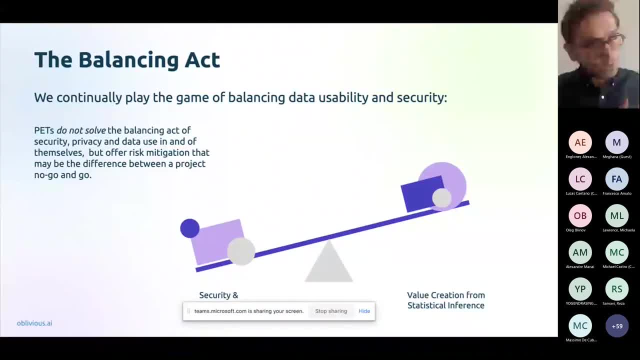 will not solve all of those issues for it when it comes to privacy, but they can offer risk mitigation that actually may be a difference between whether the project actually goes ahead or not and can really kind of tackle some of those risks associated with processing sensitive data. 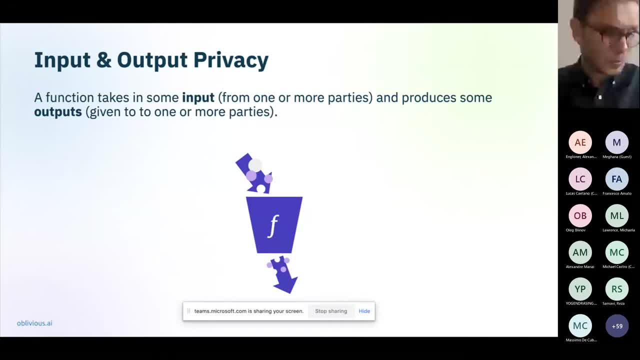 Very broadly and from high level. we'd like to categorize those. There's a lot of privacy and ASIC technologies and I've got Nisha mentioned differential privacy can have things like KK, anonymity and so on and so forth, but maybe let's put some order into it. 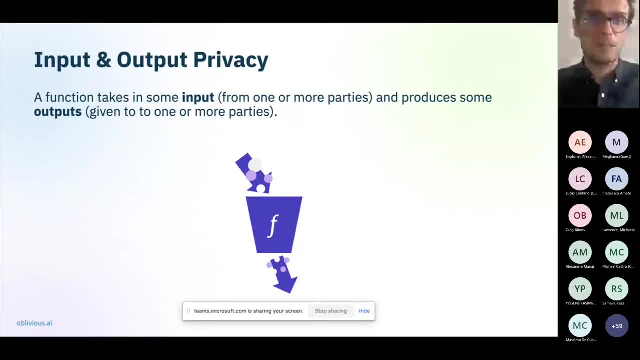 so we can categorize them as input and output privacy, And that really kind of follows what's like from a definition of a computation or a function. right, A function takes some input and then, or a computation and then it produces some output. 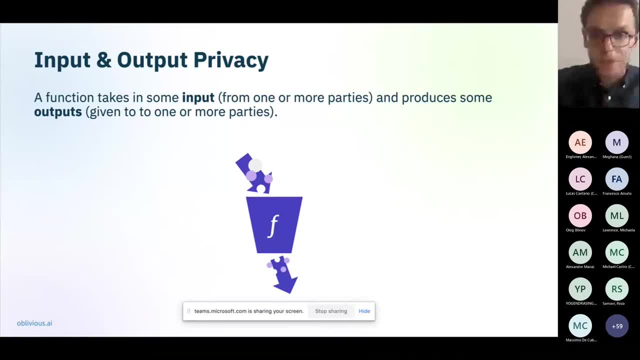 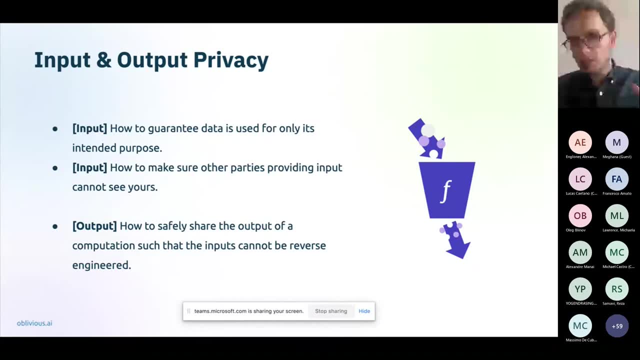 And that's really kind of also how input and output privacy come into this. So input privacy is really about how do we want to make sure that the inputs to the computation stay private, right? So if it's a very simple and they kind of 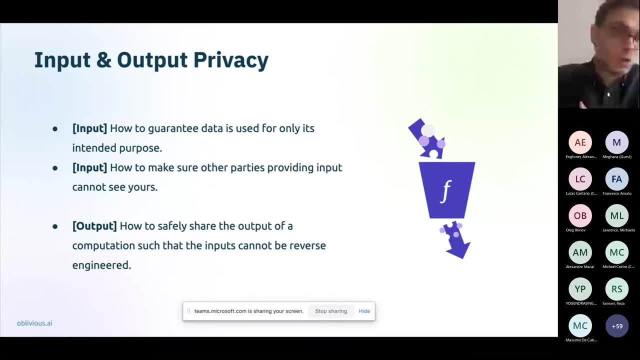 and they don't expose and they're not exposed to other parties taking part in the computation. A very simple example might be: we imagine Nisha and myself having each respective customer's list and we would like to find out, for example, how many joint customers we might have. 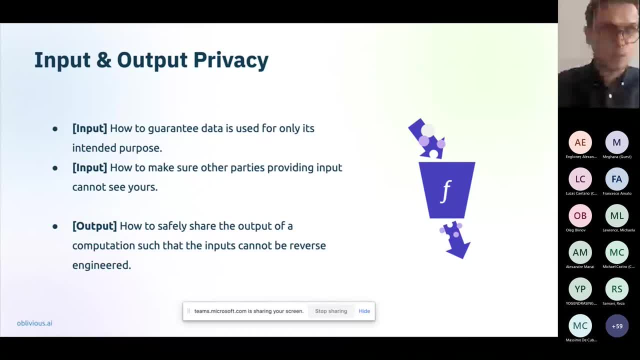 What we don't want to expose to each other during this computation is a whole list of customers, right? So we just want to find out how many joint customers we have. So that really is what an input privacy is about. Output privacy on the other side is really. 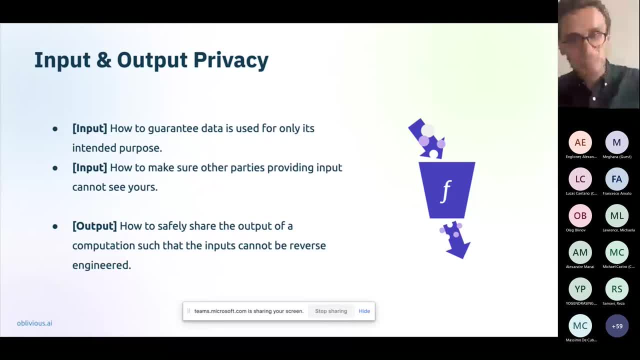 how do you want to make sure? how to make sure that from the output of the computation you cannot reverse engineer the inputs right? So when you're publishing different statistics, different aggregate statistics, like the number of joint customers, but it can be some demographics data and so on and so forth, 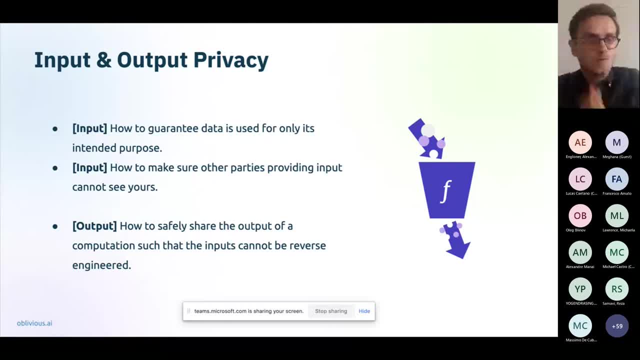 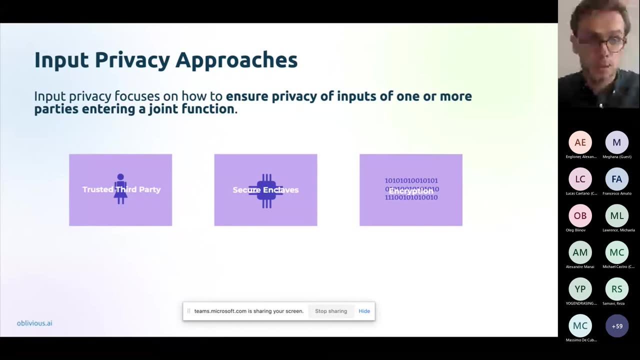 How do you make sure that from different data points you cannot reverse engineer the original inputs? So that's kind of the two categories, But of course you can achieve those in many different ways and there are different associated technologies When it comes to input privacy right. 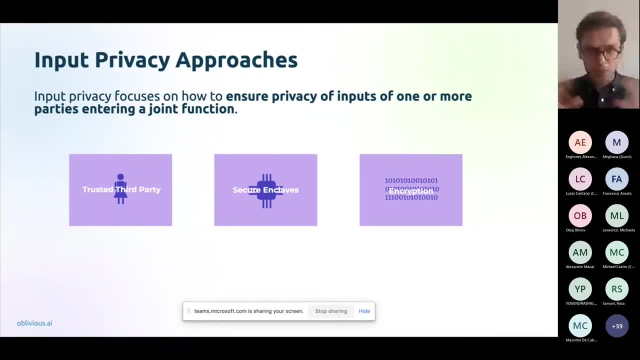 So those kind of ensuring that the inputs from different parties stay private during the computation, typically three ways to do that. The old way would be to give basically the inputs from different parties to a trusted third party. Now maybe it might be a international organization. 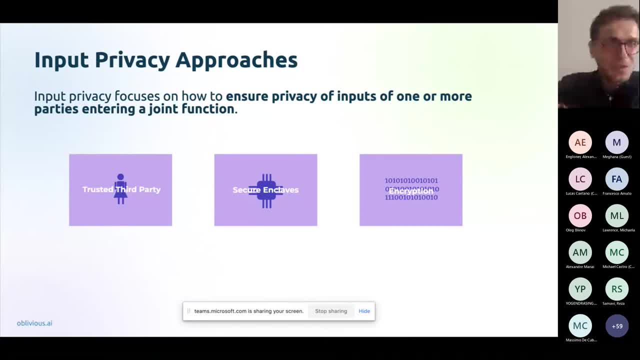 or it might be typically a consulting company, a law company that we all trust as parties, And then we can give them the inputs. They will process the data on our behalf and return the outputs to their respective parties. But of course, that's not all. 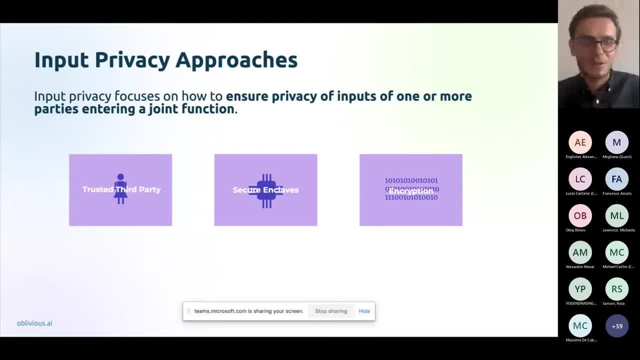 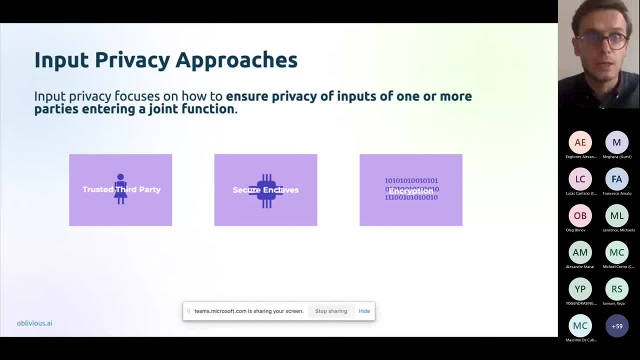 And then there are two other technological ways to ensure input privacy, and that's to do with secure enclaves and encryption based methods. So let me say a few more things about, a few more words about each of them. When it comes to encryption based methods, 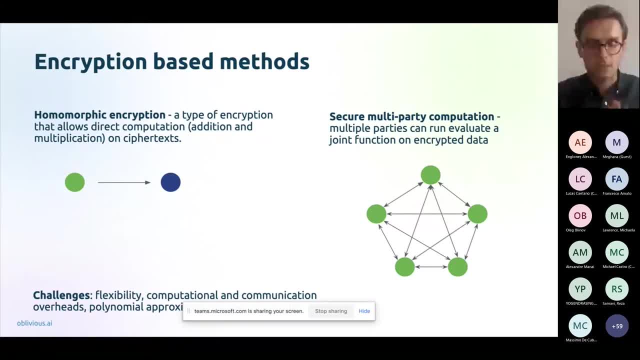 these are really the methods that kind of started in 1970s and have been the cornerstone of cryptography research for the last few decades. and what they're about is? they're about processing data and manipulating the data directly on ciphertext- right, so you encrypt the data and you and you can perform the. 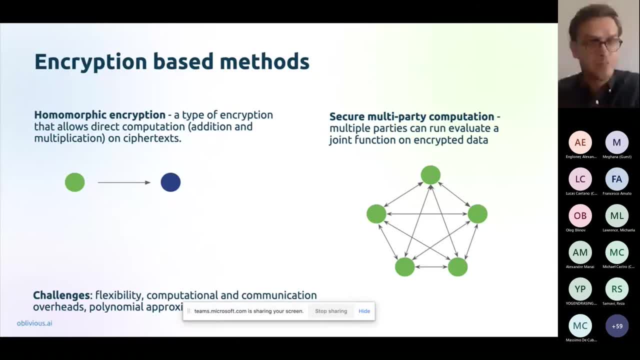 direct computation without ever decrypting that data so directly on software text. an example of that is homomorphic encryption, where you can, for example, you know, let's say, i have some data, i can encrypt them and i can send them. to send this encrypted data sets to external server and the server can add and multiply- uh, my data, and so perform. 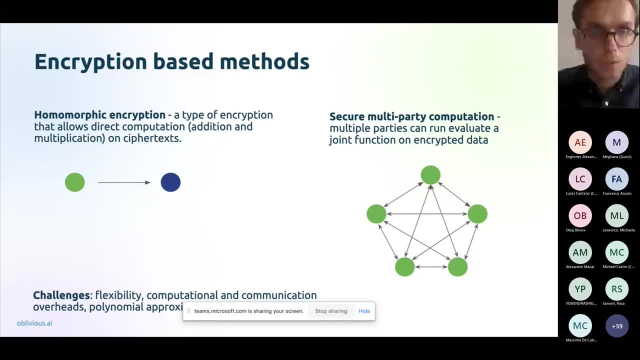 computation therefore perform any polynomial without ever decrypting these data sets, and that's really kind of. all was like part of a of the whole field of kind of secure multi-party computation. but you can have two or more parties, um, that can evaluate joint function on encrypted 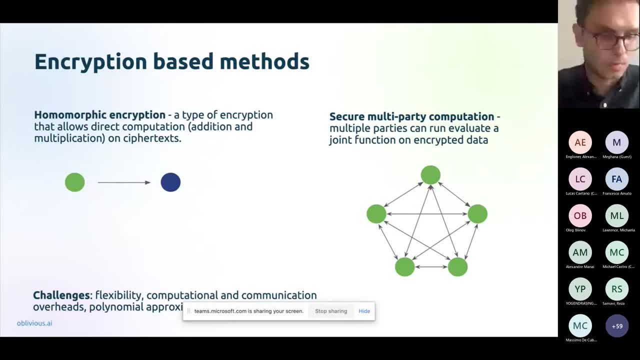 data sets, so not just um, you know, uh, delegating uh computation to an external server, and that's really composed of many different cryptographic primitives. uh, one of them is, for example, like secret sharing, where each party can almost like split their inputs between uh many different parties, such that no single party can learn anything about that input, and only if you. 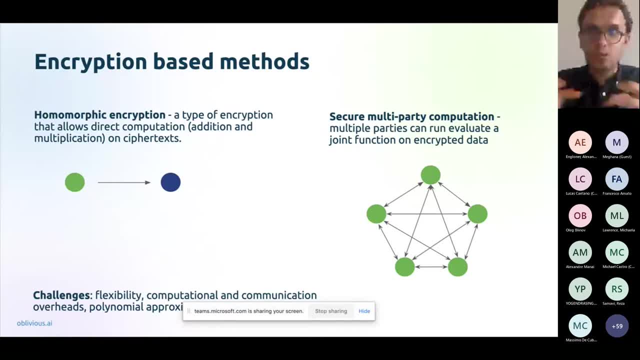 aggregate the kind of this, the shares from different parties. you can recover the inputs, right, but no single parties could do that. and there are other um techniques and and cryptographic kind of primitive protocols, uh, that's that form different protocols around secure multi-party computation. they're- they're, of course, a great premise, right, so you? 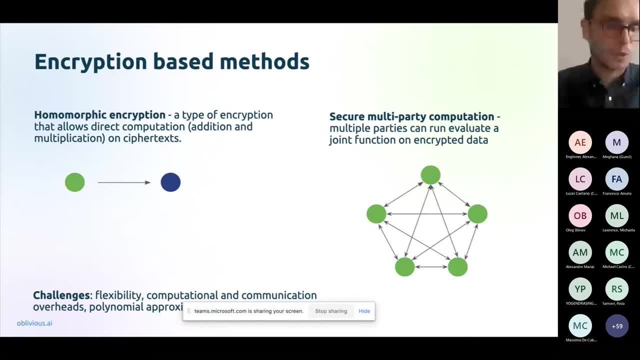 can always uh perform computation directly on encrypted data. however, there are some associated challenges, and that that really applies to each technique that we will always be describing here. right? so there are some great things about them, but you always need to be also careful about some of the associated challenges or risks. uh with encryption based. 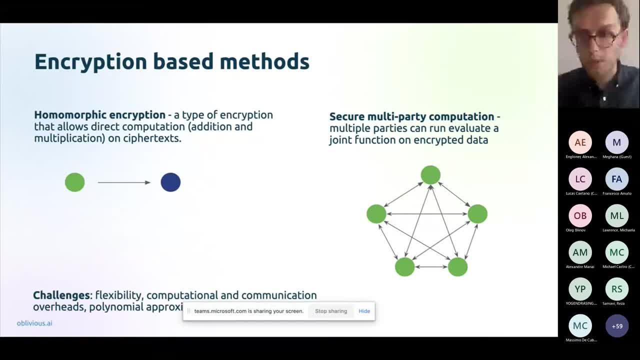 method. you often have a very large computational and communication overheads so they can be painfully slow, um, from what the encryption is doing, for example polynumerary approximations, um and especially when you're talking about um kind of production, um deployments. there might also be challenges associated with the lack of standardization, for example when it comes to some 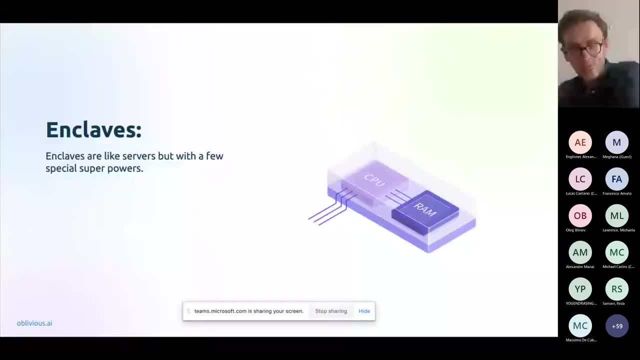 of those um techniques. um, so the second way to achieve um input privacy is through something called secure enclaves, or so some- because trusted execution environments or confidential computing- different names but essentially same things. um, and enclaves are really like a normal server, but with a couple of uh. 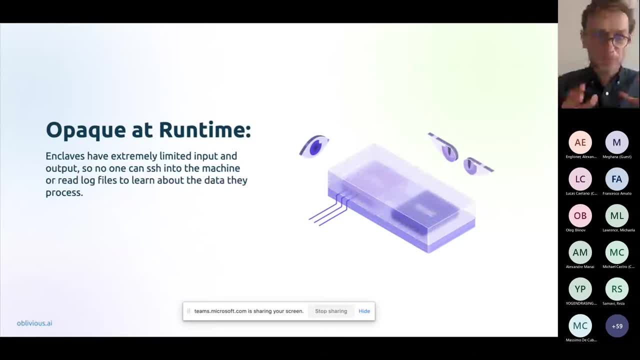 special superpowers? um so firstly, enclaves have they basically isolated from the rest of the computing environment and they have very limited input and output, right? so nobody, even like a system administrator, cannot ssh or look into the machine, read log files or see, you know, the data. 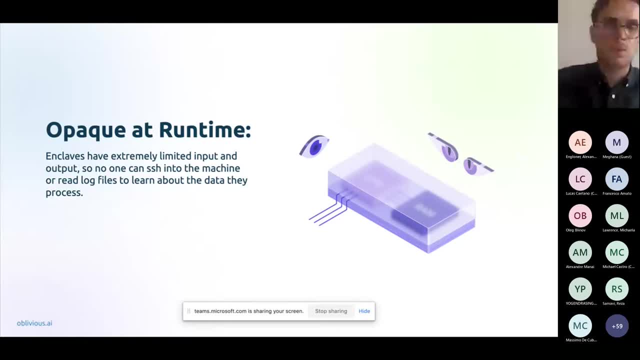 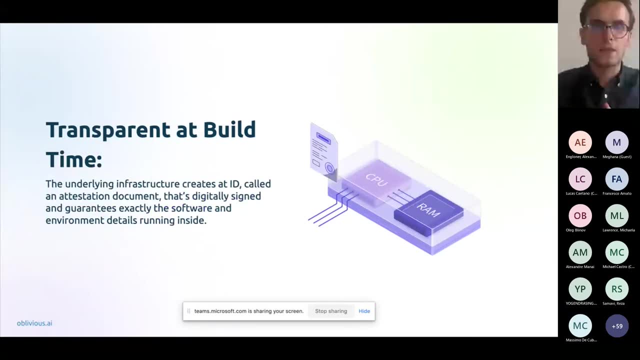 that that are being processed inside of the enclave. and the second property is that the underlying infrastructure, um, can issue something called cryptographic attestation document. it's essentially like an id that basically guarantees the software and the code and all the environment variables um around it, the being of the code that's run inside of the enclave. right so you? 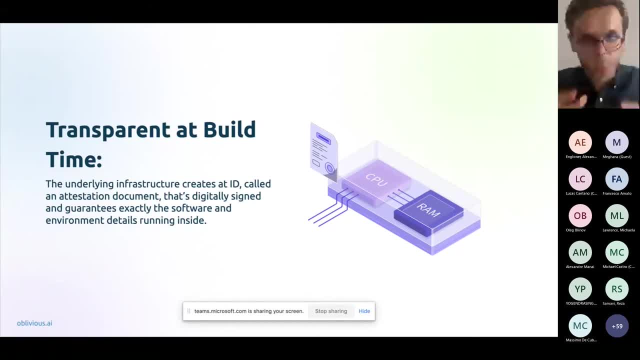 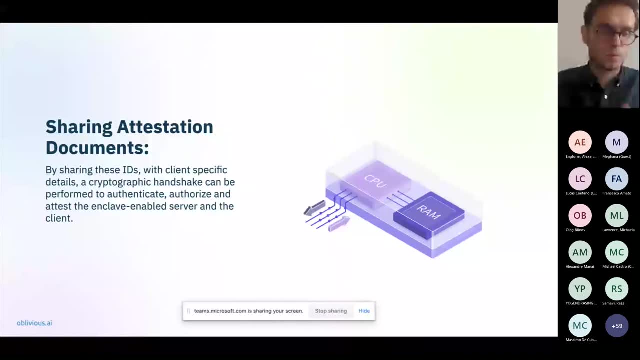 guarantee strict guarantees about what's being run inside and you have this isolation and through the attestation document, you can- you can use that to to establish a secure connection with the enclave right, so you can make sure that you have authenticated and authorized users that can communicate with the enclaves um and and through that you can attest, basically, the server. so this: 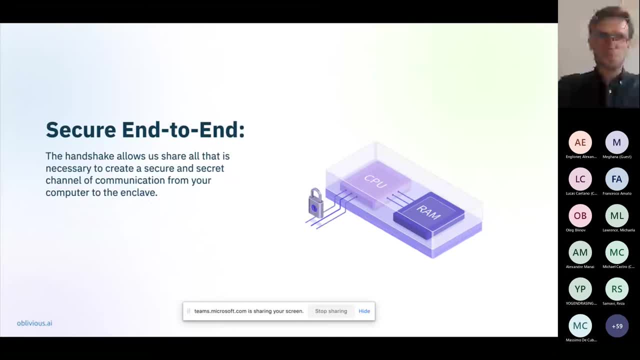 enclave enabled server and that gives you, you know, secure end-to-end connection to enclaves such that you can, you know, send encrypted data and these data will- and only authorized parties can do that- to the enclave, and these data will be decrypted within the enclave to run specific pre-approved application. um, so enclaves are now. 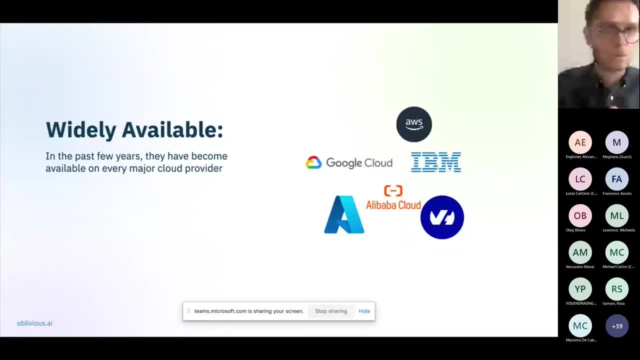 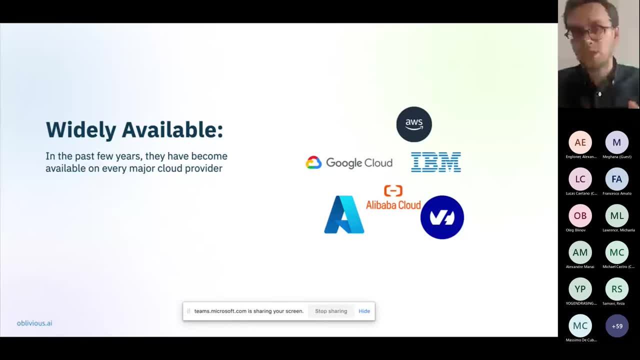 trust other hardware provider or you need to trust particular uh clouds. when it comes to enclaves, and there are also ways that you know you can, in principle, attack them, so you need to think about things like side channel attacks or timing attacks when designing applications to be run within. 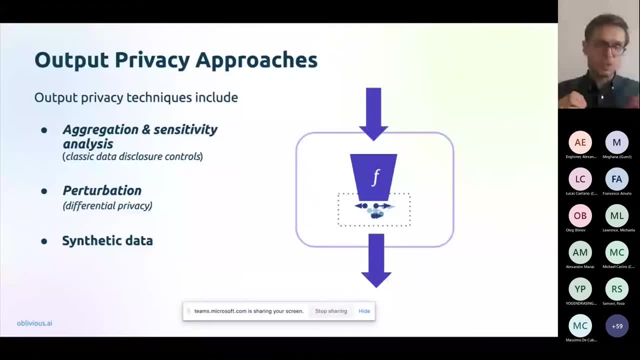 enclaves. um now turning into output privacy. um, so output privacy. yet again, there are different techniques that can be uh used to achieve output privacy. right sort of how to make, how to make sure that from the outputs of the computation, you cannot reverse engineer the inputs? um, as federico was saying there. um, of course, statistical data disclosure controls. 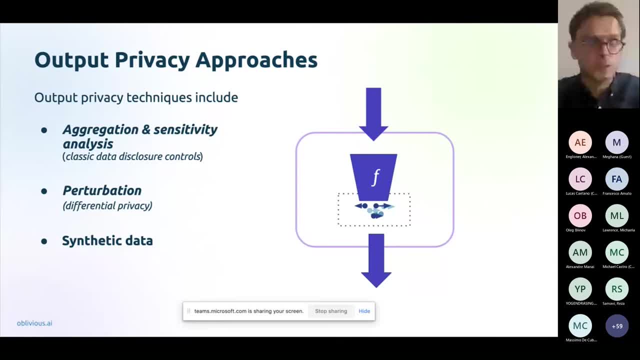 from different anonymization techniques like uh k anonymity- uh, to you know, aggregation and sensitivity analysis. it's like very careful analysis how you're going to disseminate your data. um, there are also some more recent techniques, like differential privacy, and i think james um is going to talk in far more detail about this, so i won't spend too much time on it. but 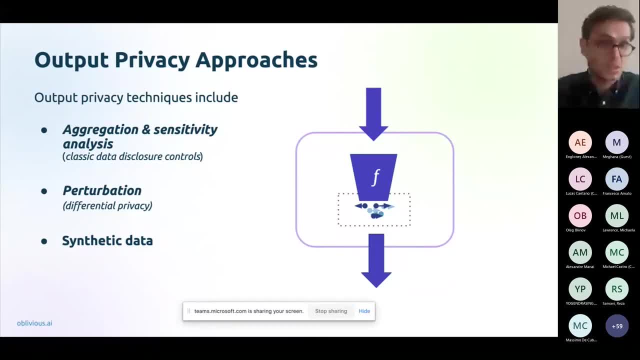 essentially it's. it's a mathematical differential privacy is mathematical definition of output privacy, um, and it can be affected, and it's most uh often uh effected- through, essentially, perturbation of the output, so adding appropriate level of noise to the output such that it guarantees that you cannot say anything about the individuals and the underlying. 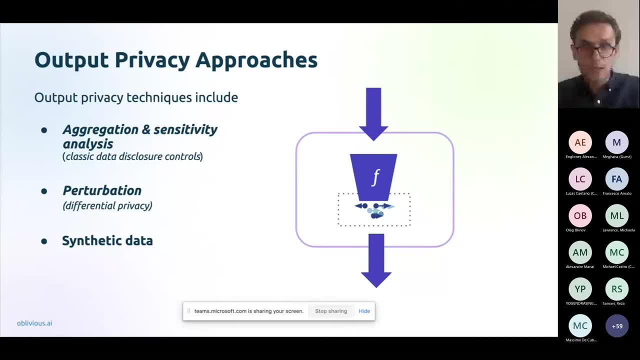 uh data set um synthetic data is, yes, another um kind of prime output privacy technique. um, and it really is about creating a fake data set that mimics the original uh data set, like through correlations or um you know uh, particular uh sensitive statistical properties, without actually having any of the sensitive um underlying uh you know uh, for example, personally identifiable. 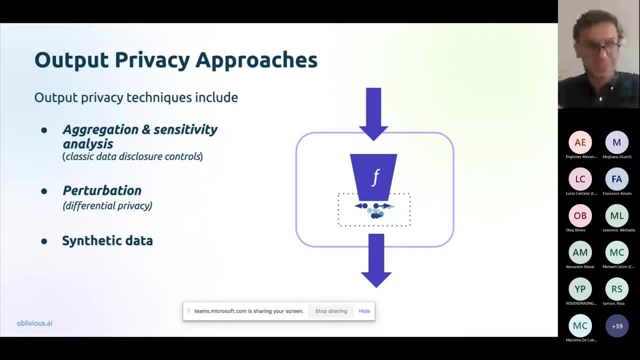 uh information, um synthetic data, can yet again have differential privacy guarantees, and i think we can. we'll also be talking about that where you have those mathematical guarantees about, about output privacy. so that really is kind of really after the whole um ecosystem of uh, of of privacy and seek technologies, and i think the exciting part about this hackathon is that. 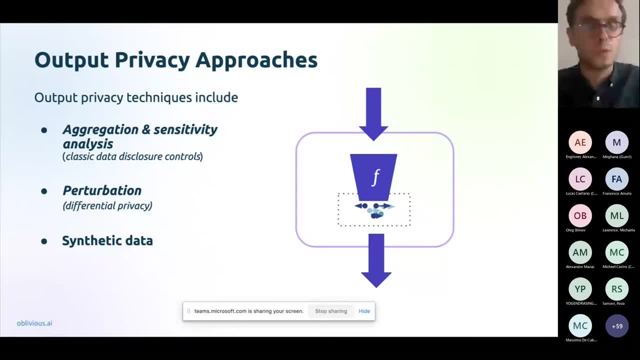 that both input privacy and output privacy techniques will be part of it. so in particular, secure enclaves and differential privacy and different private synthetic data will form will be used in that hackathon. so if there are any questions, again happy to answer them at the end of the q a session. thank you. 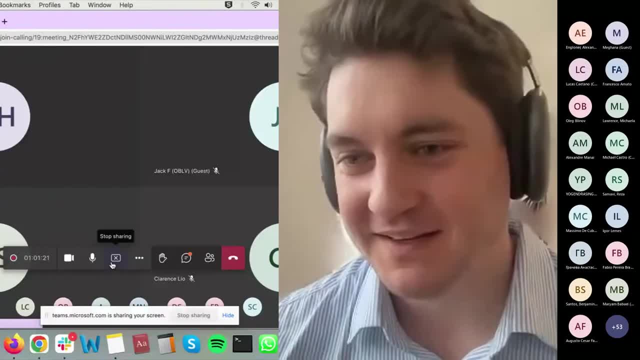 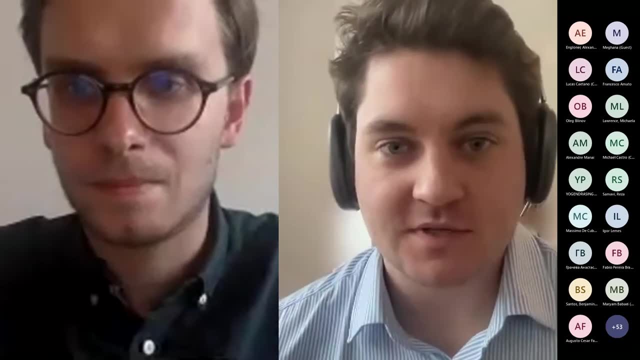 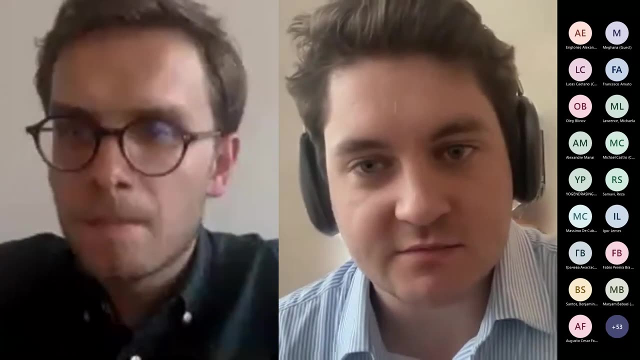 great. thank you, rob. so i see more questions coming in, so, um, i'll copy these into into the thing for the q a at the end. but now we can pass over to james honaker. so james is the chief privacy engineer of open dp um and a research scientist in the statistics of privacy group at meta. 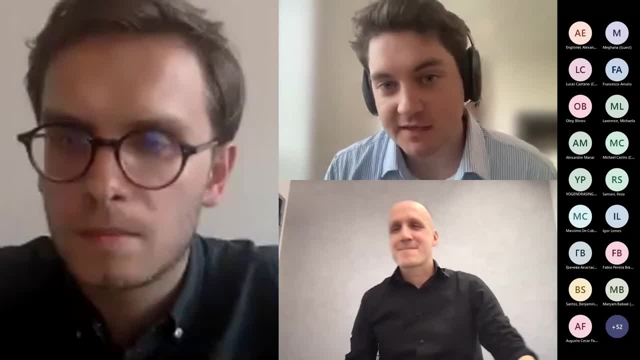 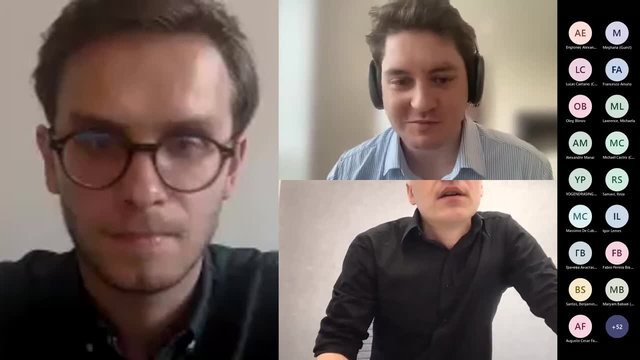 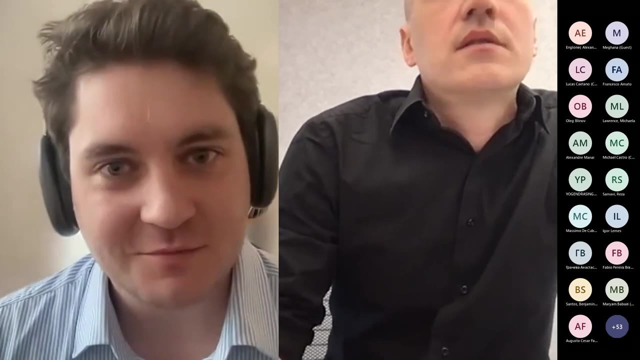 where he works on differential privacy applications at scale at meta's advertising models, and he's very well known in the space and it's probably one of the most appropriate people to introduce differential privacy to the group, so we're delighted to have you. thanks very much, james, and i'll pass it over to you. 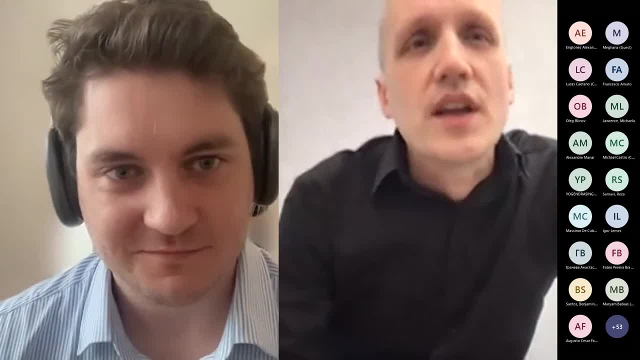 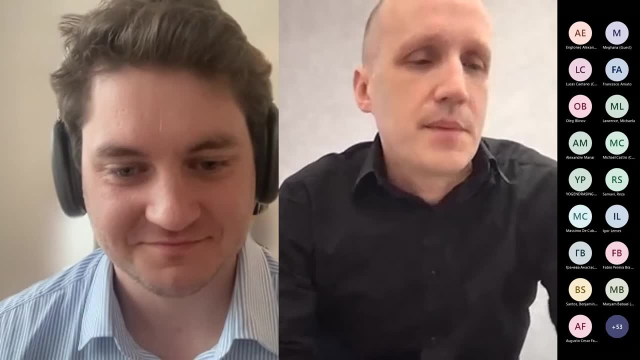 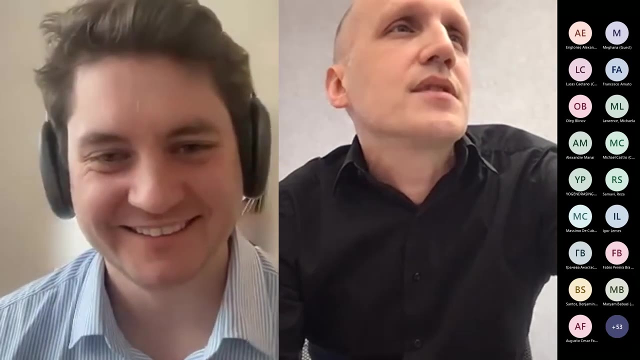 lovely. thank you. um, i'm attempting to share. let's see if we can do. might be confused by having multiple screens. your computer is too private, it's not willing to absolutely like like differential. privacy is not just a you know, it's just not just a mathematical theorem, it's a way of life. 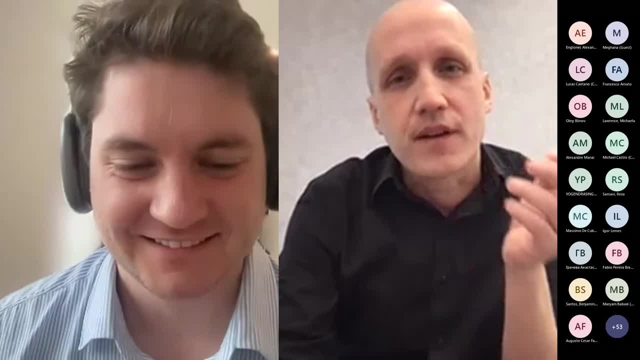 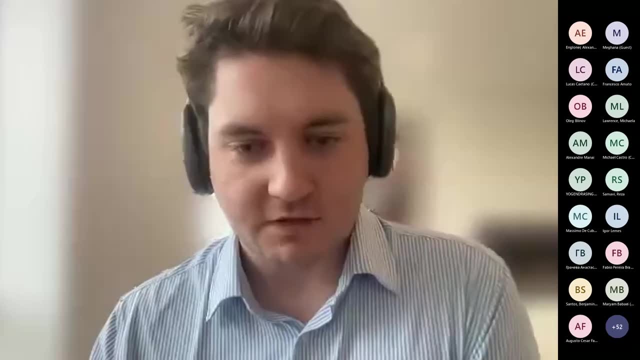 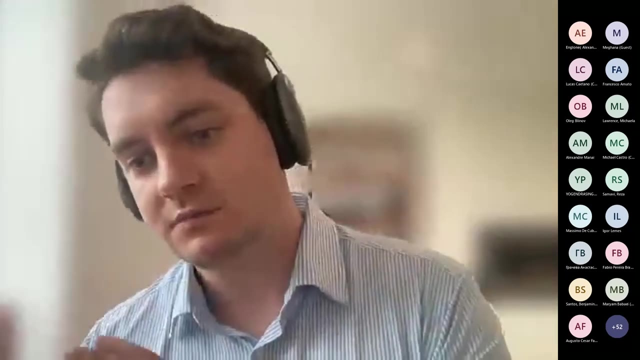 um so uh, let me see. if i unplug my machine, maybe i will have a little more luck, maybe as a useful um, i think we can do for the time being is we actually got some some questions in, so instead of leaving them to the q a at the end, 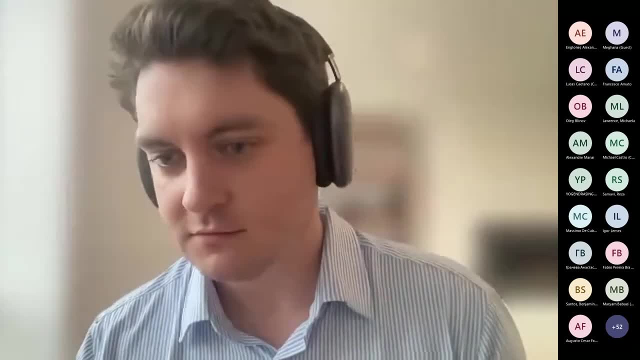 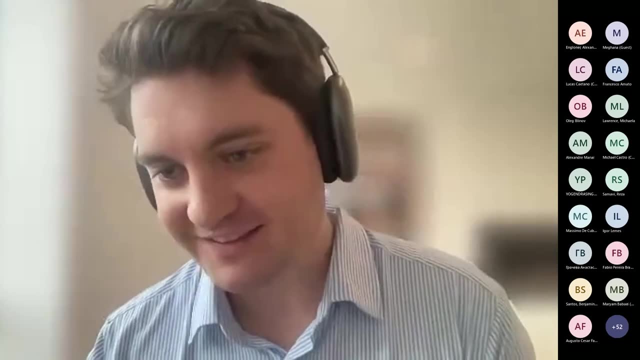 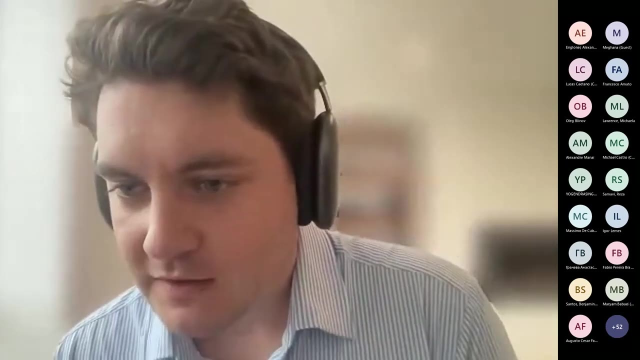 um, if james needs a few minutes, i guess we can probably go through some of these in the meantime. so these are in no particular order because they're kind of copied um at different points. so we'll get through all of them. and but so matt weldon asked: are there quantum safe? 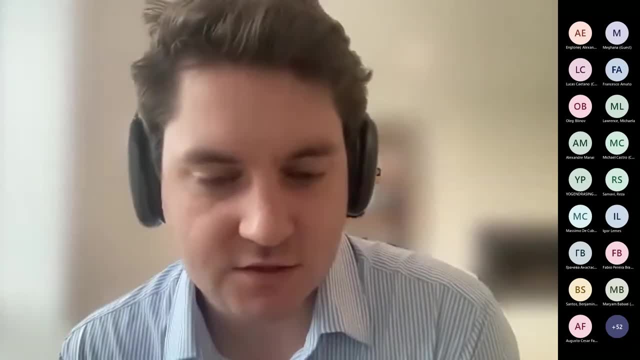 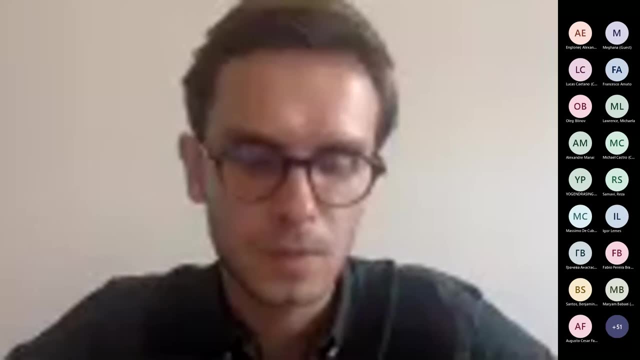 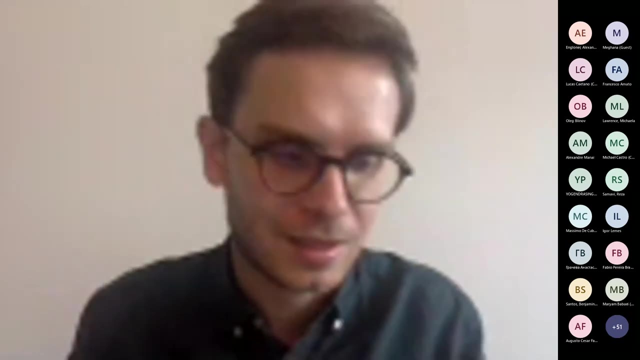 homomorphic encryption methods. so, rob, maybe your best place to to answer that um. so yes, um, in a sense that, um, there are post quantum, so we have this. you know all this kind of cryptography primitives like rsa and dickie hallman and so on, that, uh, i believe i mean that. 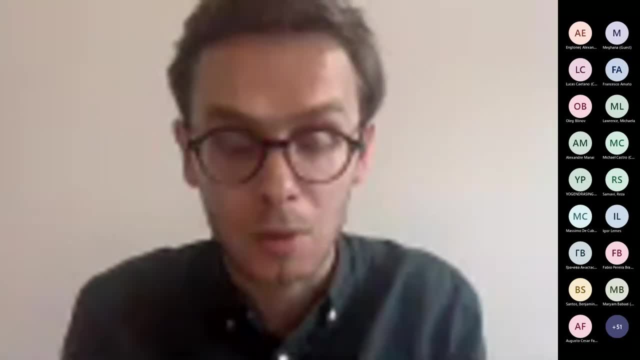 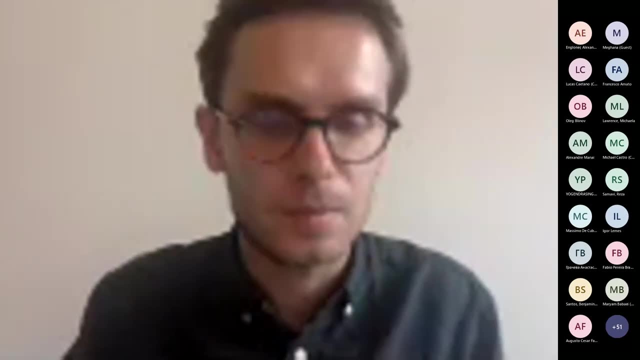 we have basically an algorithm that they could. if we have a quantum on a quantum computer, that can hack it in a polynomial time, right. so they are not quantum resistant. and there are those other protocols, um so-called post quantum uh cryptography protocols that are believed to be secure against 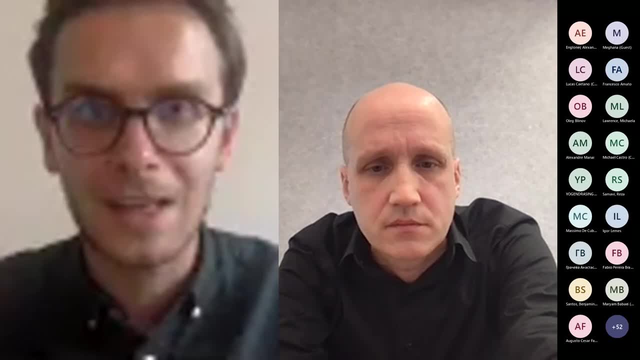 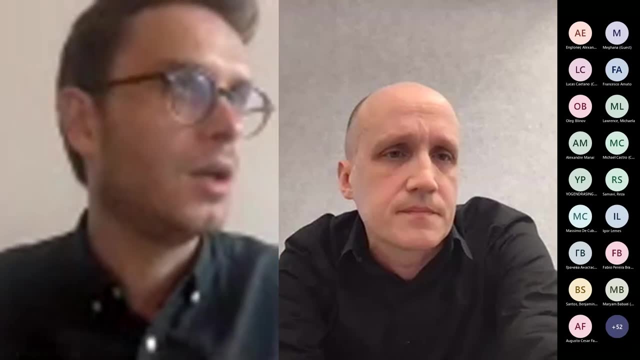 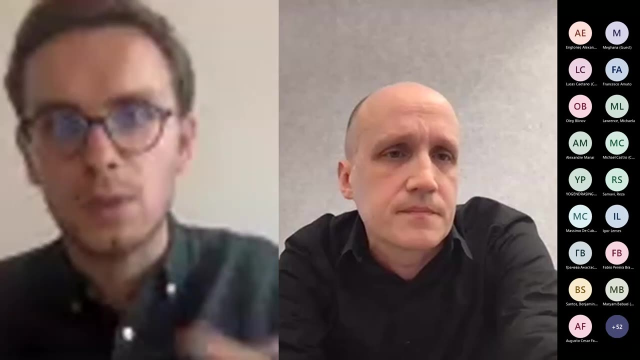 quantum computers, and those are, for example, based on lattice-based cryptography, um, and most of the fully homomorphic encryption scheme in use, like uh tori fully homomorphic encryption scheme and so on. they're based on lattice-based cryptography, um and, as such, are believed to be secure against. 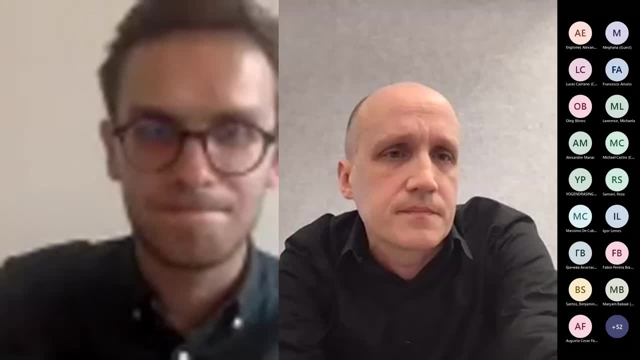 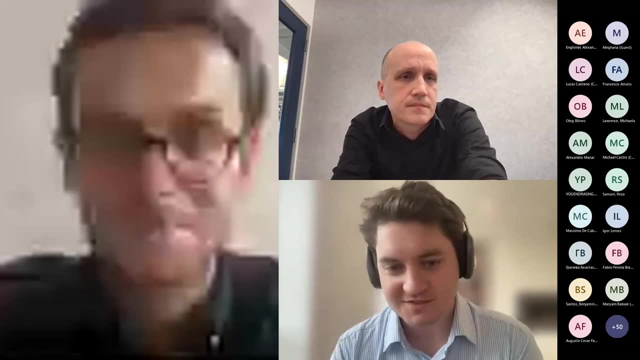 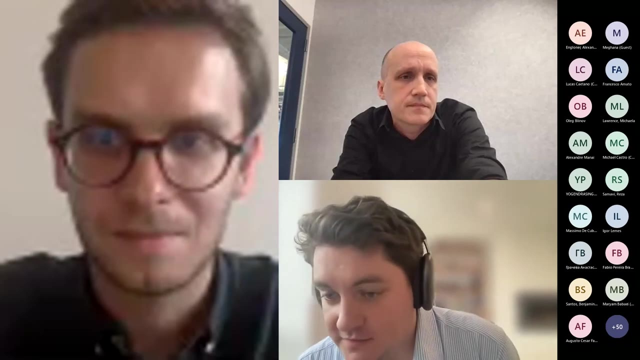 quantum computer attacks and asset. now, all right, thanks. thanks, rob, we can keep fielding questions. and james, hopefully you can give us a thumbs up when you're, when you're good to go. so, and sakanya asked our enclaves, sorry, our enclaves. uh, hardware or software can be run on your local machine. does it require? 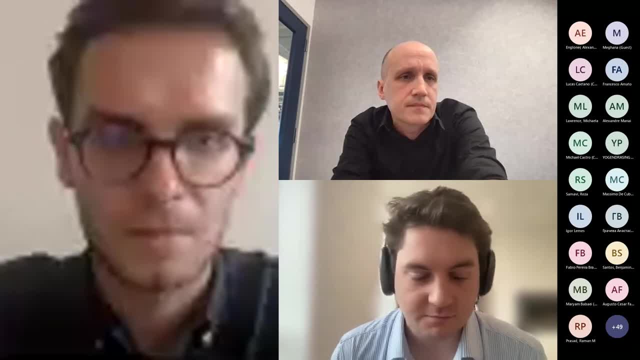 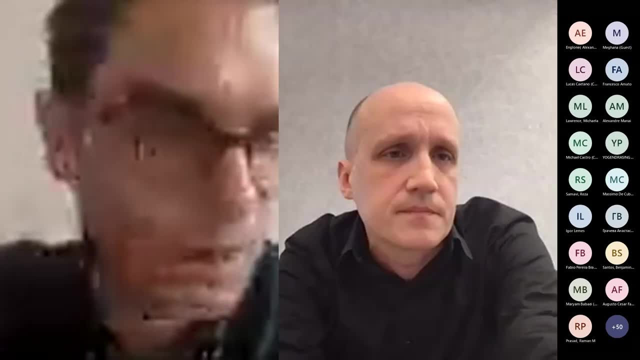 purchase of specific equipments, et cetera, et cetera, and so pass that back over to you, absolutely. um. so when it comes to enclaves, they're both like hardware based enclaves, so actually almost like the story of on-plate starts with intel sgx in 2014, uh, where they roll out a separate piece of silicon. 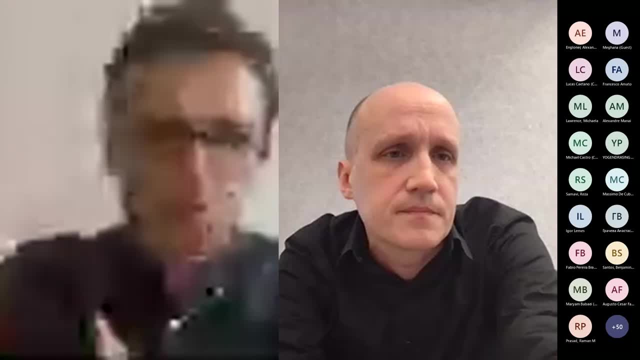 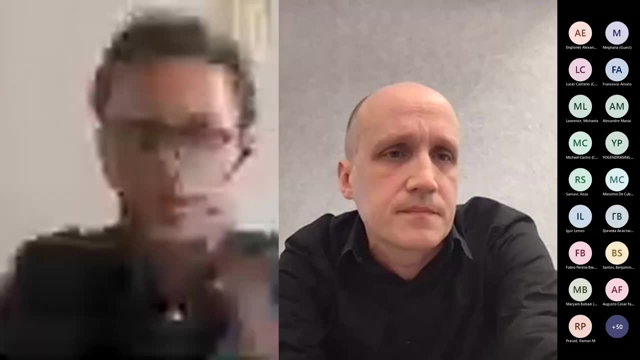 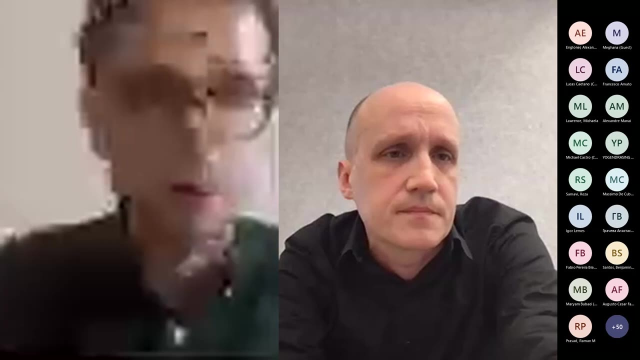 um and that uh, that had kind of two properties: um, right kind of isolation, and it could attest the software that's being run inside um, and it could, of course, buy the physical chips. now they're also actually like software sort of enclaves, uh, minnesotans kind of hypervisor based on it. so 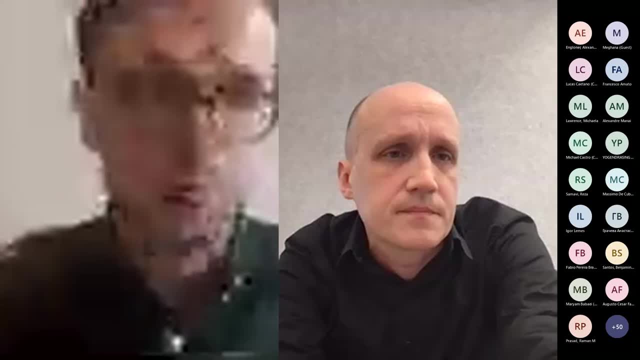 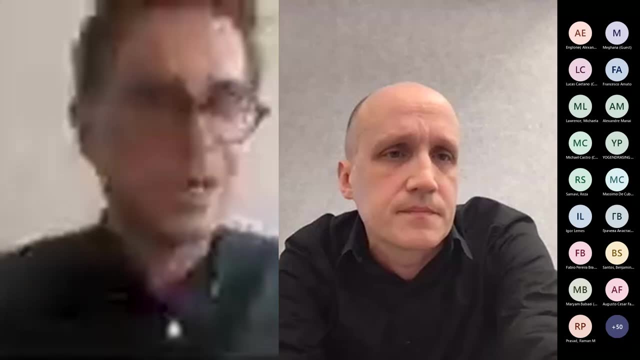 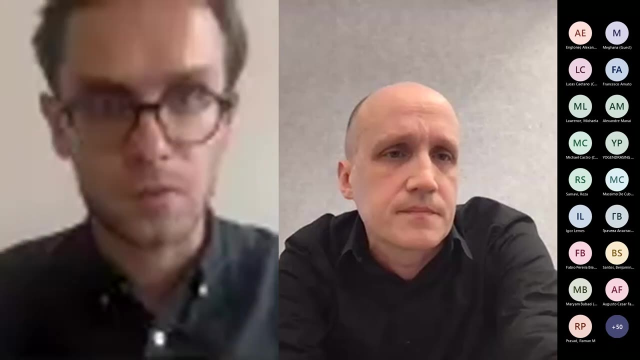 essentially over the last couple of years, a lot of cloud providers have realized that they could also offer similar uh properties um, so they could guarantee the code that's being run within enclaves and separate it from the rest of the environment, such that even the host um of the of the enclaves. 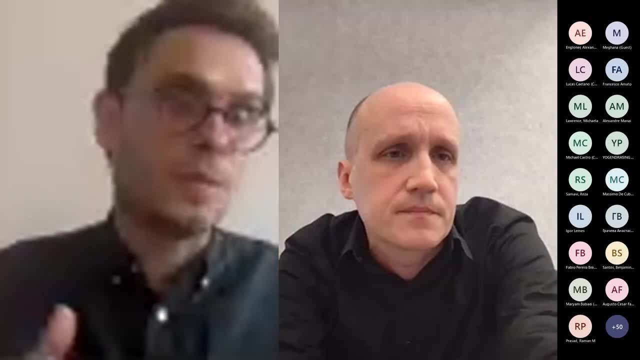 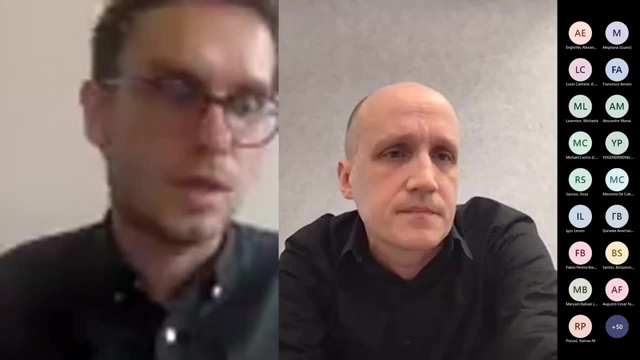 cannot look inside um, and these don't have, for example, limitations in terms of such limitations in terms of memory, like intel sgx, which has, for example, like 128 megabytes of limitation, and so on. so they're, they're both kind of hardware based enclaves and 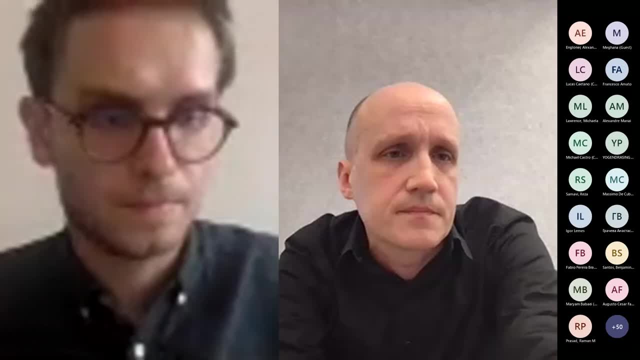 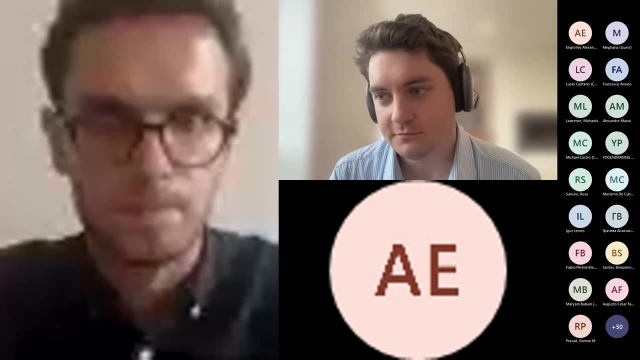 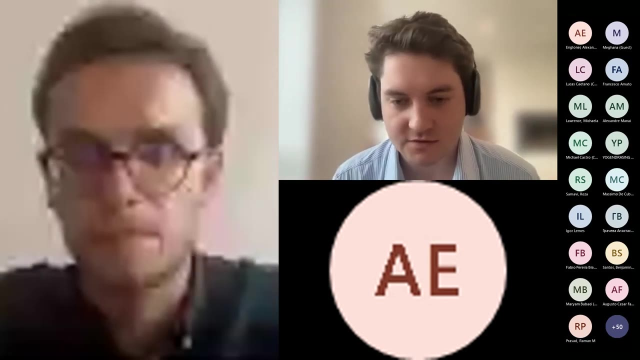 say, hypervisor based enclaves from cloud providers. yeah, great, i think. i think the point in both of those contexts is that um, like 90 of it seems to seems to be people using their cloud or managing their own um data centers and buying physical infrastructure. i don't, although if you have an iphone, there's actually an enclave. 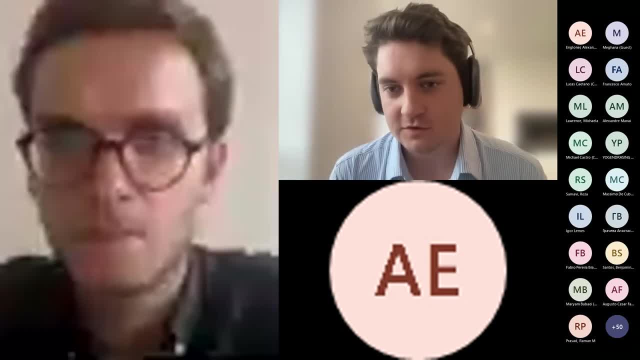 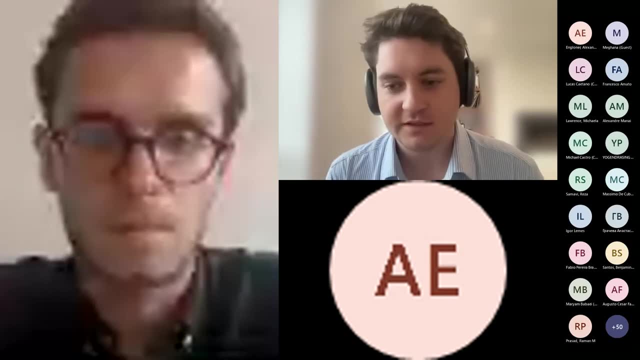 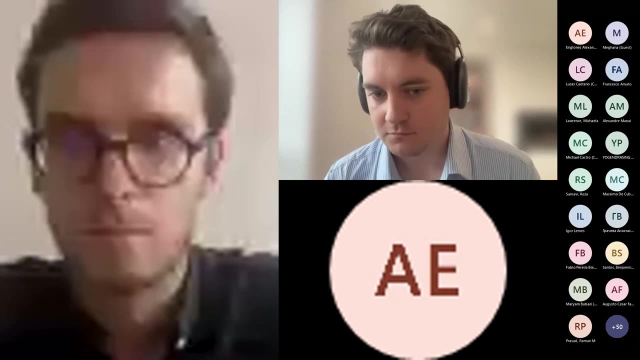 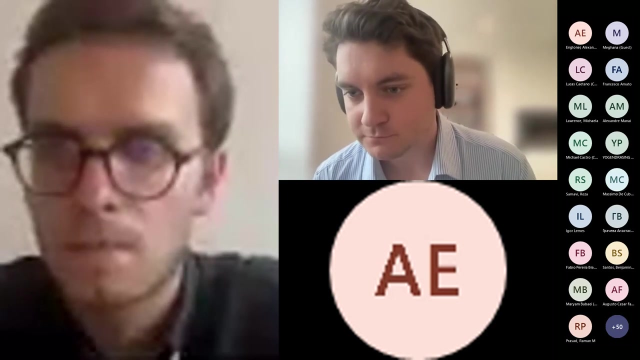 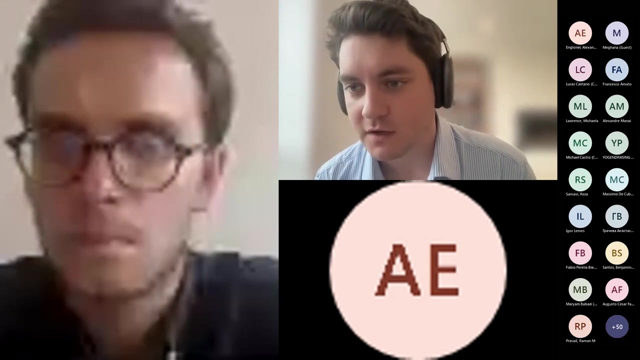 but that does work and james are. do you think we're good to go at this point? i believe he is okay, i believe he's frozen, so, um, let's, i'll scroll up um another question from oleg and said: rob, if we have to trust the owner of the hardware- and i need the enclave anyway- why don't we trust? 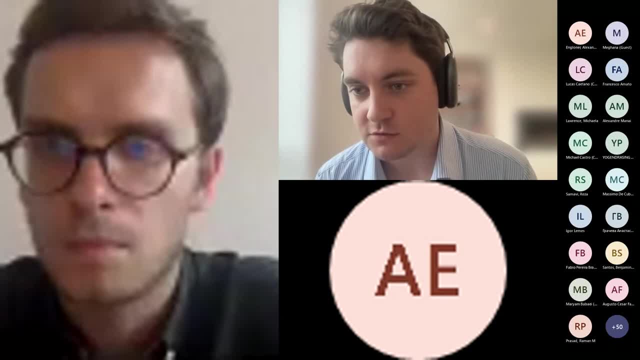 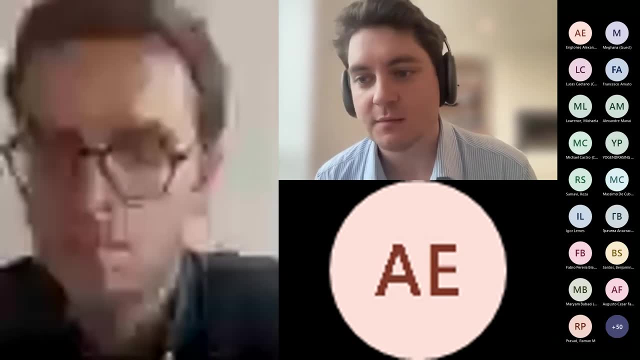 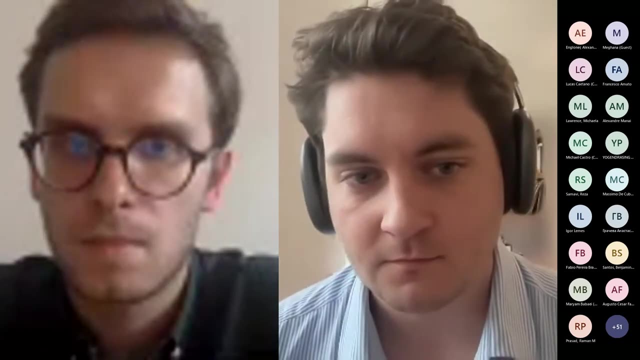 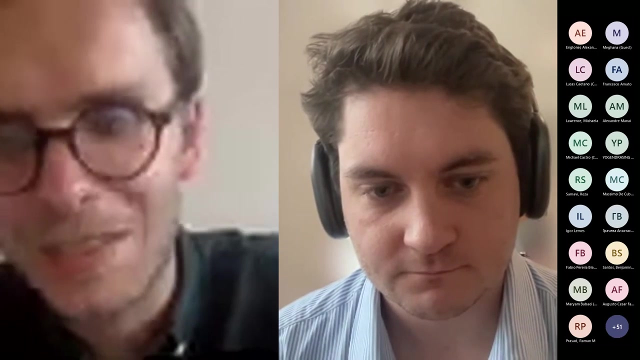 like a key management service, a kms hardware to manage keys and provide protections from hosting providers, eg aws. at the same way, would kms amount to sufficient supplementary measures for transfer to the us, etc. um, yeah, when it comes to the um, the kind of the, but this is sufficient supplementary measure for transfer, uh. 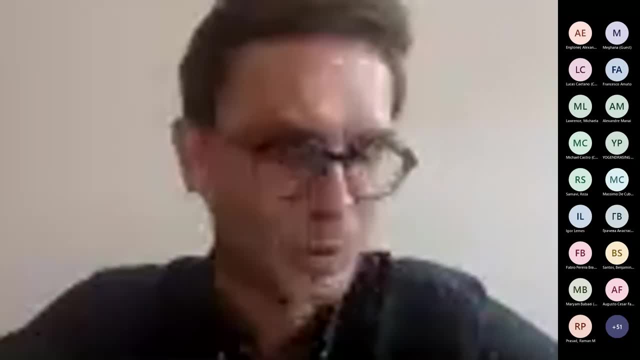 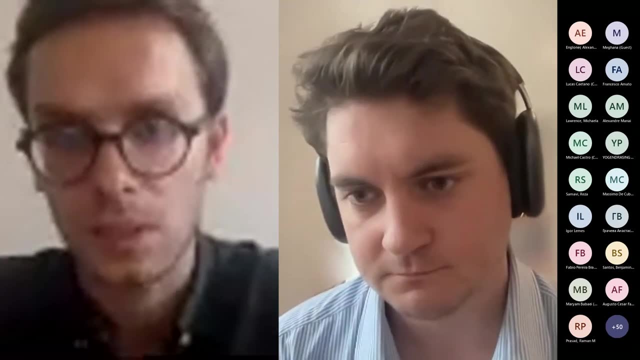 i cannot really comment on that. uh, it's really kind of the question to the lawyers and, of course, part of the whole discussion around: uh, shrems too and um and sending, for example, data between the eu and the us- um, so i don't think there is any definite answer when it comes to that. 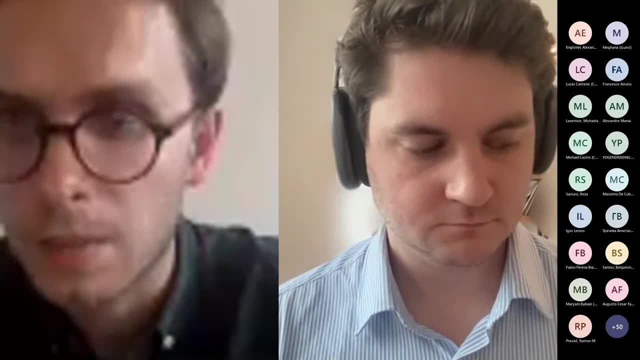 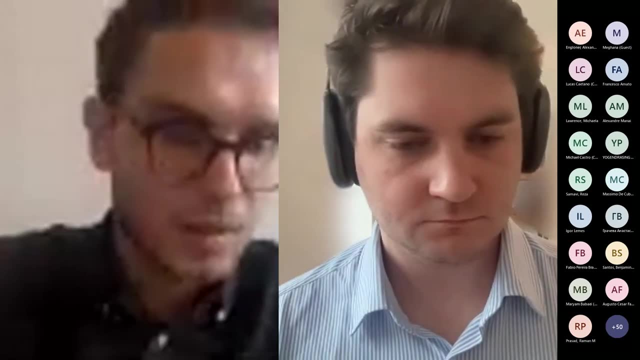 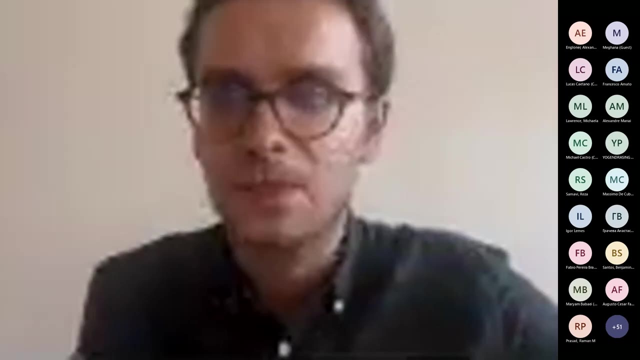 um. however, when it comes to the um key management and, uh, um, that and kind of the hardware based enclaves, really that that's almost like exactly what you're saying when it comes to, like, what the clouds have realized, right, so what you can do is that you can essentially now trust the cloud, um, and ultimately, 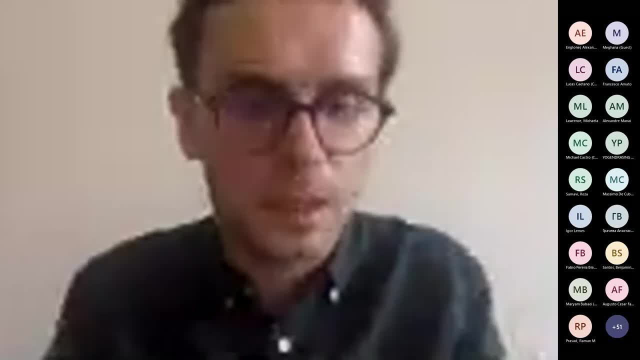 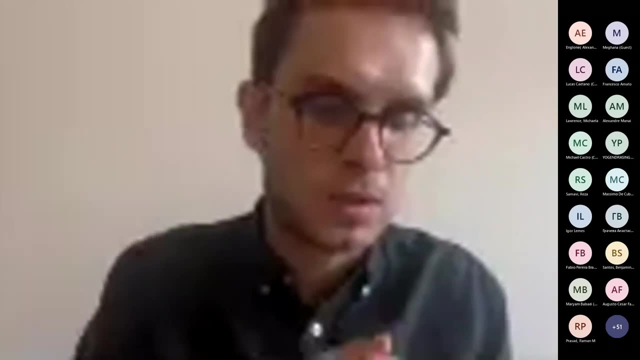 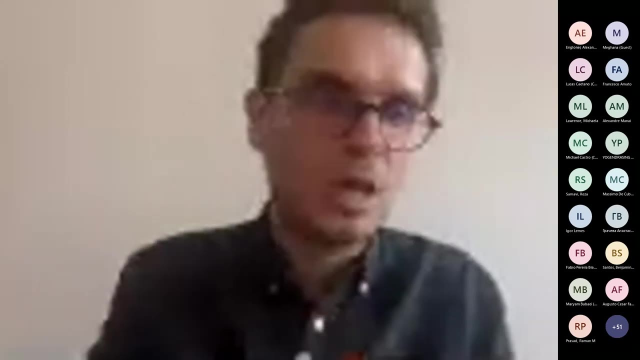 for example, you know case of aws, aws certificate authority, or, in the case you know of other clouds, their respective key management services and and certificate authorities. um, when it comes to the um, you know the guarantees about what's being run inside, so you can have kind of the 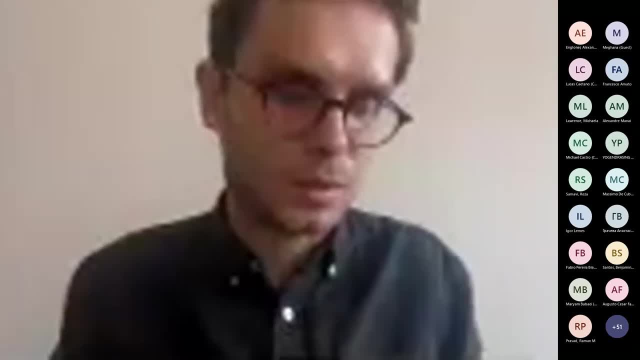 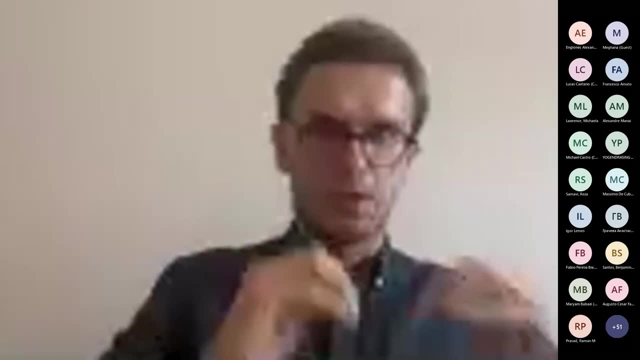 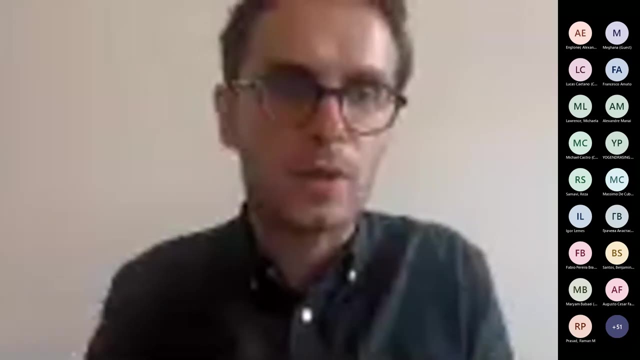 hardware, uh, guarantees, if you, if you're more concerned about, um, you know you don't trust the cloud, for example, and you really want to make sure that, um, that it's actually, you know, the producer of the chips that provides these guarantees, together with through the attestation mechanism with, for example, the cloud provider. 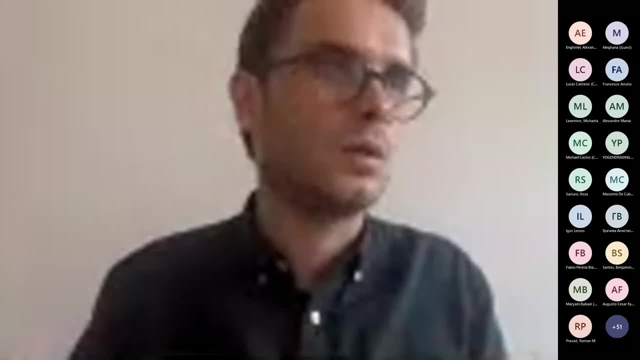 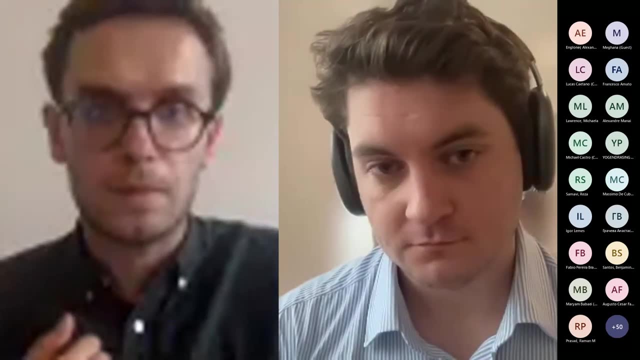 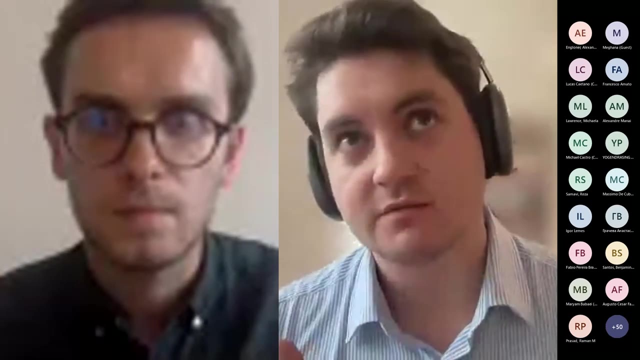 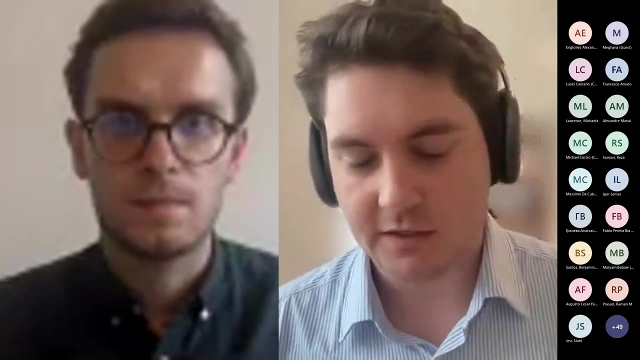 but neither of the parties solely can can be all of that information, um, or you decide: okay, i just trust the cloud provider. yeah, so maybe as well. just to clarify so the like a kms key management service on aws, for example. you typically store keys- symmetric or asymmetric keys- and then you have either people or servers. 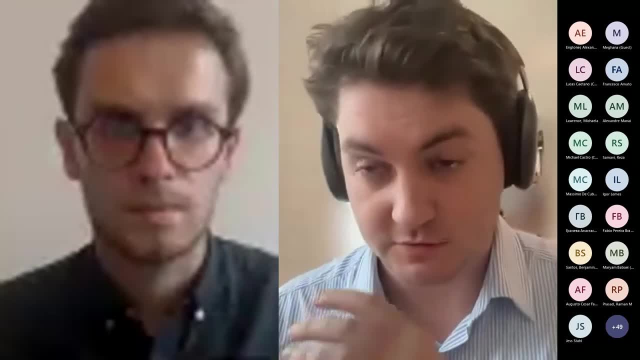 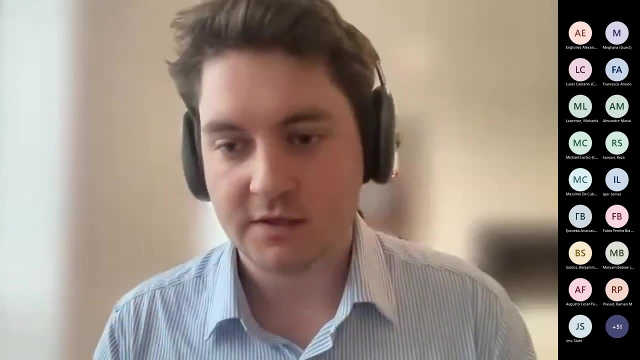 or armies etc. that have access to receive them to encrypt or decrypt some data. so the inclusion of enclaves is kind of a step forward. so it's like the ec2 server itself running specific pre-approved code and the handshake that it does to the kms. 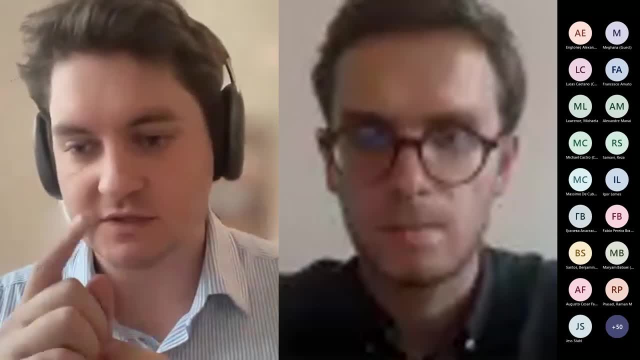 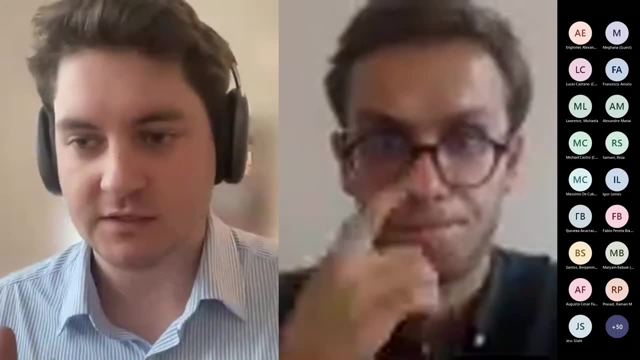 um gives it access to a key so you can, instead of saying this server or this person has access, you can actually say, uh, isolated environment that's running this specific image is is the only thing that has access to maybe decrypt a particular amount of data. so they're often used. 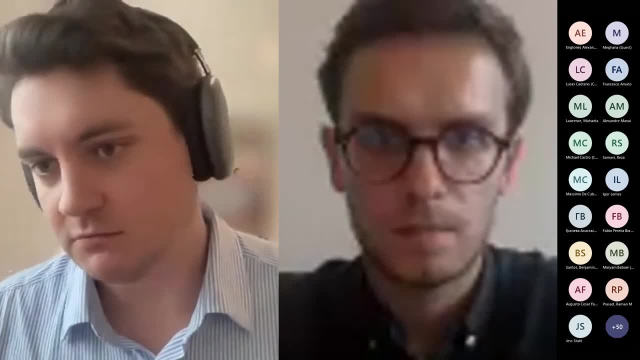 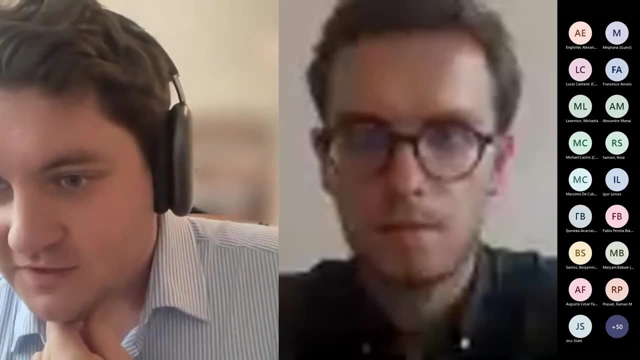 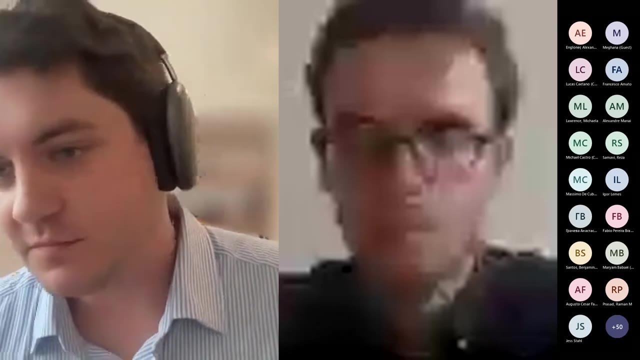 in conjunction with one another, um, as a, you know, as opposed to separate, and okay, great, so maybe as well field another question for the time being. so, cp, i said as to the regards to te enclaves. by the way, these are all concrete questions. it's just because they were the most recent. 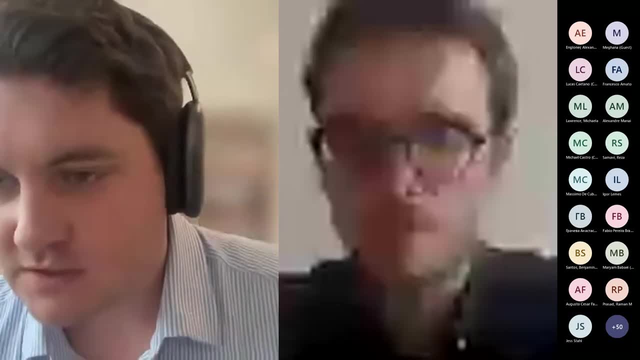 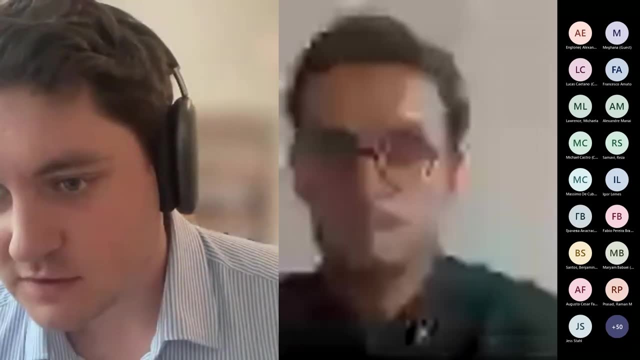 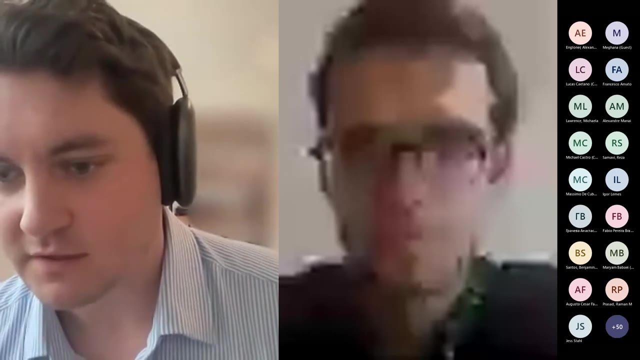 ones while rob was still on here. and as to regards uh, to just execution environment enclaves, and it is specialist hardware that comes in with the current uh in in some intel servers. uh, basically, when the server was: oh, this is an explanation. okay, that's not a question, that's totally fine. so, um, i can roll up. 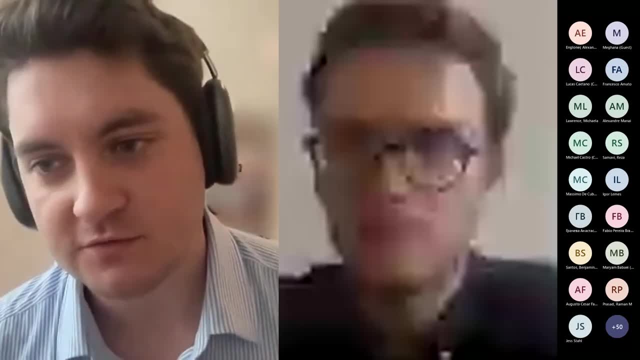 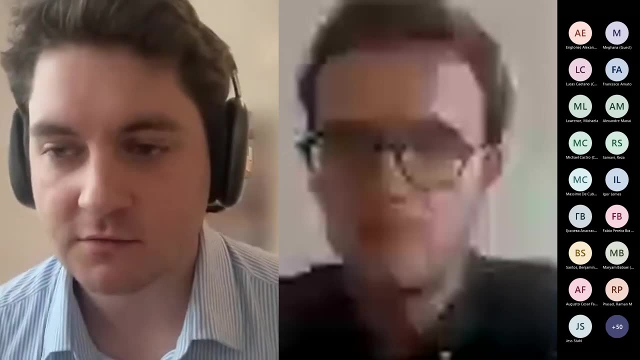 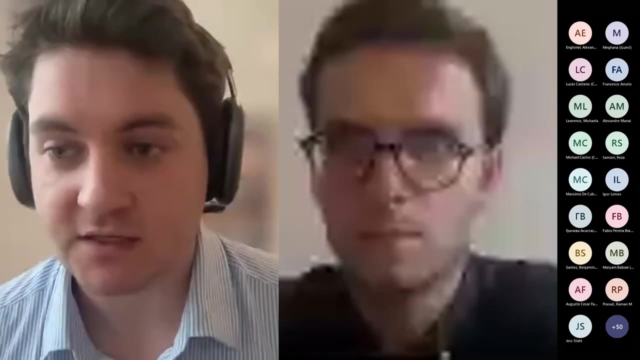 okay, so there was a question from matthew bush- i believe this would have been to federico um- saying: are there any other privacy risks other than re-identification for unhcr? so i think there's a lot of risk to whole groups of people. uh, as well, depending on information that. 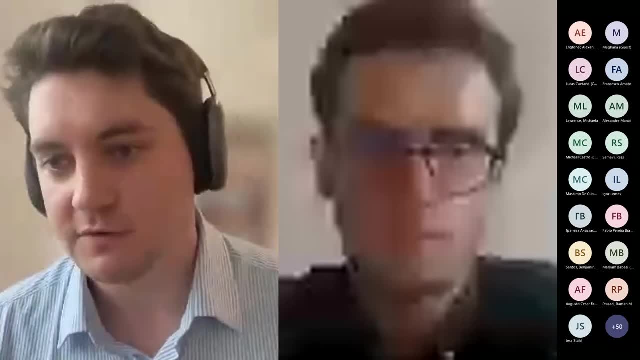 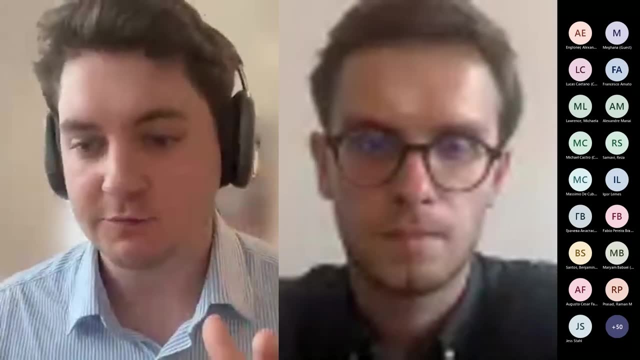 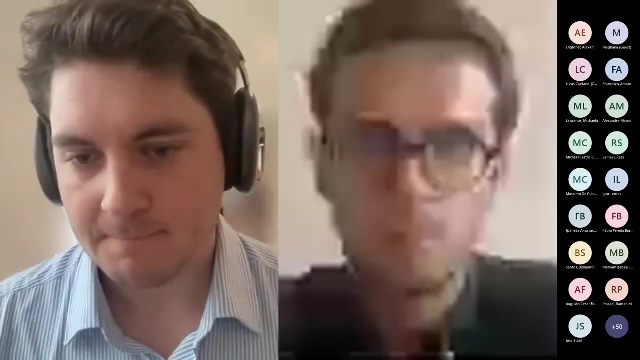 gets disclosed. so i can imagine there'll be different subgroups within refugees or something which potentially um might be very sensitive characteristics as an entire group as opposed to just at an individual level, and do you have any comments on that? uh, federico, yes, absolutely. uh, there is also this kind of disclosure that is possible to happen. 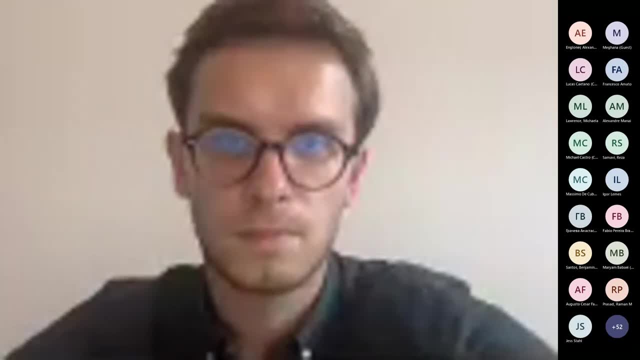 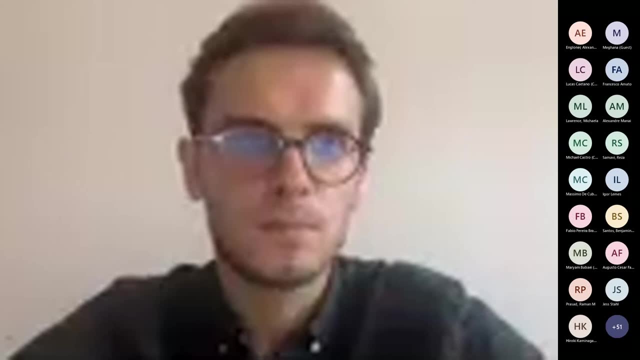 and for example, just to give an example, you could have like a subset of or people that even if you cannot disclose the individuals, you can still say that people belonging to this group have these particular characteristics. so for example, just to give a practical example, you could tell in some circumstances that in one camper refugee camp, most 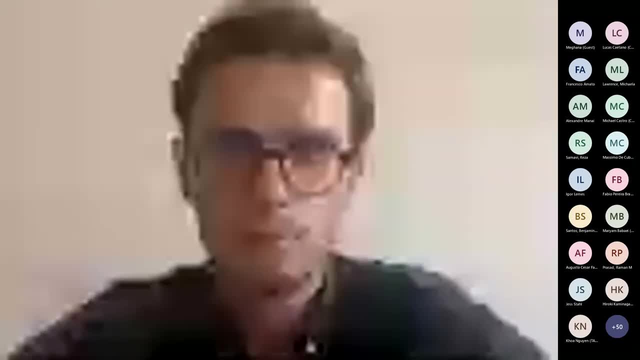 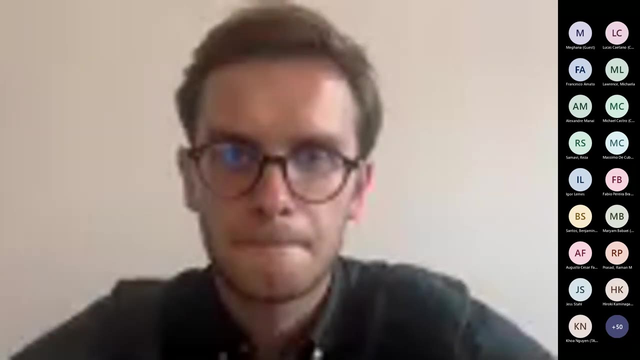 or all of them belong to a particular minority. so in this case, even if you cannot disclose the individuals, you can still disclose some characteristic individuals. they are in that camp. so we do check this as well in the data checking what is sensitive, particular sensitive, and also we use a sensitivity that was 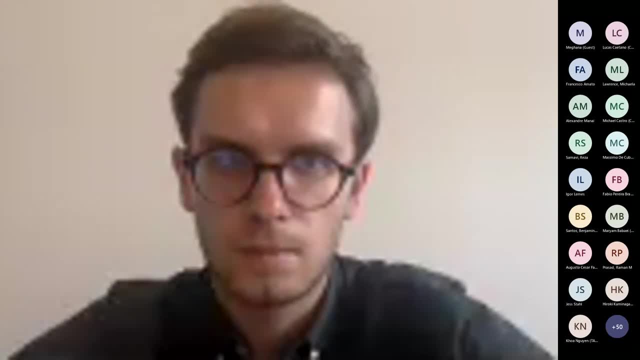 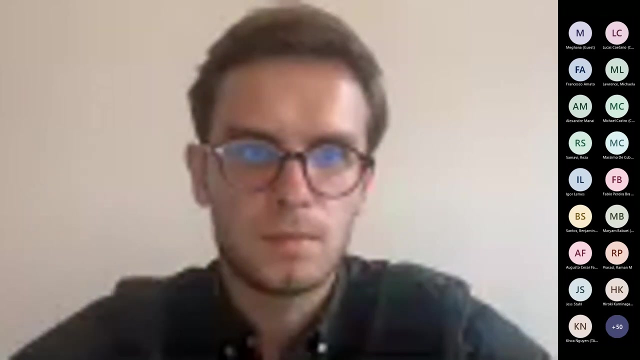 another question, um, to see what are the numbers of the diversity in each camp or for some sensitive variable, but to answer also to answer to oleg plino, since it was related. we don't have a standard value for lbu because also depends on the values that can the sensitivity. 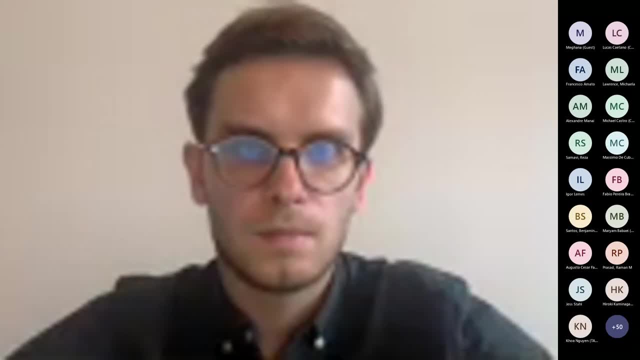 variable assume. so there is some institutional descriptionality in the decision making is also why differential privacy could be more scalable. it just to answer quickly to oleg as well. they asked the community level that we apply. typically we apply key rebuild of level 3. we decide this level looking at literature. 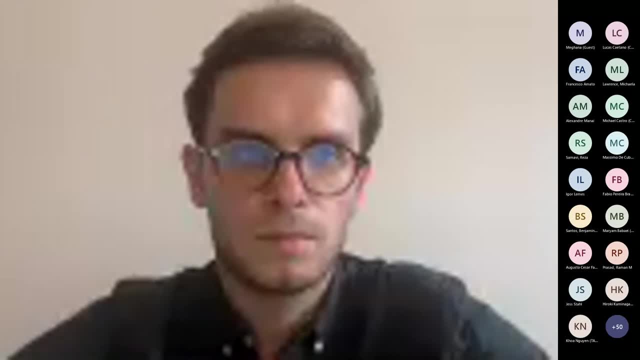 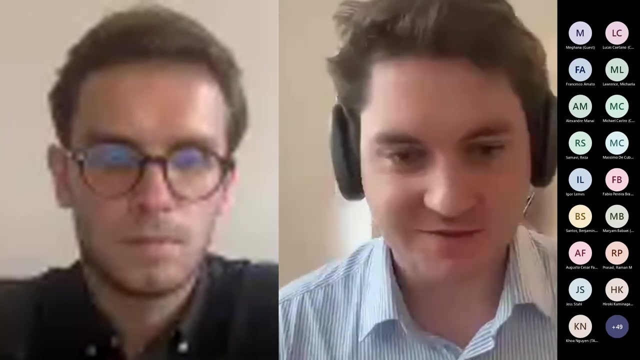 doing some tests, also discussing with other organizations the use, the same methods, and we came up with this, uh, this standard over great well, thanks. thank you so much for clarifying that, federico. so i think, uh, james is back and i now have the slides on this side, so i'll share screen um and hopefully screen up and hopefully. 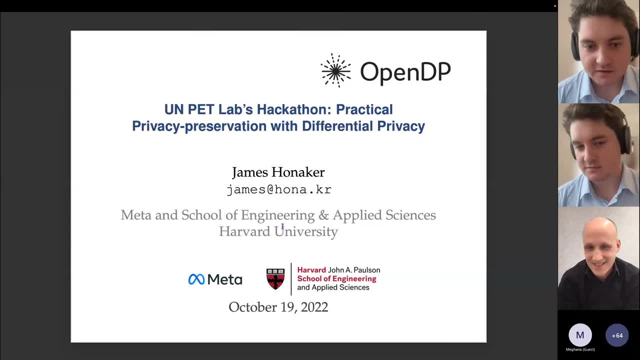 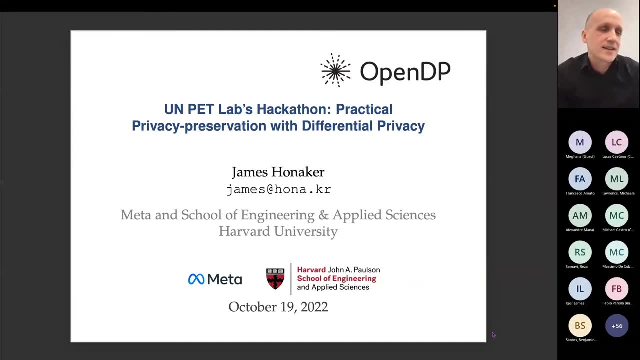 we can go from there. can everyone see that this slides lovely? um. so, yeah, uh, thank you for this opportunity. it's, uh, it was, uh, it's. it's very rare that i, that i get to be in the uh situation of um, um, having such such a nice foundation set up by the other speakers, um, so you'll see that in these. 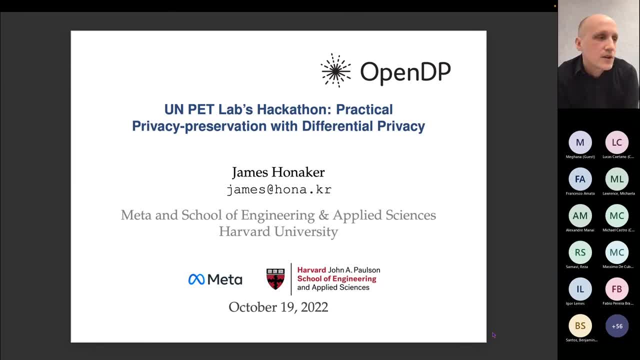 particular slides. uh, there's a quick review of some of these, these, these things we've already talked about and, uh, and we can scroll through the slides and see if there's anything else that you want to skip through those. um, uh, my name is james. uh, uh, i'm a research scientist at meta. i work. 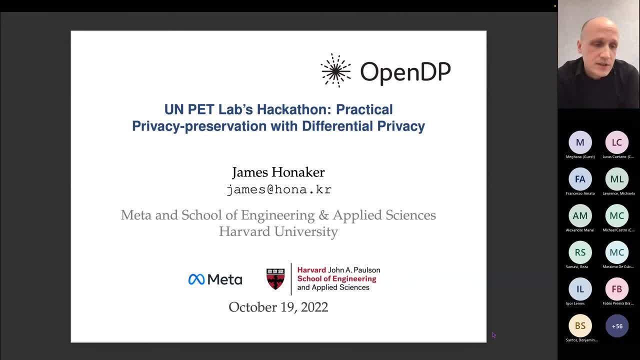 primarily on differential privacy. but hearkening back to the oblivious talk um differential privacy: in and of itself it gives you output privacy, but you, if you, want an end-to-end private solution, often what's really interesting and and what's sort of at the forefront of innovative research. 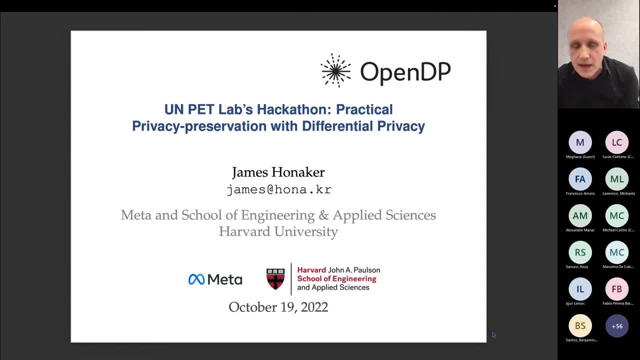 is ways to combine differential privacy with other privacy, enhancing techniques, um so ways of privacy, uh, you know, uh, protecting privacy over the computation itself, and so combining differential privacy as an output layer with multi-party computation, with enclaves, as talked about, with homomorphic encryption- um is is really exciting in in building real systems and uh. 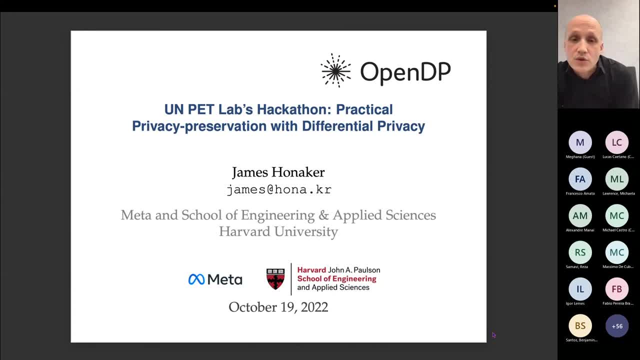 and it's it's. it'll be exciting to see what kinds of uh solutions people come up with uh in in this hackathon. it's, it's a. it's really interesting um proposal to be to be playing with um in the live in this, in this project. okay, um, let's see what the next slide is. 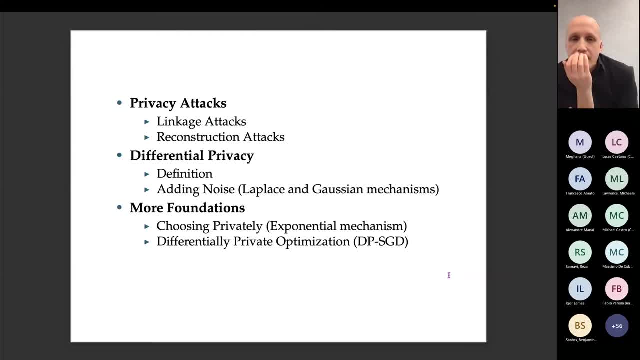 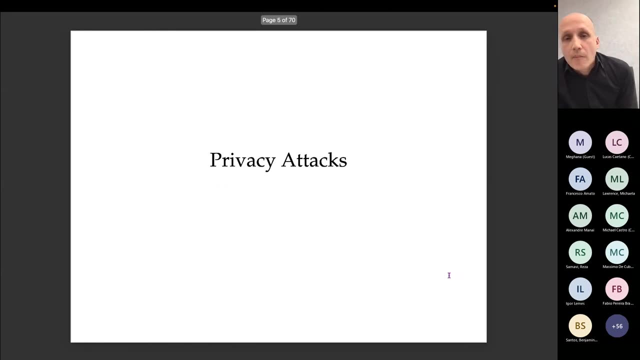 ah, okay. so, uh, we've talked a lot about uh already, uh, in the first talk about um, uh, the different types of linkage attacks and reconstruction attacks that are that are that are possible in the world. if we skip to say like slide 21, 22, um way down there, um, i'll just say uh, 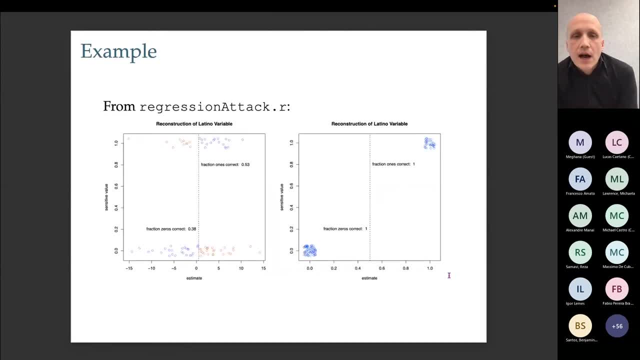 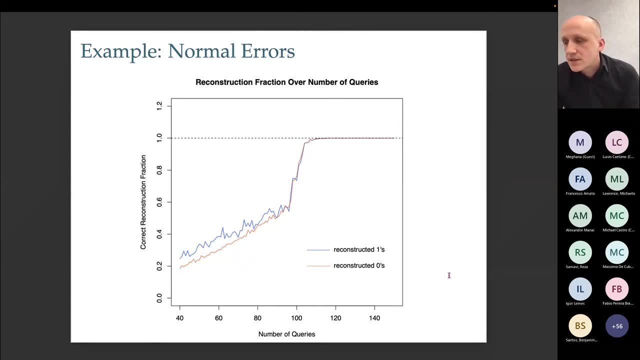 here's a bunch of attacks. they've been, they've been. next one, please. um, the, the, the fundamental sort of thing that we're pressing up against here, uh, this, this, this sort of information, theoretic, uh result by dean or nissim, that that sort of launches a lot of the, the pets world, uh. 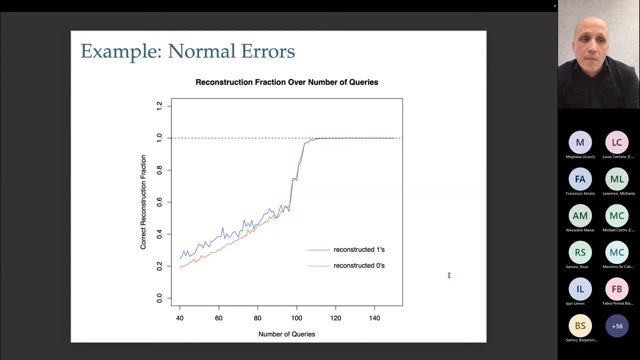 you know, 20 years ago perhaps- is this idea that, um, if you start releasing information and you release too many query answers on a data set, or with too much uh, or with too much precision, you will eventually leak the underlying data. there will be a way to. 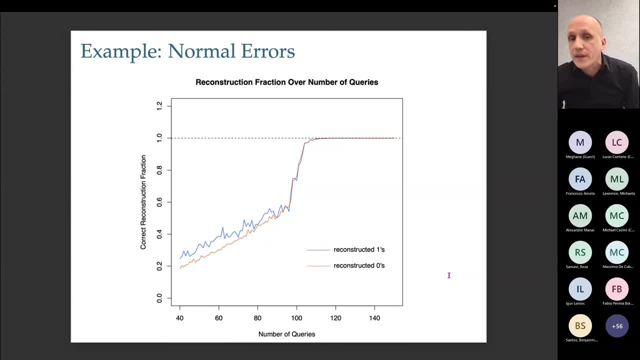 reconstruct from the answers that you've you've released what the underlying data is, and sometimes that's really interesting. you know really simple sort of linkage attacks to auxiliary information. sometimes it's the fact that every time you release information you're learning a little bit more about the underlying data and eventually there's only one underlying data set that could. 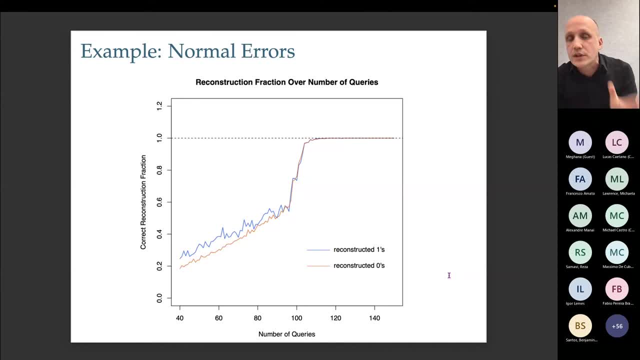 have given you all those possible answers, and so what we see is that, as you start releasing more and more answers, we can. we can in, in increasingly sophisticated ways, start to reconstruct what the underlying data must have been to give you those answers- okay, unless you steeply limit how many. 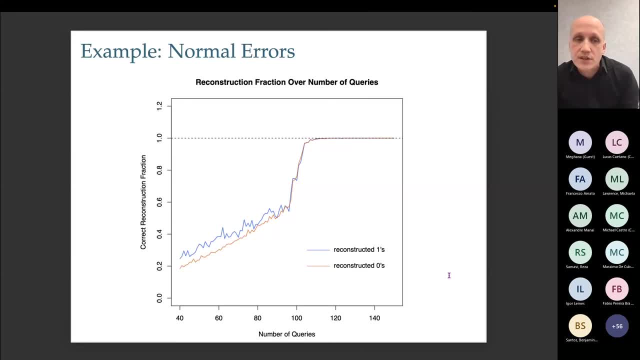 queries you can allow on the data set and then just end things okay, which is unsatisfying, or we add sufficient noise, um to uh, to provide privacy, and that's that's what differential privacy is going to allow. it's going to allow us to, i would say, still learn the underlying truths of the data set, which is what we want, we often want. 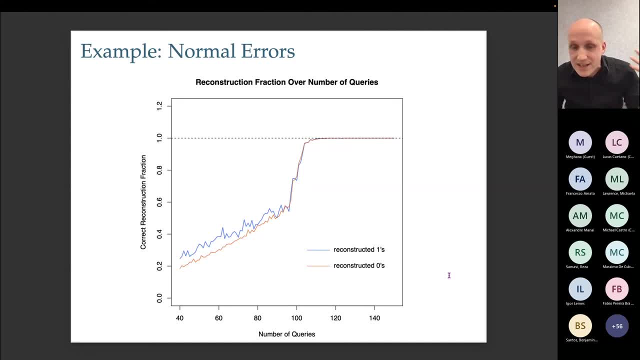 generalized knowledge. we want scientific truths about the, the statistical truths about the broad population, but not learn anything about individuals. it's a way of, if you will, of politely, a polite line um in in my original work. you know my background is in statistics and and originally in statistics i studied a lot of missing data and measurement error problems and, if you will, 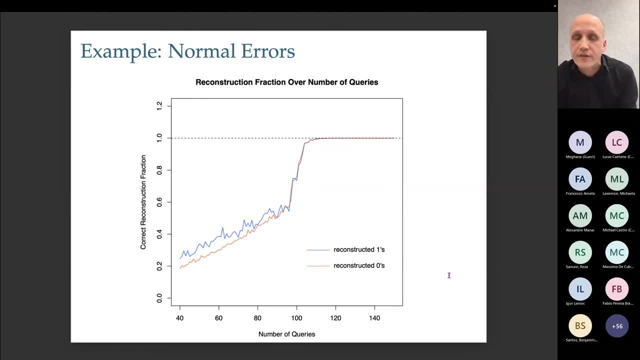 this is a way of Tower. the data set is an intentional, very, very small form of measurement error, and we know how to correct for these things, and the measurement error is going to allow us politely to lie to the, the data analyst, in such a way that we can protect, protect privacy, um, so uh. 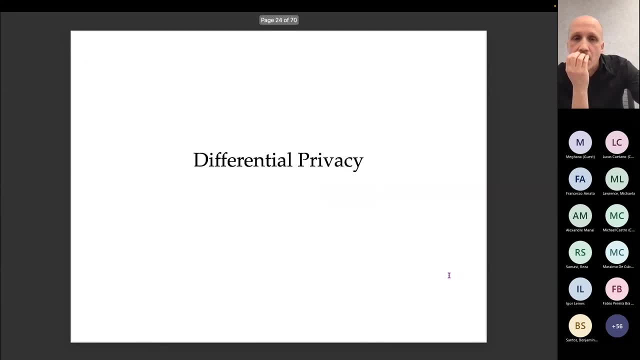 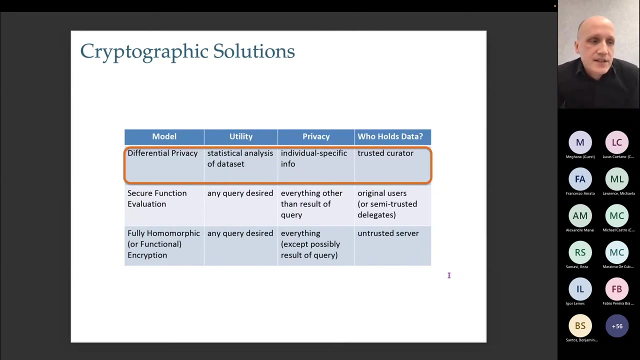 let's skip. uh, perhaps. uh, next slide: differential privacy: perfect, uh, one more um and one more. So we've seen that differential privacy is not in and of itself an end-to-end solution in a system. It's one particular layer, and it's often the case that you want clever combinations with other privacy-enhancing techniques. 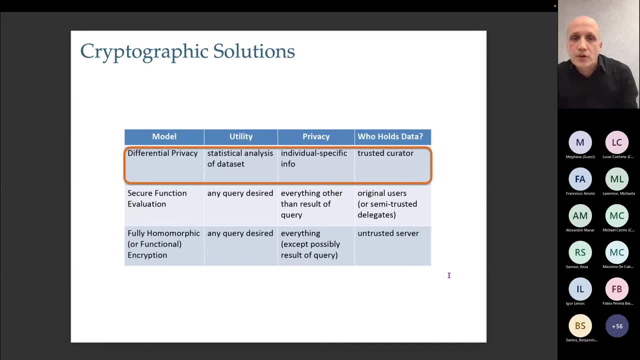 But it is the output layer of many systems. It's the way that the actual answers, when they get out into the world at large, can be guaranteed to still protect the confidentiality of the data that generated those answers. Okay, so next slide. 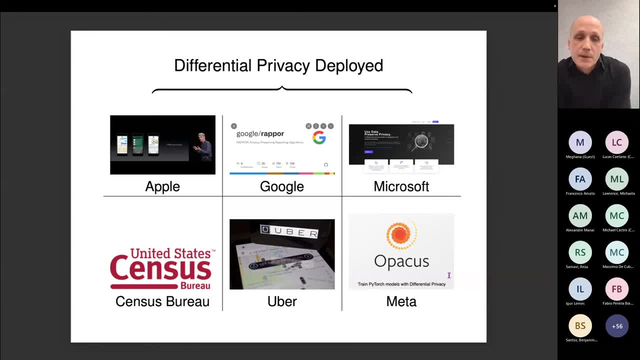 Okay and we've seen, as this literature has been maturing, that we have real large-scale deployments by large tech groups. you know Apple, Google, Microsoft, all building systems for users. Opakis here at Meta, very impressive work to move the US Census Bureau to differential privacy. 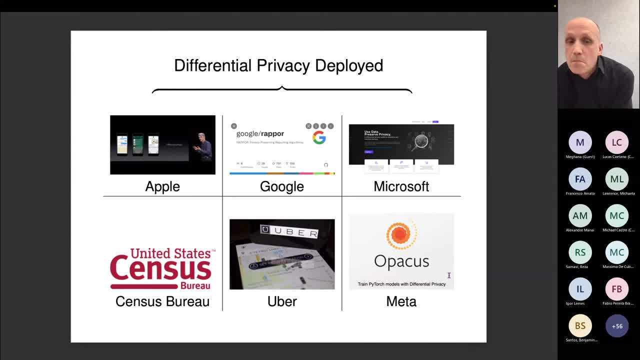 for a few years. For exactly these reasons that the US Census Bureau releases literally millions upon millions of summaries to the data set, and they proved that it was possible, from all that information, to reconstruct the underlying data, and so differential privacy was necessary. 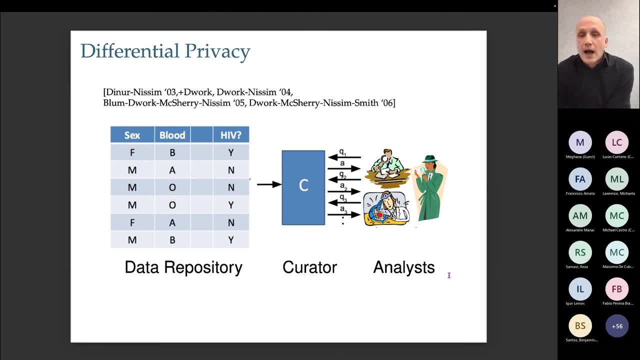 Okay, so next slide. So what do we mean by differential privacy? We'll try to do this a little bit rapid fire here. So let's say there is an underlying data set Here. it's a bunch of individuals and we know their gender, their blood type and say also a particularly sensitive 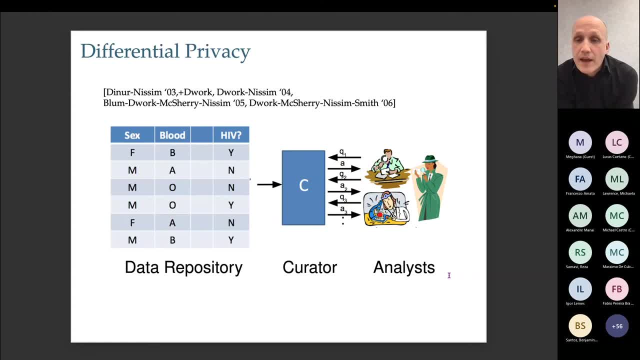 at-risk person. So let's say they have a certain attribute, like what is their disease status, and we have a bunch of analysts who look, you know, like cartoon characters here, but very benevolent souls who are trying to learn fundamental truths for social good, making queries of this data set. and so they ask queries of the data set and they get back answers and the work that's cited on the top line here the Dean Ernissim says: well, if they ask too many questions, some more malicious soul- let's say, go to the next slide- would be able to take all of the answers from the data set and then get back answers. 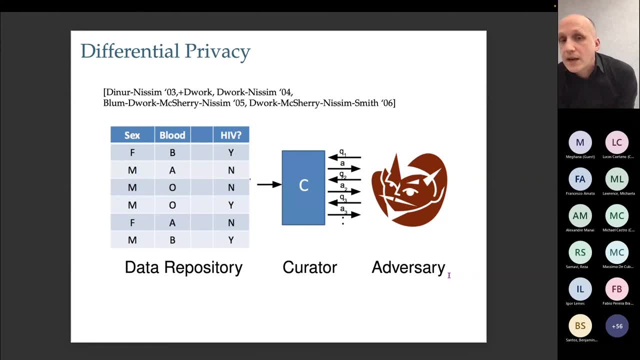 Okay, so next slide. So let's say they have a particular attribute, like what is their gender, their blood type, and say also a particularly sensitive soul- let's say go to the next slide- would be able to take all of the answers from the data set and then get back answers. 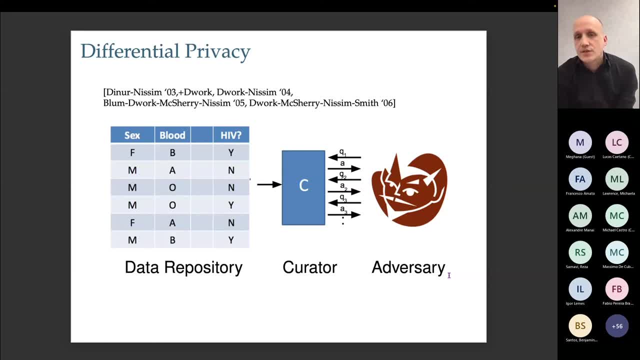